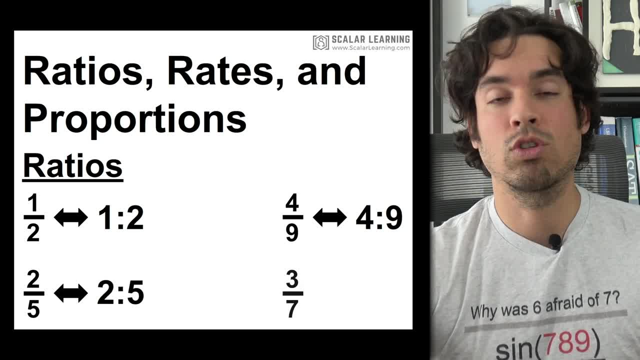 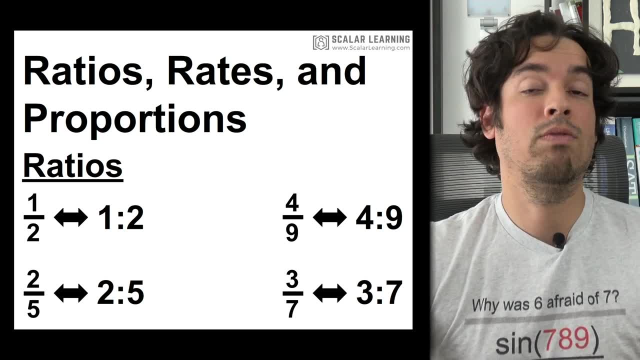 five or two fifths is like a two to five ratio and, of course, three sevenths is like a three to seven ratio. So a lot of times too, when they're asking you, hey, you need to find the ratio of a to b, A great way to do that is actually put it in fractional form of a over b when you're trying to 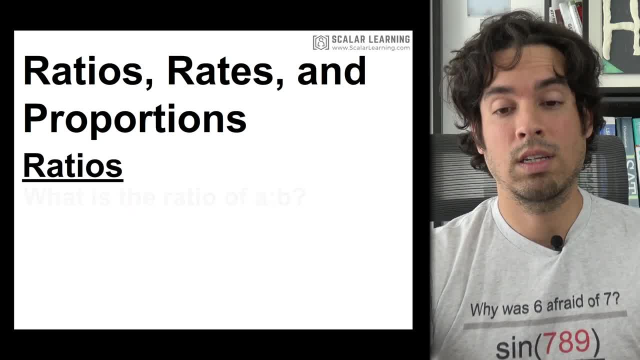 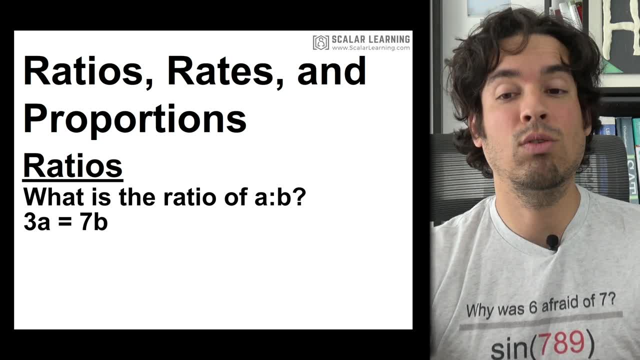 isolate that particular ratio. So now we're going to walk through a quick example where they say: hey, what is the ratio of a to b? So, for example, we start with an equation and we've got three a equals seven b. Now I know a lot of you want to immediately jump to say: well, 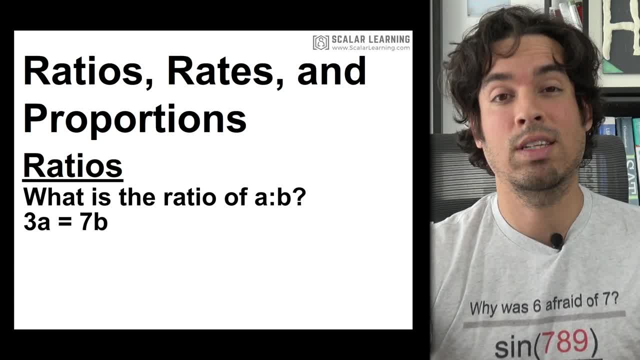 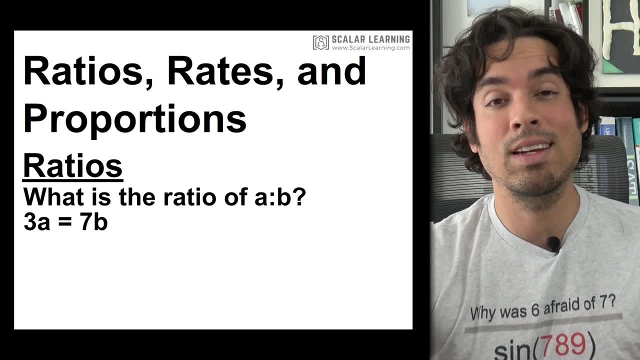 if they're asking for the ratio and it right now says three a equals seven b, the ratio is three to seven. You can't go that quickly. First you got to think: all right, well, if I want the ratio of a to b again, I want to put it in fractional form of a over b. So what we do is we divide both sides by. 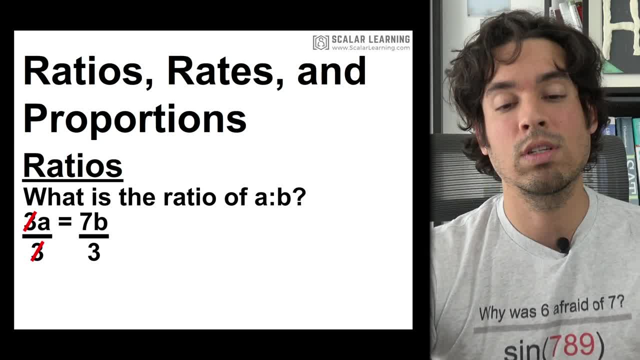 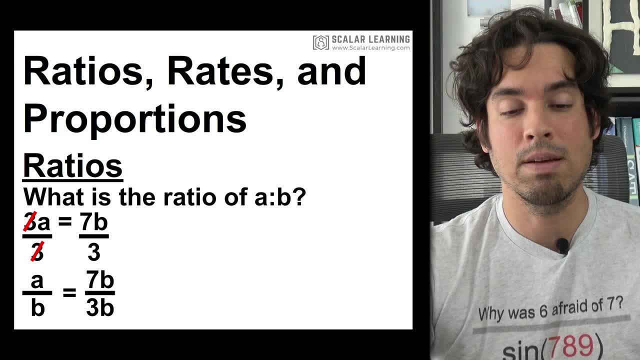 three. right, We cancel out those threes. Now we have a equals seven, b over three. Okay, in the next step we want to get a over b. So now we're going to divide both sides by b and again canceling out the b's on the right side, And now we've got a. 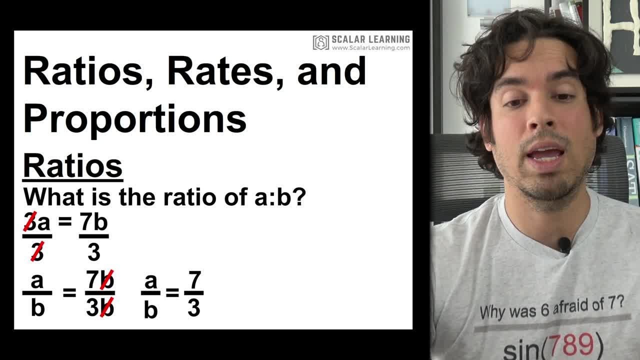 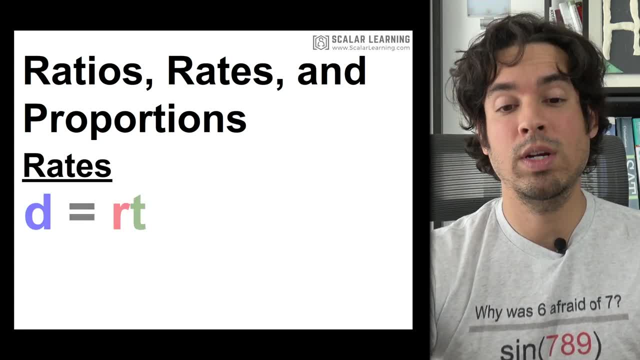 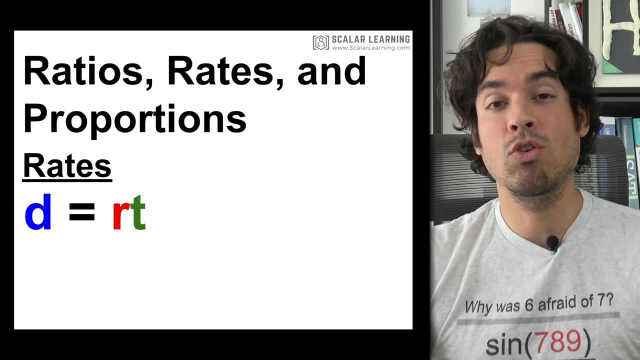 over b is seven thirds, which means that my ratio of a to b is simply seven to three. Next, let's talk about rates. So what are rates? Rates are essentially from this equation: distance equals rate times, time, Basically talking about speed. This equation- I know you guys might think it's 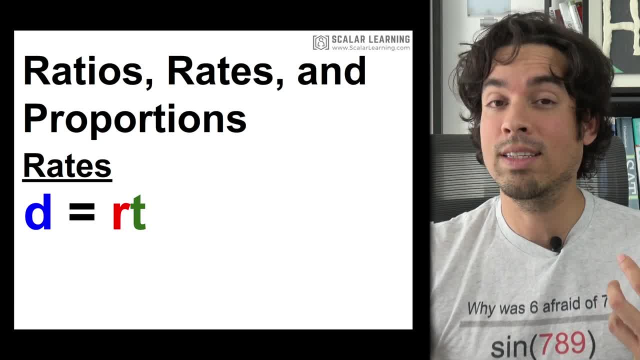 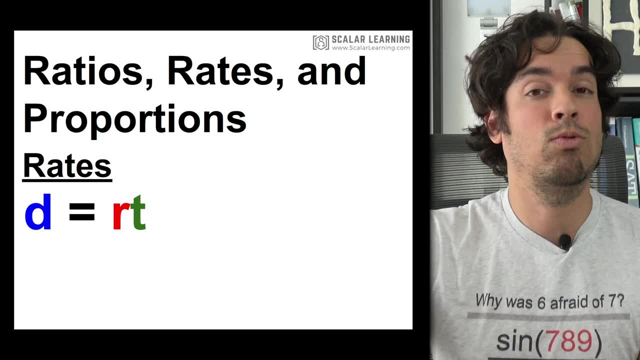 super simple and I don't need to worry about it. but it's such an amazing tool- at least I find when I'm working through problems- to have this as a backbone. So when I'm when I'm trying to figure out how do I get those, I just plug it into this formula and I don't have to overthink it. So, again, 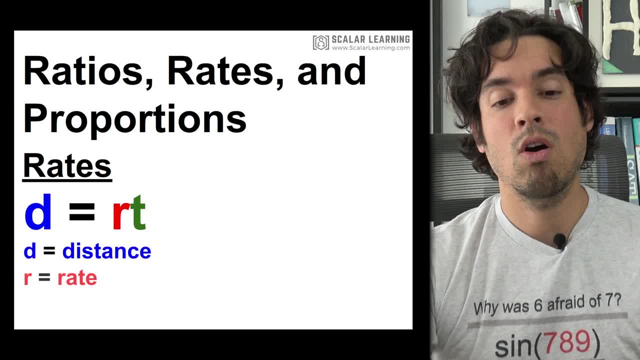 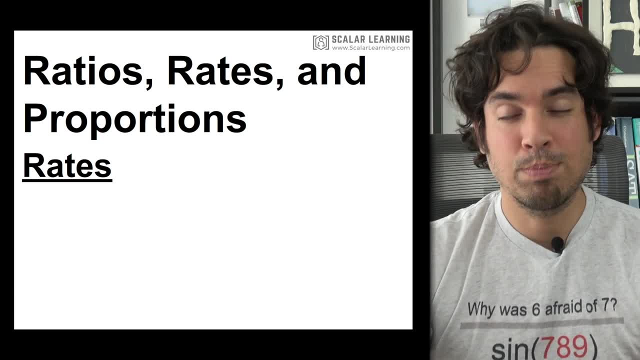 in this formula let's just go through the terms: D equals distance, R equals rate- again, which is synonymous with speed- And, last but not least, t stands for time. Now let's look at a particular example involving rates. So if we look at this problem, it says: Laura can swim two laps in the 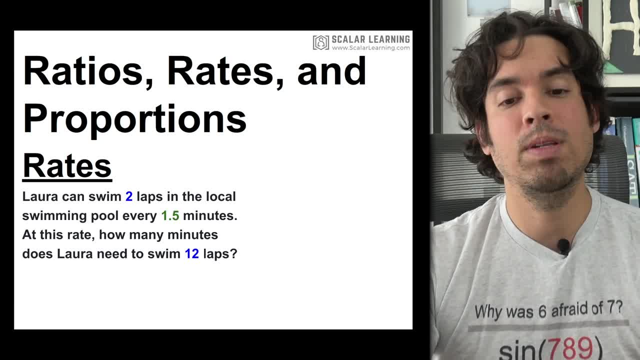 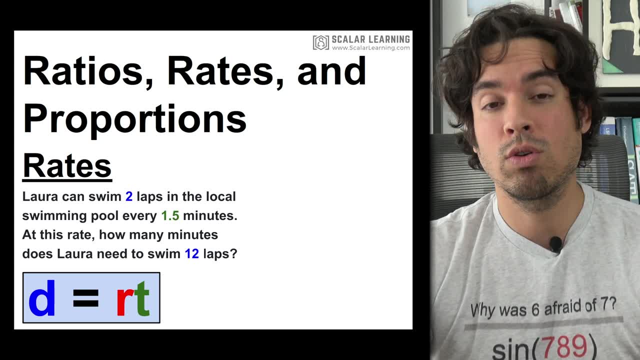 local swimming pool every one point five minutes. At this rate, how many minutes does Laura need to swim in the local swimming pool every one point five minutes? R equals rate times time. Now notice I color coded those numbers right. The numbers in blue correspond to distance and the 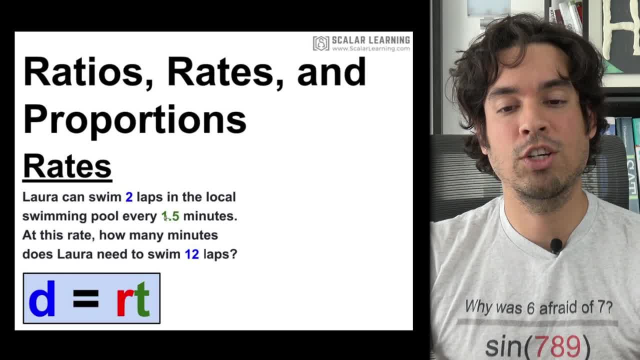 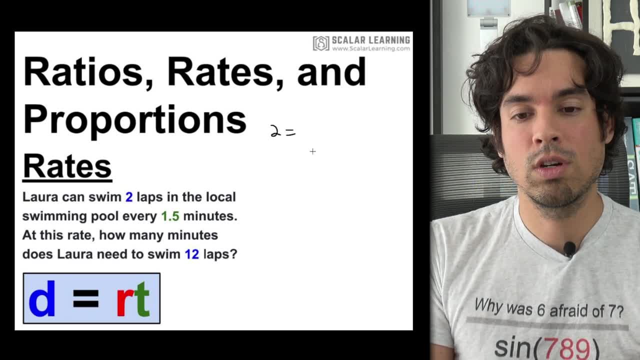 number in green corresponds to time. All right, So now, how do we break it down? So, first of all, with the initial pieces of information, I can actually calculate that rate. So I'm going to go ahead and do that and I'm going to plug that in as follows. It's going to say two equals rate, which. 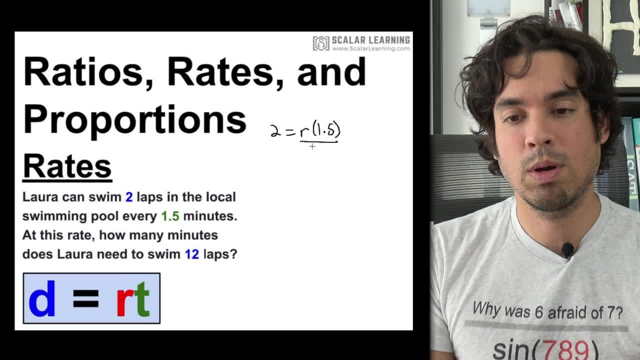 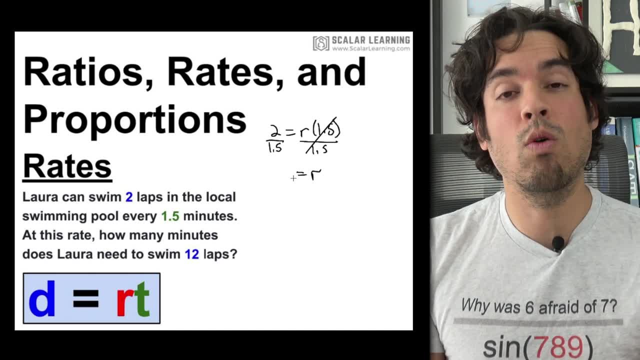 is unknown times, one point five minutes. OK, And then I'm going to isolate R by dividing both sides by one point five. by one point five. And what do I get? I get R equals instead of two. over one point five. I'm going to double it, double. 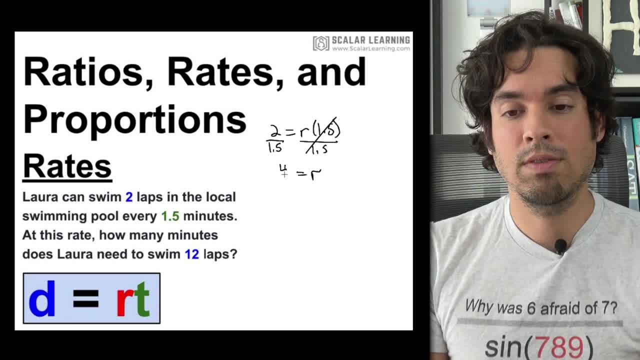 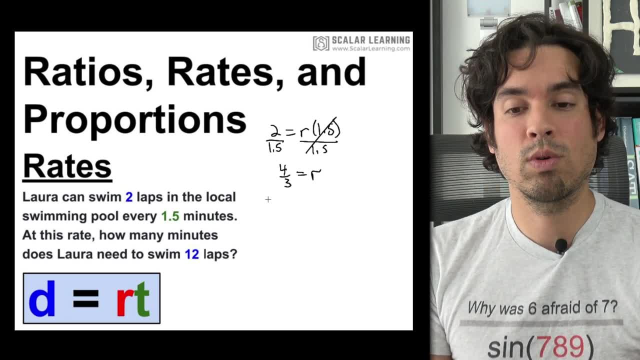 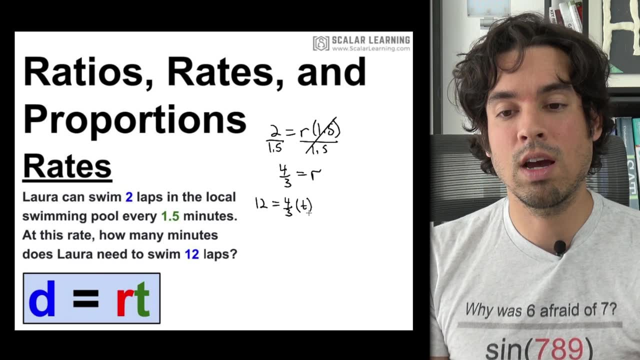 numerator and denominator. so I don't have a decimal in a fraction And I've got a rate of four thirds. All right, Now I can plug this in again with this information: How long does Laura need to swim 12 laps? So now I've got 12 equals a rate of four thirds times an unknown time. OK, Now we can. 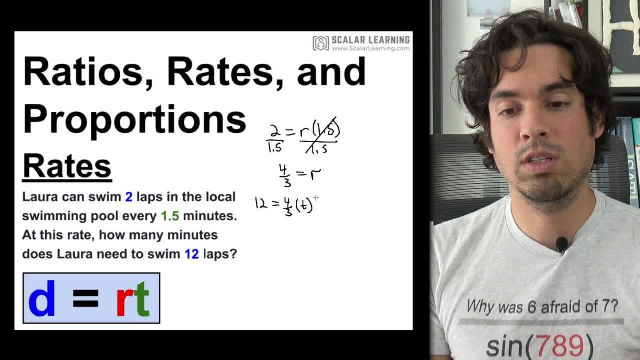 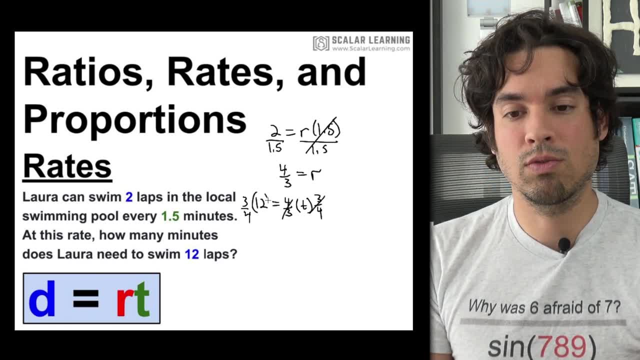 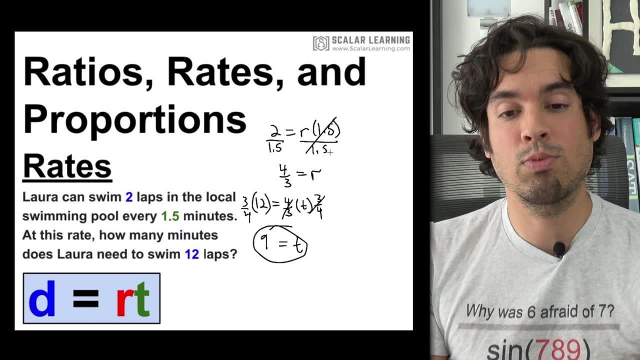 solve this way. So I'm going to isolate by multiplying both sides by the reciprocal of four thirds, which is Three fourths like. so that cancels three fourths of 12 ends up being nine. Now, this isn't the only way, by the by the way, that we can solve this problem. Instead, we could have used a proportion. 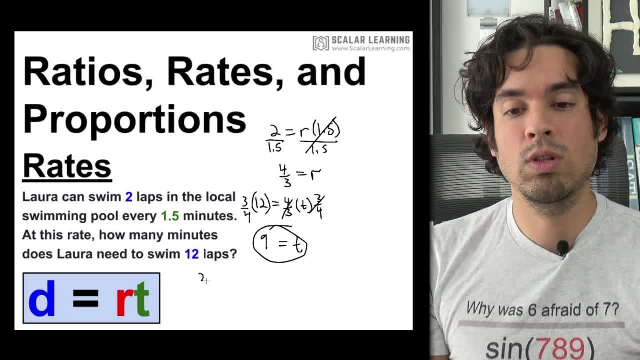 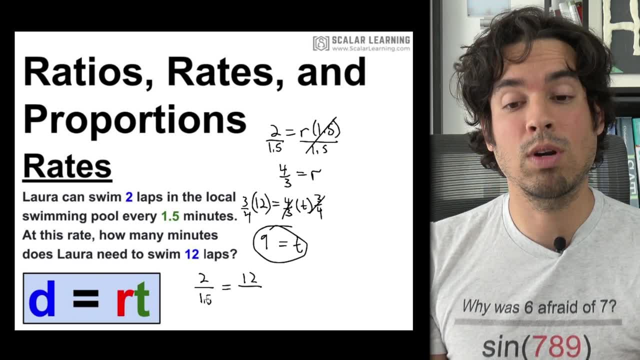 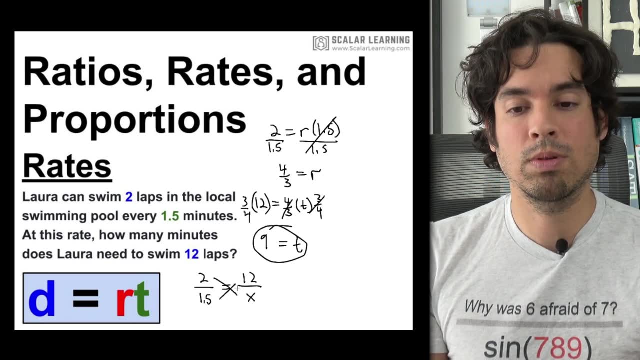 So, for example, I could have said: if we do two laps in one point, five minutes, how long will it take for 12 laps? And again the time goes on the bottom right. We have matching time and matching laps on the top. This is my unknown time and now we can just cross, multiply, right. 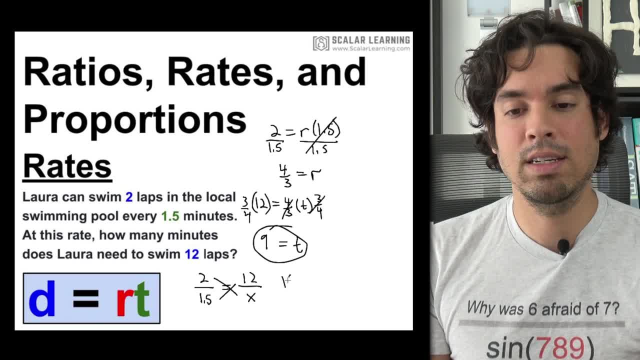 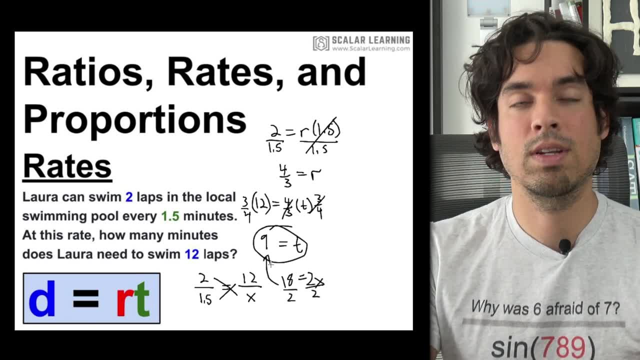 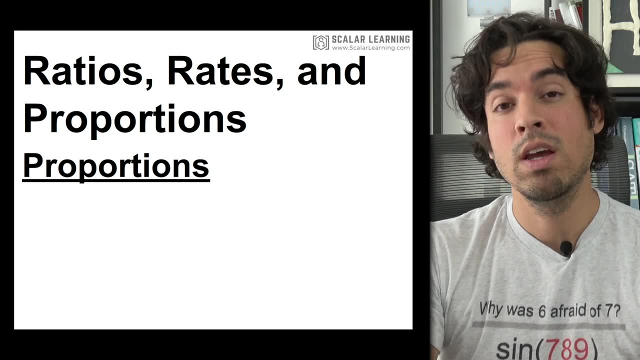 So 12 times one point five ends up being 18 equals two. x dividing by two gets us that exact same answer of nine. Next let's talk about proportion. So proportions are incredibly important on this test And, as you saw in the last example, even though I did solve it using distance equals rate, times, time, initially, proportions came in quite handy. 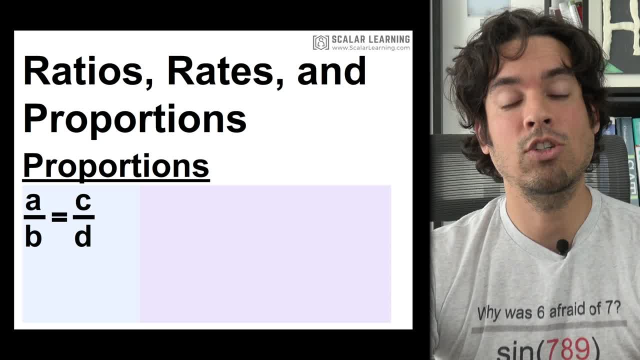 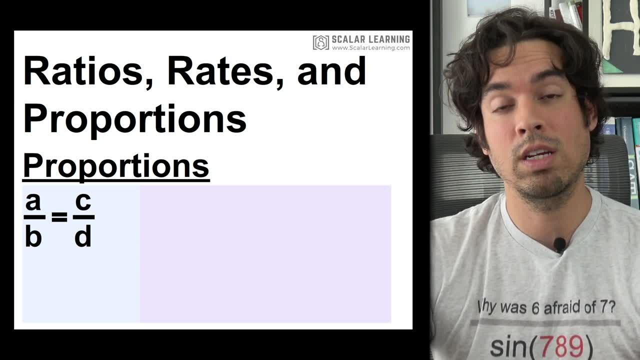 there as well. When we talk about proportions. All right, It's essentially a fraction equals a fraction. That's how you want to think about it, And this is sort of a standard way to look at it. A over B equals C over D. Or, if we're talking ratios, A to B is the same as C to D. 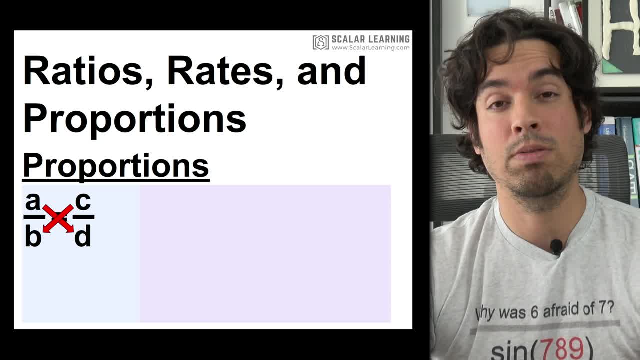 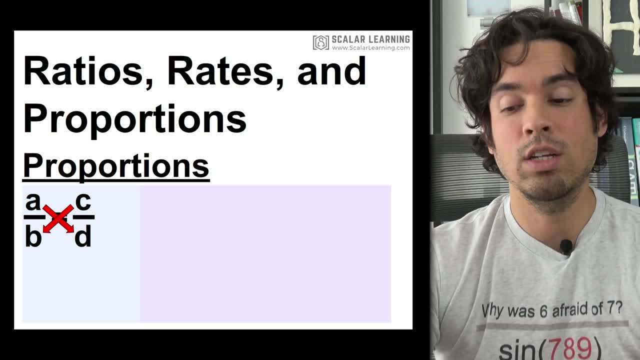 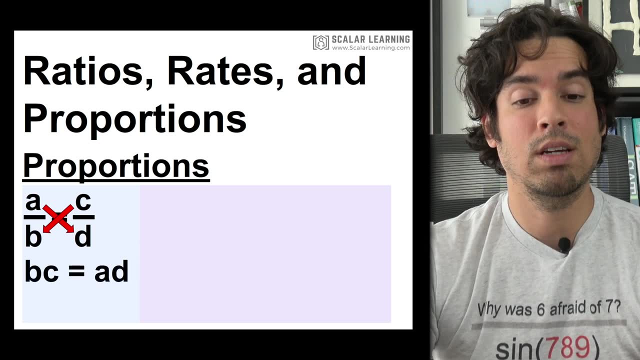 Now, when we solve a proportion, we always want to cross multiply. That literally means the variables are crisscrossing, jumping across the equal sign to multiply each other. And when they do jump across, you have a nice, simpler equation of B times C. So you see how the C jumps down to the B. It's B times C equals A times D. 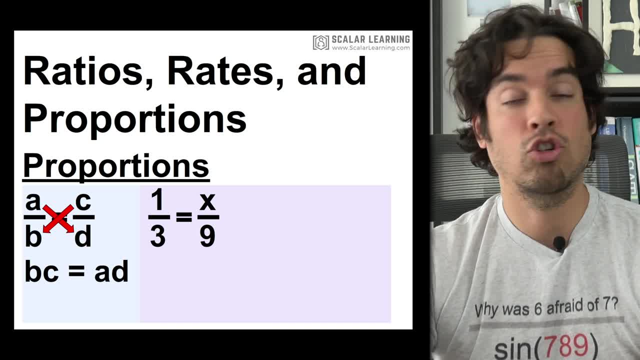 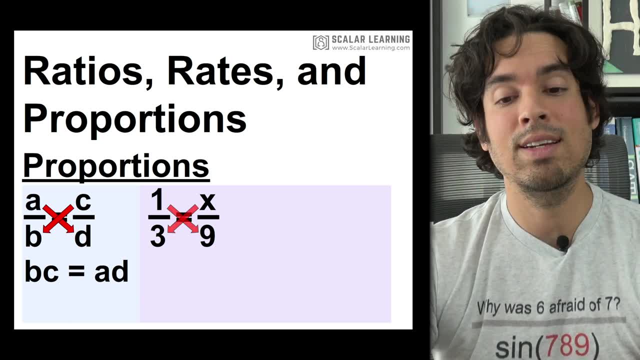 So we put this into practice. Let's say, we're given a proportion as such, You set up a proportion, like we did in the last example. All we do to solve is cross multiply, Right. So the one multiplies the nine and the X multiplies the three. And now we have a new. 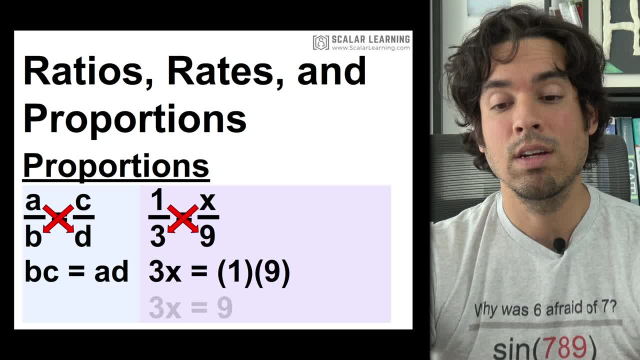 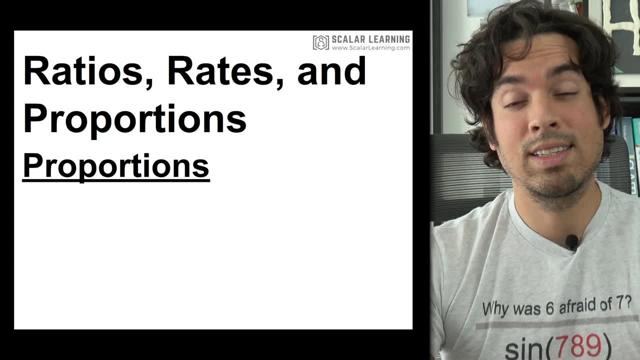 equation of three X equals one times nine. So to simplify, we have three X equals nine And of course this gives us X equals three. Continuing on with an example for proportions, Let's take this example. We said: if seven pounds of plums makes eight, 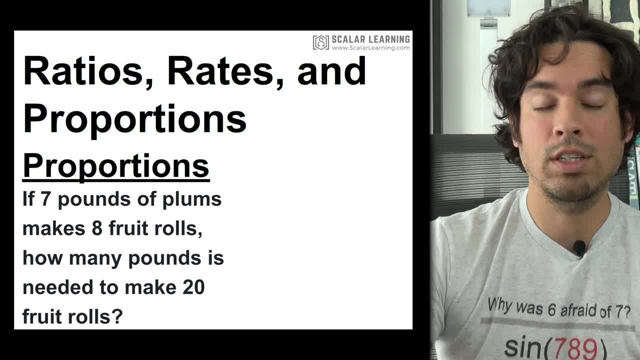 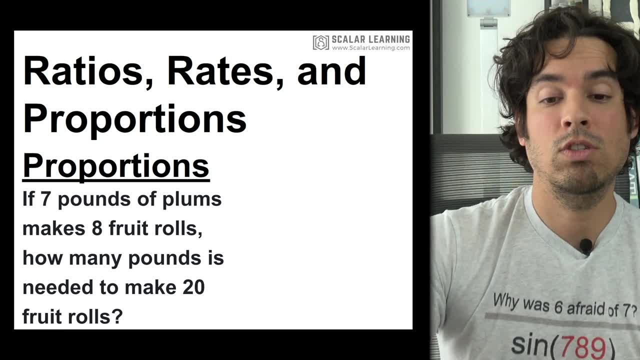 fruit rolls. How many pounds is needed to make 20 fruit rolls? The first thing you want to do before you set up a proportion is set up your category. So now we're talking about pounds of plums and corresponding fruit rolls. So we want to sort of break down those categories. 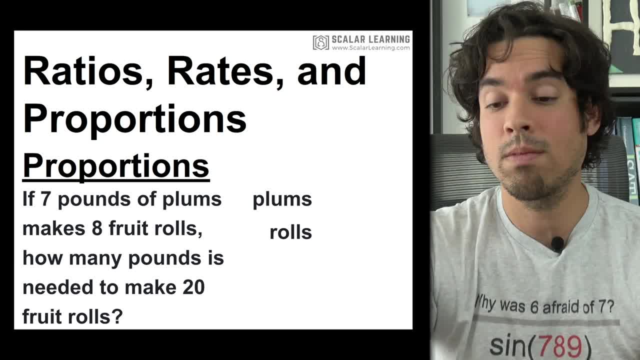 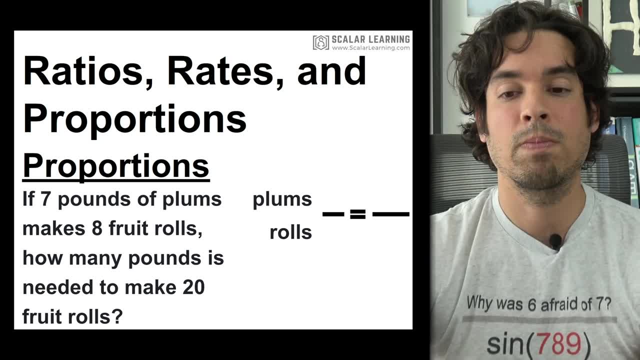 And it's arbitrary. I could have put rolls on top. I ended up putting plums on top. It's just arbitrary. So now we've made that, Now we get our framework for the proportion Right, Because we know it's going to be a fraction equals a fraction. Well, I know on the left side I've got seven pounds of plums to make. 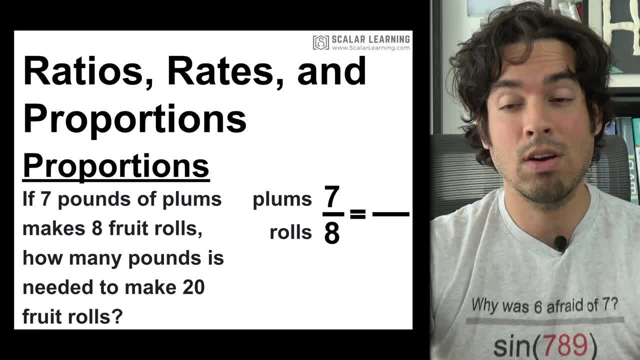 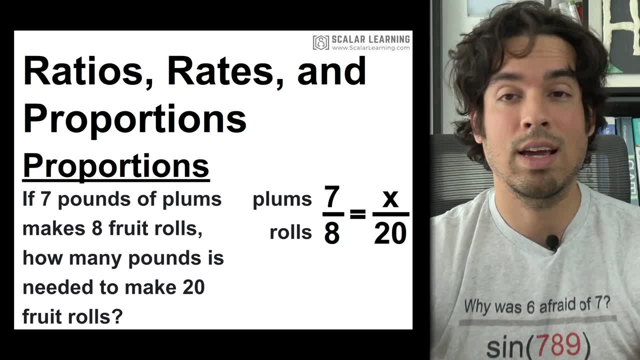 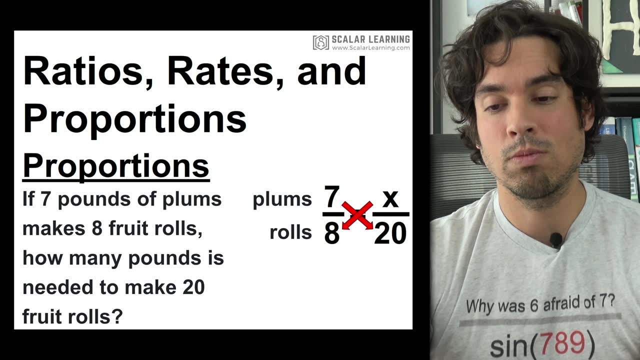 Eight fruit rolls. So you notice how those two are together. They're paired up And on the other side we need to make 20 fruit rolls, But I don't know the amount of plums we need. That's why there's an X in that position. All right To solve for this. we again cross multiply, So then the X jumps down and the seven jumps across and down and we get eight. X equals seven times 20, which is of course 140. 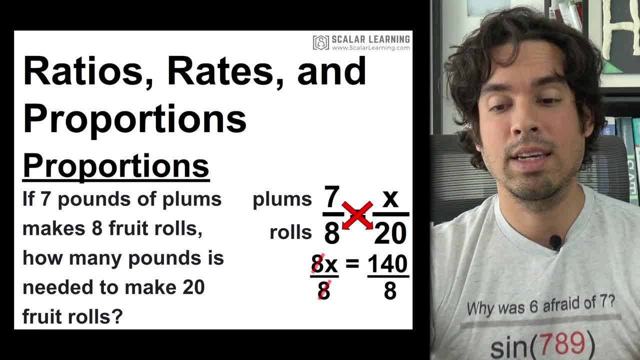 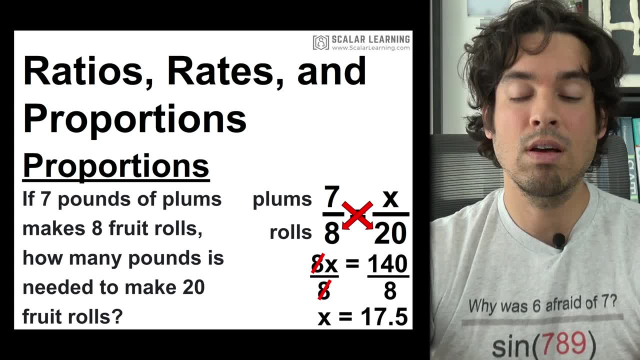 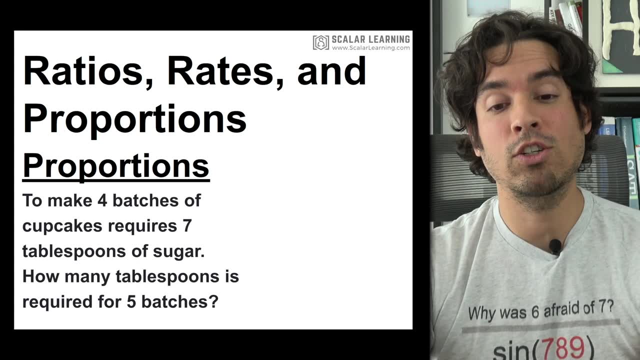 Last but not least, we divide both sides by eight and I get X equals 17.5.. So the answer is: it takes 17.5 plums, or pounds of plums, to make those 20 fruit rolls. Now we'll jump into another example here. It says to make four batches of cupcakes requires seven tablespoons of sugar. 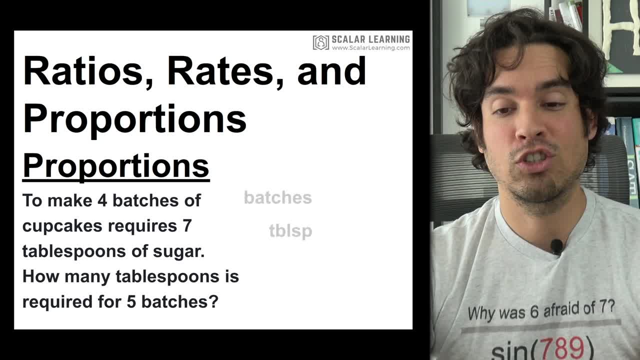 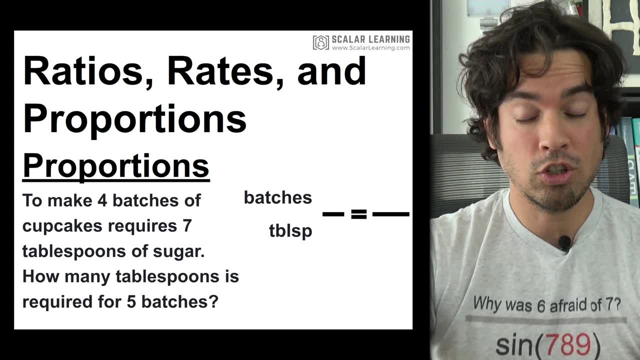 How many tablespoons is required for five batches. All right, So let's check it out. We again set up our framework. We've got batches on top, tablespoons on the bottom And there's our baseline structure. So we see that we've got four batches for those and required. 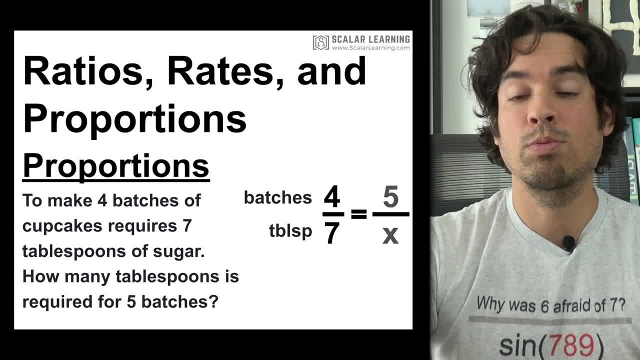 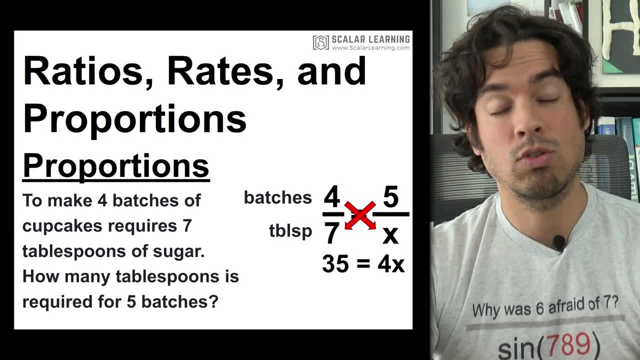 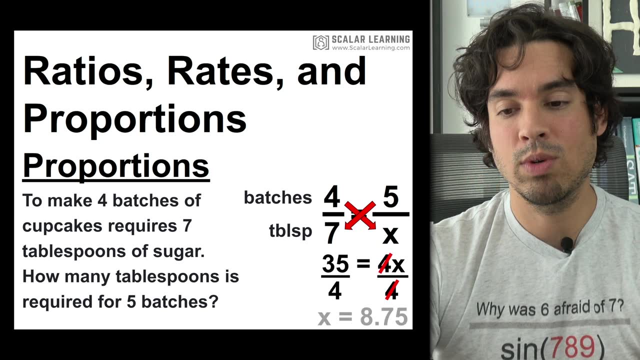 We've got our seven tablespoons of sugar. Now we need to make five batches. but we have the tablespoons is unknown. All we got to do now is cross, multiply boom, and we get five times seven is 35 equals 4X. Last but not least, isolate by dividing by 4.. Boom, Cross those out and we get X equals 8.75. 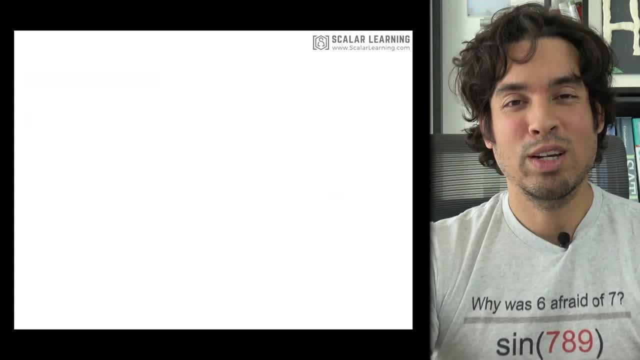 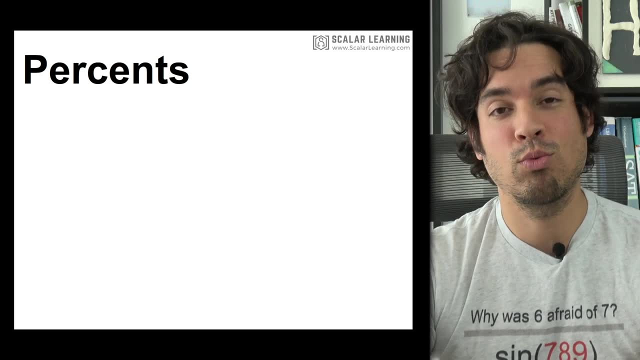 so it's 8.75 tablespoons of sugar. Now we're going to talk about percents. This is such an important category on the SAT. about percents, i always go back to what my french teacher told me in high school, which is percent is. 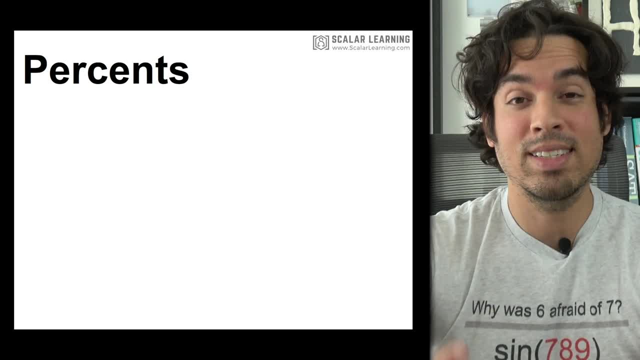 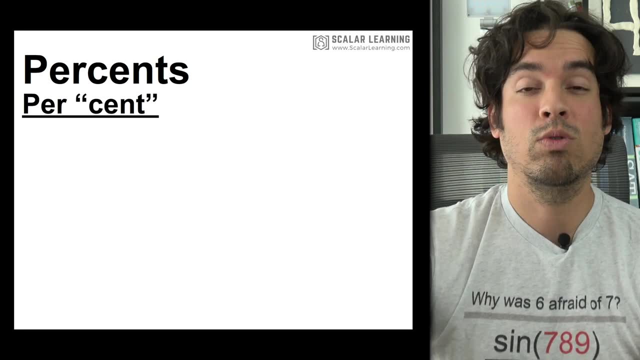 a french word and it translates directly or what you the right way to say it is. and that song part- okay, that separated song part- translates directly to a hundred. so really we say percent, we're talking per 100. so that's a very important thing to remember when we're trying to understand percent. 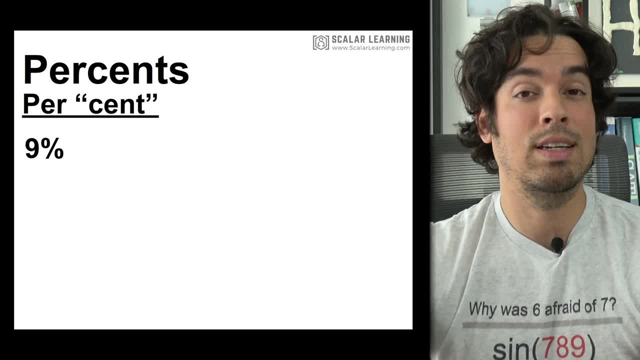 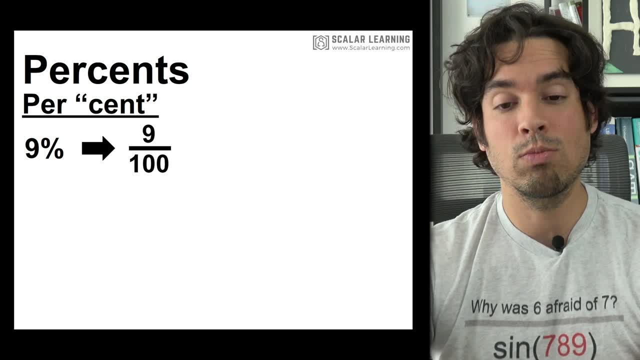 so like, for example, when we say nine percent, we're really saying nine per hundred, so it's really nine out of a hundred. okay, nine hundreds, and if we wanted to write that in decimal format, it's simply 0.09. again that nine goes in the hundred spot, another quick way to think about. 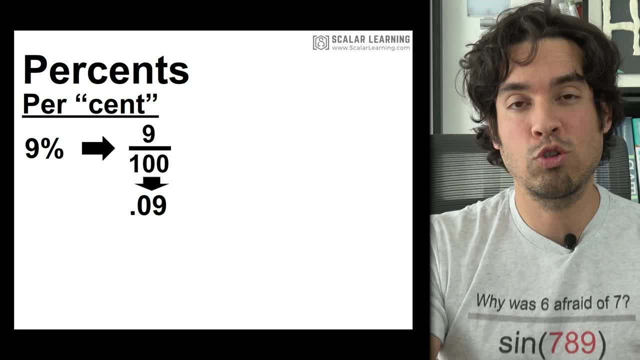 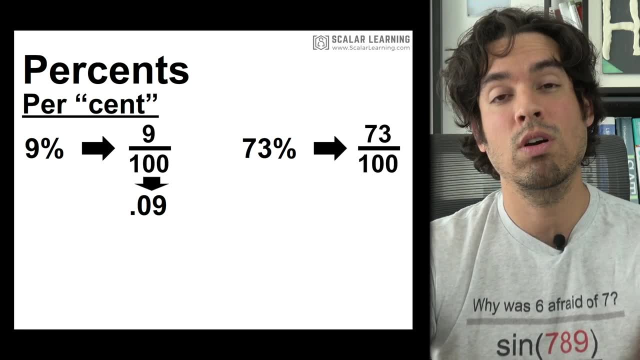 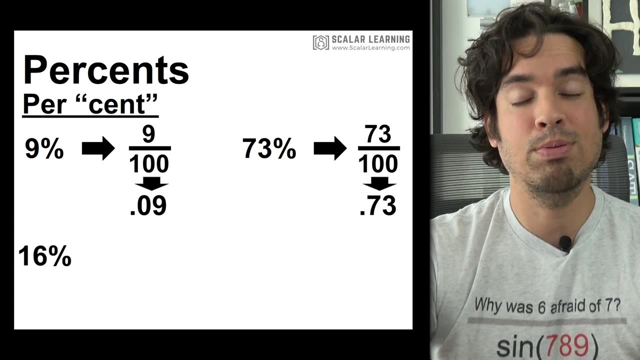 that, when we go from percent to decimal, is removing the decimal two spots to the left, but we're going to talk more about that in a second. likewise, 73 percent is simply 73 per 100 or 73 hundreds in decimal format. once again, point seven, three, sixteen percent would be. 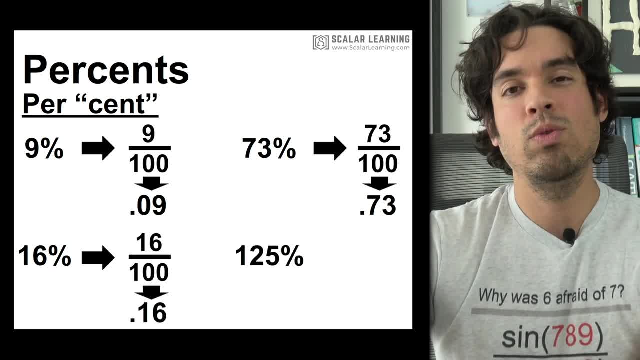 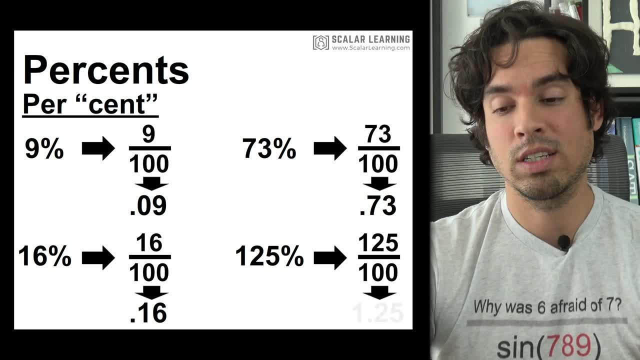 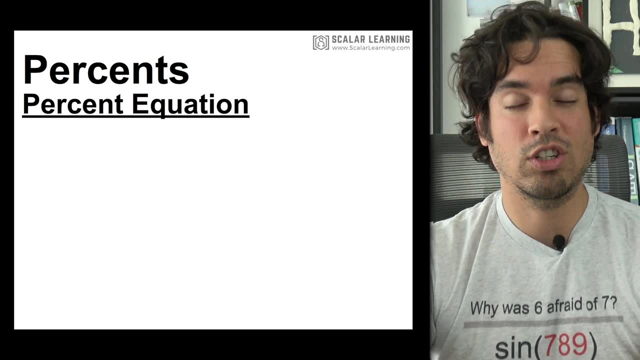 Sixteen hundredths, or point one, six, and then, when we get to numbers bigger than a hundred, we still move the decimal only twice. So it's a hundred and twenty five hundredths, which translates to one point two, five. When we solve for percents, I like to use something called the percent equation. 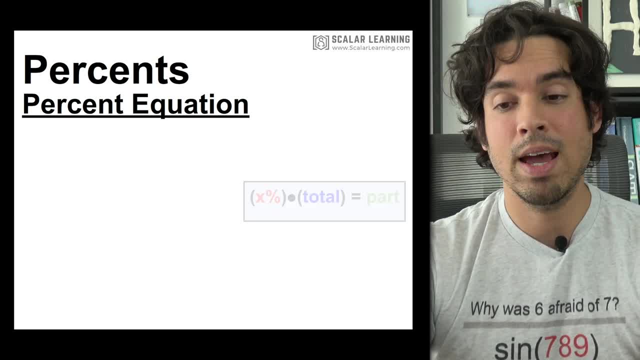 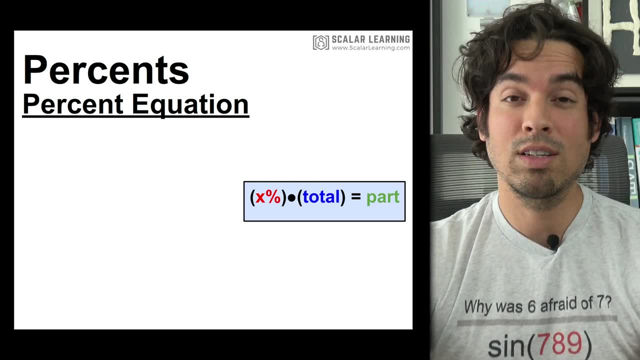 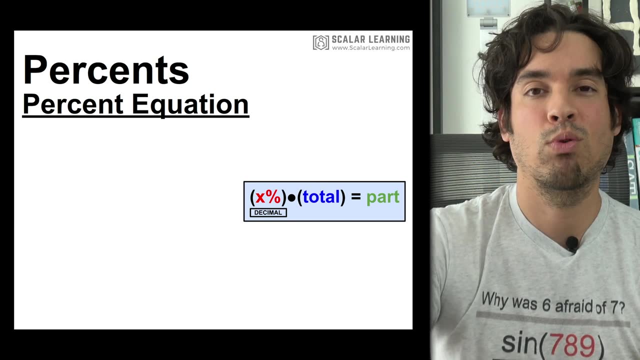 This is what I highly recommend, especially for the SAT level type of math. The percent equation is very simple. The percent times whatever the total is gives me the part. The only thing you remember is the percent goes in in decimal format. So, like we saw before, sixteen percent is point one six. you plug in point one six into this equation. 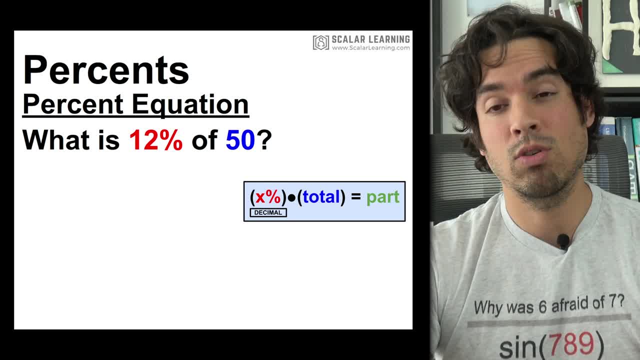 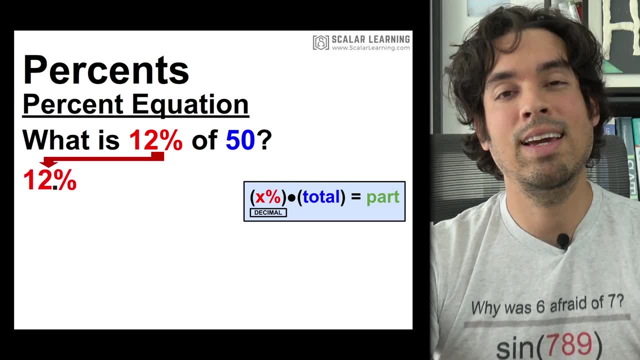 So when we ask a question- what is twelve percent of fifty- and notice how it's all nicely color-coded, that twelve percent, That's the percent part that's going to come down first as twelve percent. But again notice where the decimal is and notice where it needs to be. It needs to be moved two spots to the left. 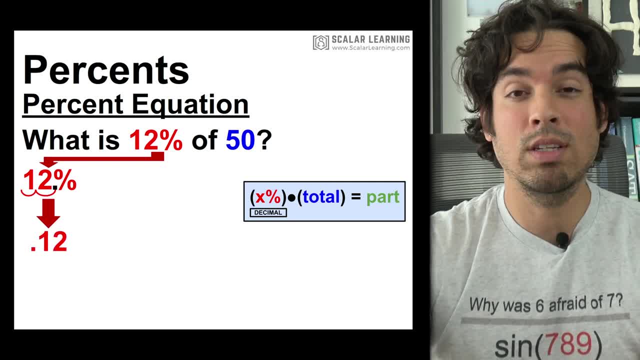 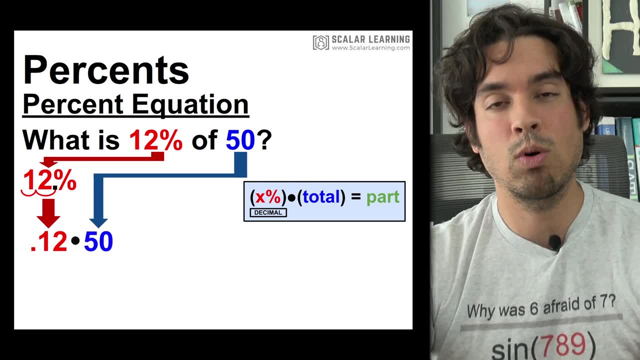 So alright, so now it's really point one, two. now It's in the equation, in the right format, and then we've got the total, what is twelve percent of fifty, So fifties coming next, and it's going to be multiplying that point one, two to get my answer, which is, of course, six, right? 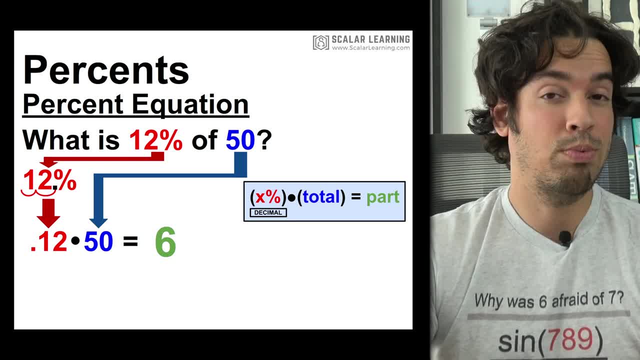 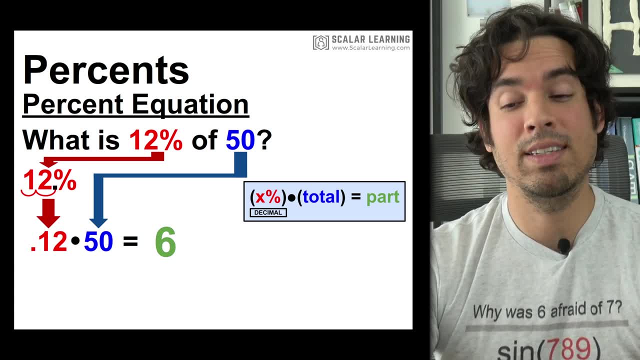 This is sort of like it's the same thing as multiplying five times one, point two, or point five times twelve, if you'd like to manipulate Numbers that way. So there we go. 12% of 50 is indeed six. another way to use the percent equation is in a question like this: 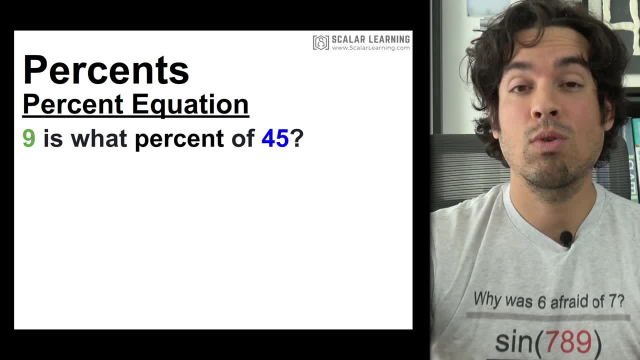 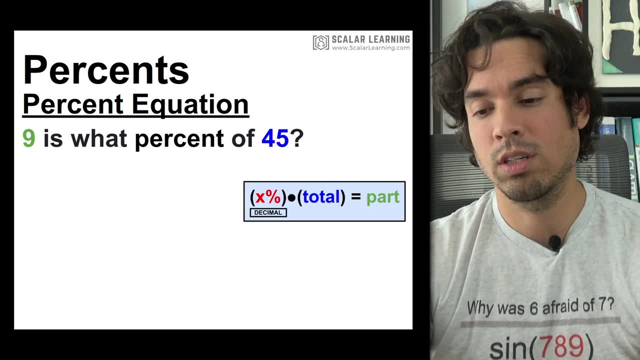 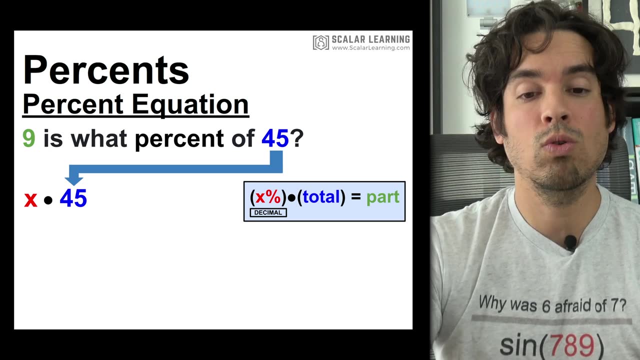 Where it says: nine is what percent of 45? now we're actually trying to solve for the percent, But the beautiful thing is we just use that same percent equation- decimal version, of course- for the percent We're good to go. So in this case, the unknown is the percent. it is what percent of 45? 45 is still that total. 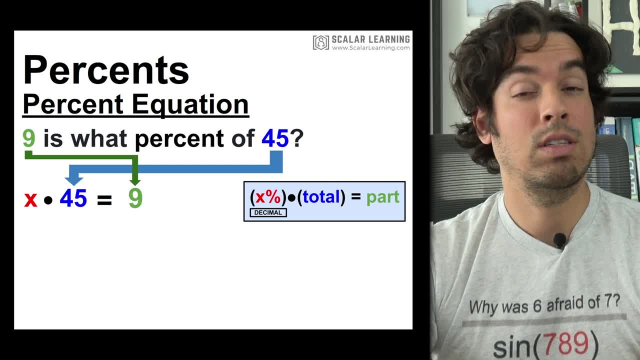 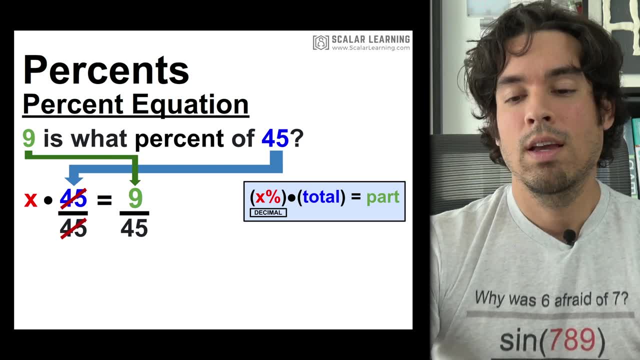 Equals nine, right, All right. Now we got to figure this out simply by isolating. So how many get gonna get rid of that 45? we divide both sides by 45, cross those guys out and X equals. As they guess, it's nine. forty-fifths. 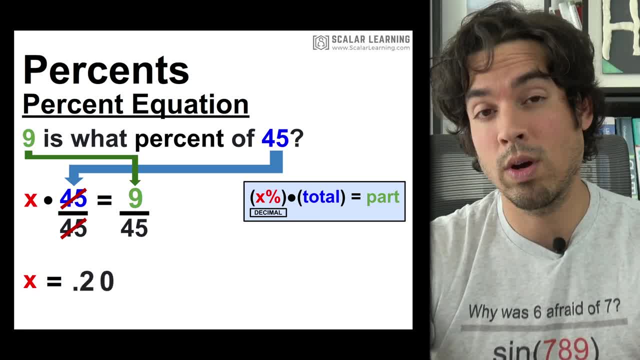 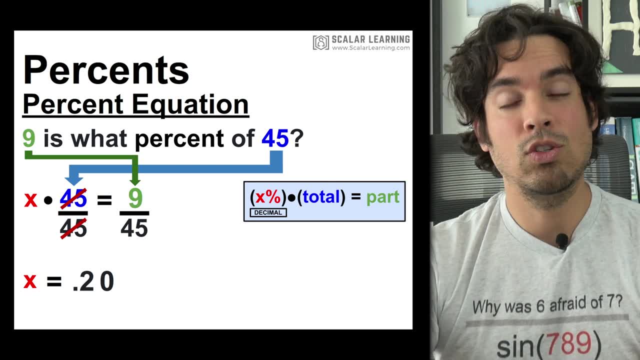 But as a decimal it is point two or point twenty. same thing, Right, if I add a zero, because one-fifth in decimal format is of course point twenty. and then, last but not least, to convert it To its appropriate percentage, just like before, was moving the decimal two spots to the left. 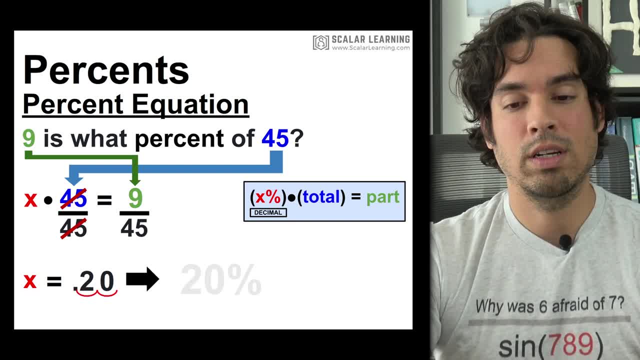 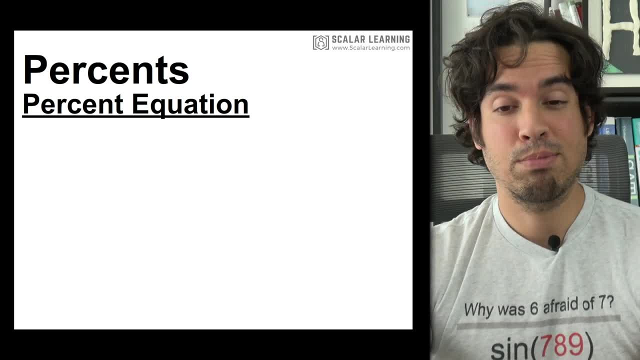 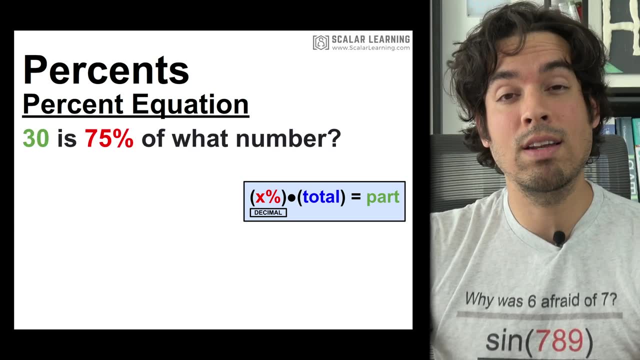 Now I move it two spots to the right and the answer is twenty percent. So again, nine is twenty percent of forty five. Now here's another example using the percent equation. So again, there it is. For your refreshment. it says: thirty is seventy five percent. of what number now? 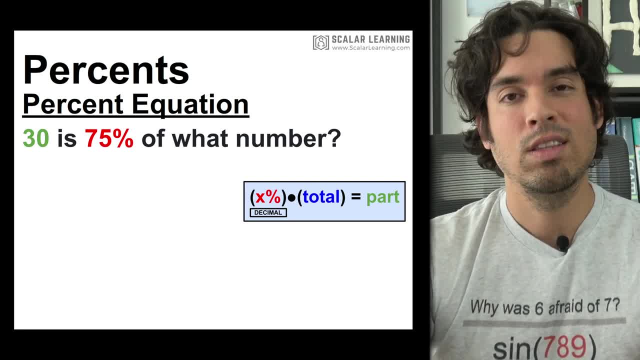 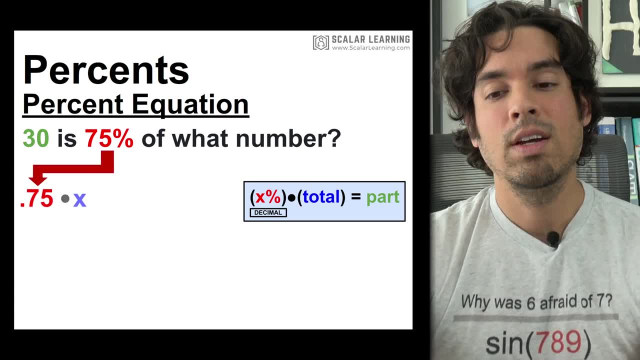 We're actually trying to find that total. you see, the part is there and the percent is there. the total is what's missing. So let's give it a shot. So again we've got seventy five percent in decimal format. That's point seven, five times my total. 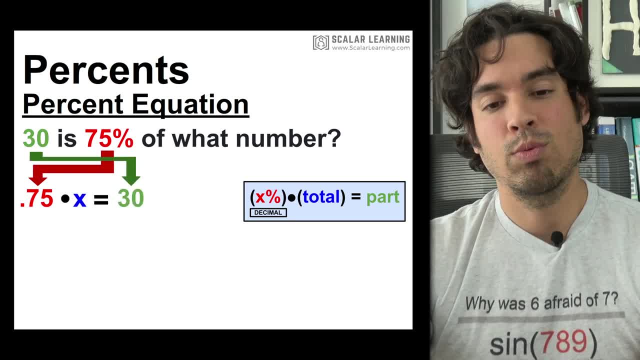 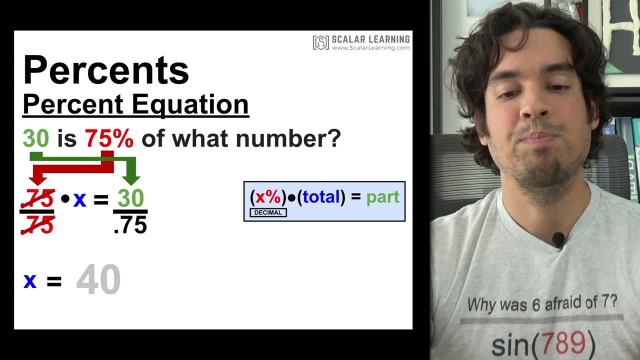 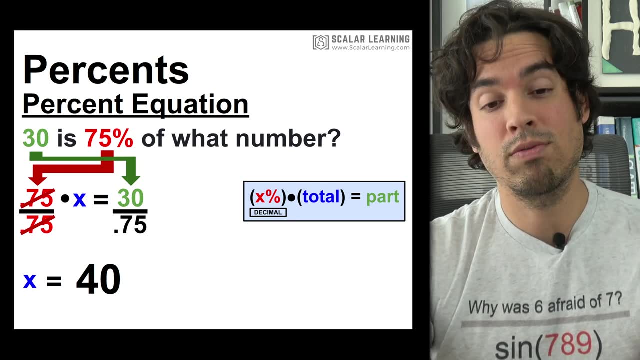 Which is unknown, equals thirty. now what do we do? Of course we isolate, so we divide both sides by point seven, five. and what do we get? thirty divided by point seven, five Becomes forty. So there we go. Thirty is seventy five percent of forty, and that makes sense, because seventy five percent is really three-fourths. 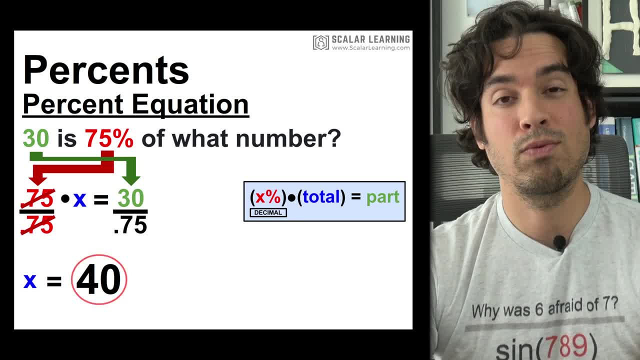 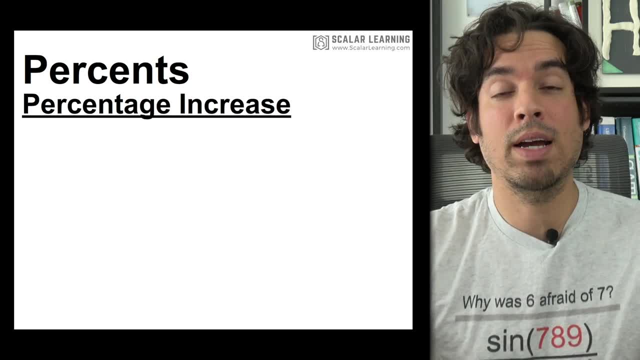 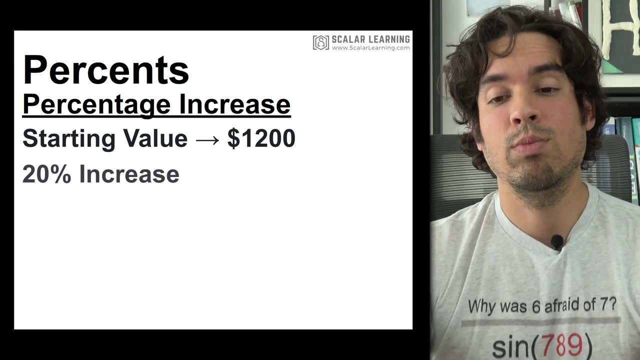 So, of course, thirty is indeed three-fourths of forty. next Let's talk about percent increases. So what is a percentage increase? It means we're increasing the value by a certain percentage. So let's take a look at this example. We have a starting value for any item of twelve hundred dollars, and we know that there's meant to be a twenty percent increase. 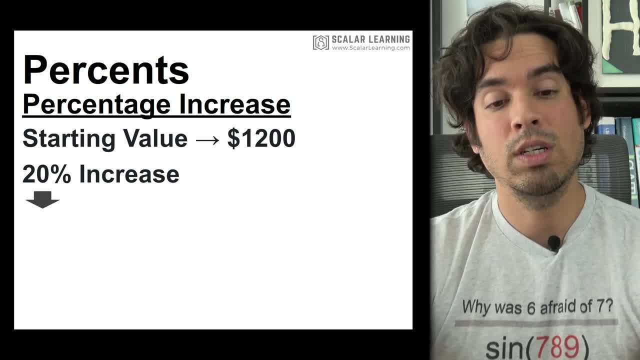 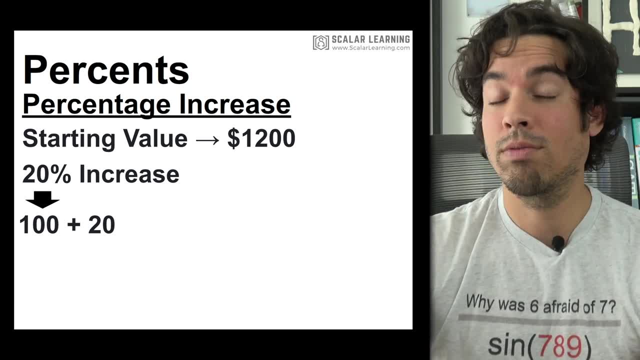 So how are we going to calculate this precisely and efficiently? what we're gonna do is we're gonna take That twenty and we're gonna add it to a hundred. So anytime we've got an increase, we're gonna add that value to a hundred. now, 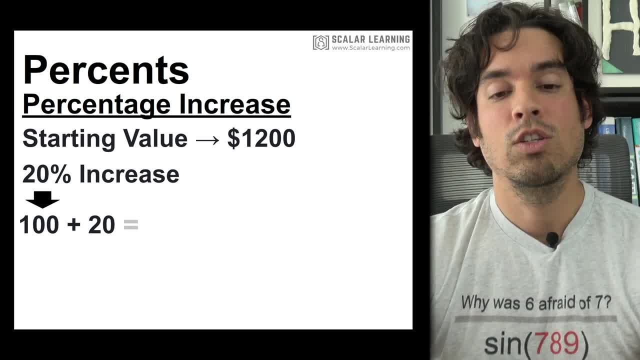 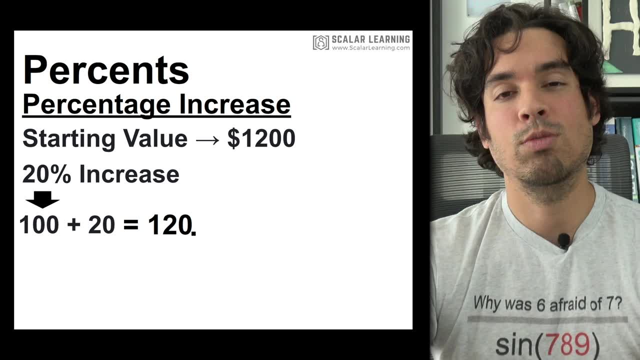 If it was a decrease we'd be subtracting it, but we're gonna get to that in a moment. So we add those two together, we get a hundred and twenty percent. Next we take that decimal and we convert it by moving the decimal two spots to the left. Boom, Boom. 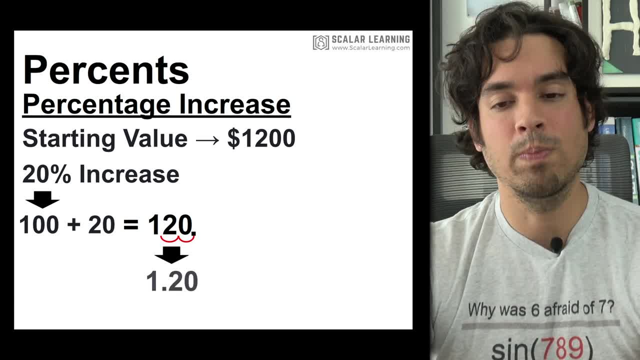 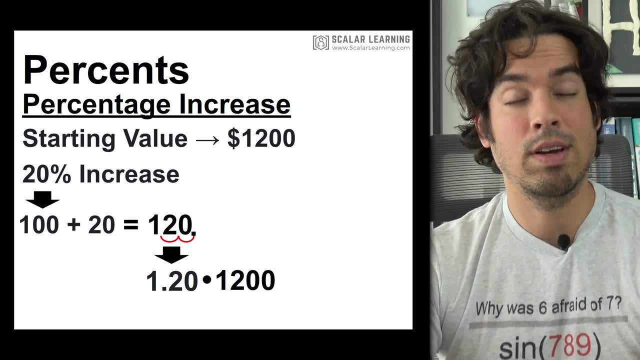 So now, instead of a hundred and twenty we have one point two. Then we take it in decimal format, in keeping with our percent equation, and we multiply it by that starting value, Twelve hundred, to get our final value after the twenty percent increase of fourteen hundred and forty now, 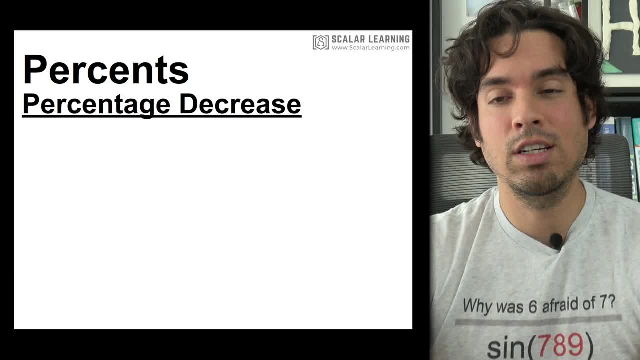 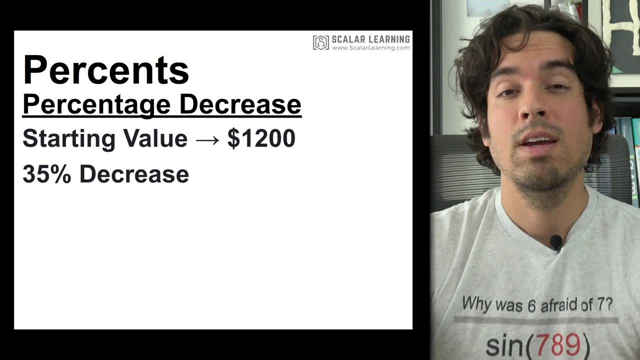 We're going to talk about the other side. We're going to talk about percentage decreases. So in this case we're going to take our same starting value of twelve hundred dollars, but we're gonna decrease by thirty five percent. now It's very important to remember, just like in the increase where we add to a hundred here. 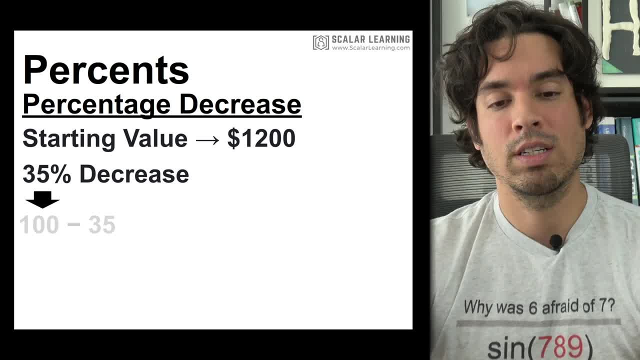 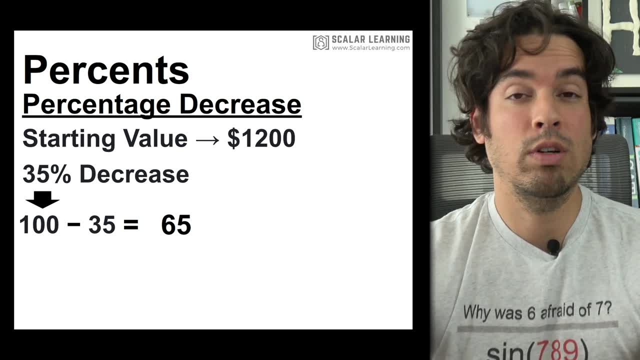 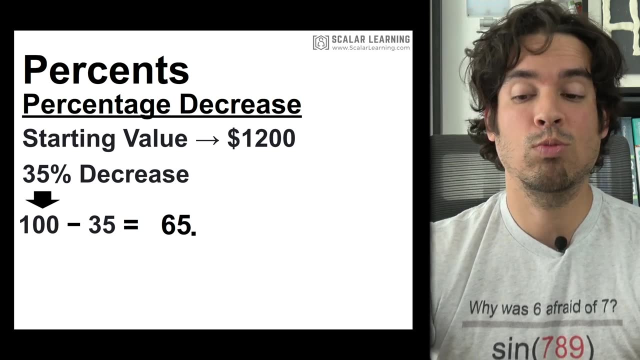 We are going to do the opposite and subtract from a hundred. So we're going to take a hundred minus thirty five, which gives us sixty five percent, and that's What remains when we're removing thirty five percent, where we have a remaining sixty five percent. Okay, Now again, just like with the percent equation before, we have to move the decimal two spots to the left to get the decimal equivalent. 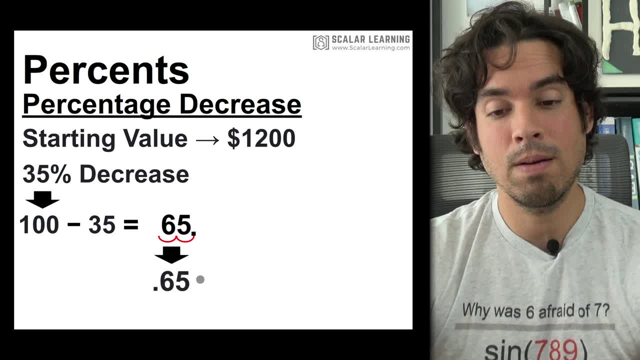 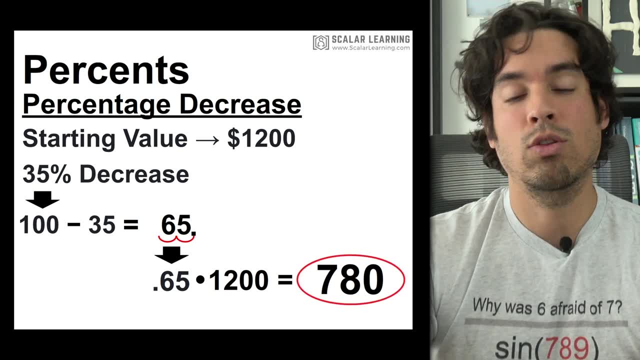 Which is point six five. All right, Now we're nicely set up. We multiply this times that starting value of twelve hundred and we get Seven hundred and eighty. so, at a thirty five percent decrease, from twelve hundred takes us to seven hundred and eighty. next, 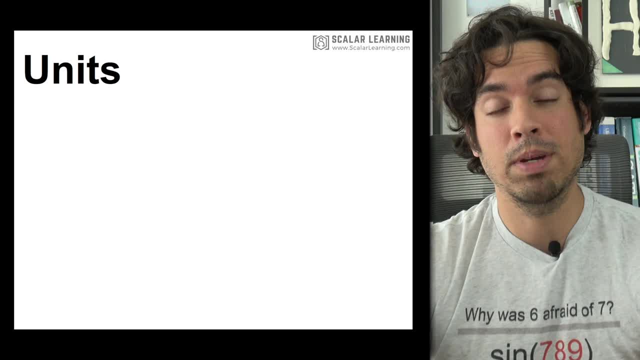 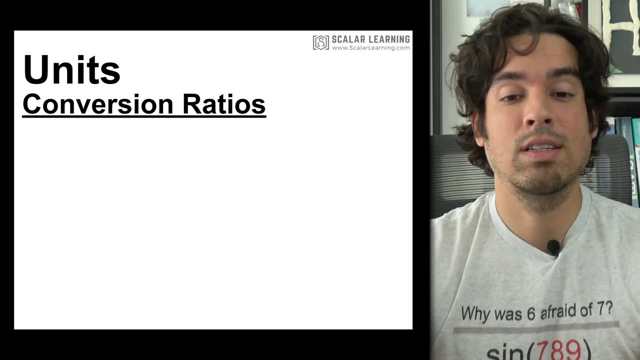 We're going to talk about units and units Conversions. this is a very big section on the SAT and very important to get down these basics. What do we use to convert units effectively? The answer is conversion ratios. All right, so what is a conversion ratio? 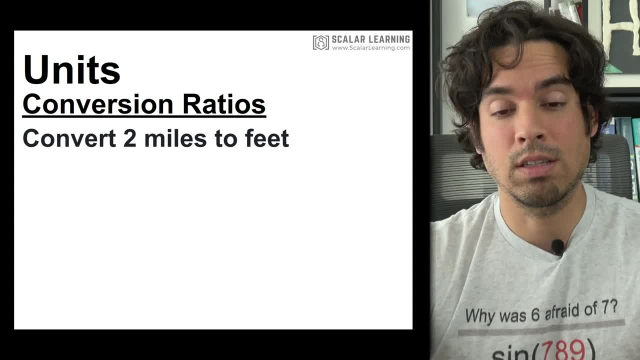 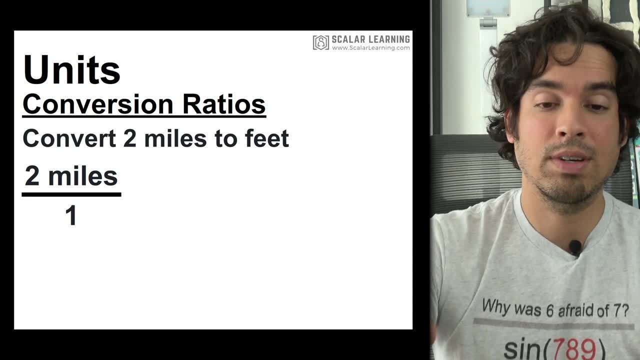 Pretend they said: convert two miles to feet. All right, So what are we gonna do here? So first we're gonna say, All right, I've got two miles, I need to convert it to feet. I like to throw it over one, just so we have it in a nice fraction format. 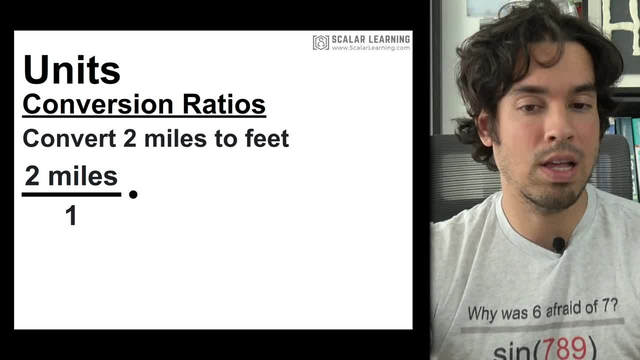 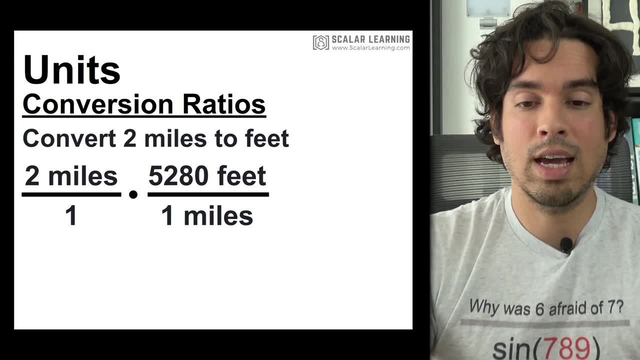 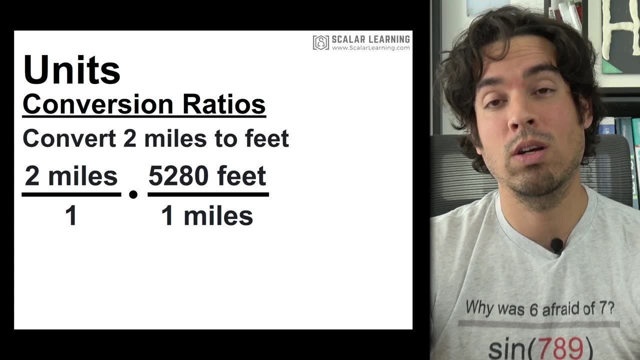 Okay, well, to make that conversion, We've got to multiply by something that equals One. first and foremost because otherwise we change the value. So why did I choose that ratio? Well, because five thousand two hundred and eighty feet actually equals one mile. So technically that is one we are allowed to multiply with the end. 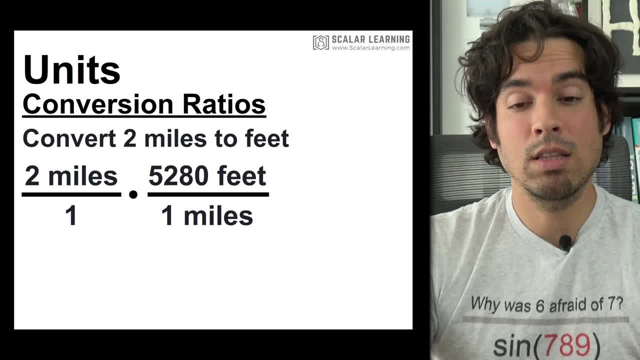 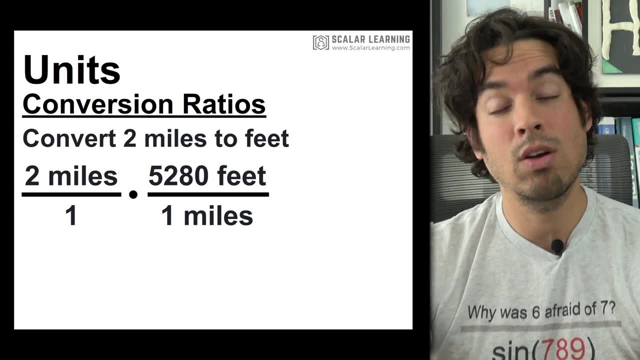 It doesn't change the value and also the fact that I've got miles on the bottom. That's very important because I want the miles to be opposite the miles in the original value. That way we can cancel those out and we'll be left with feet, thereby completing the conversion for the ratio on the right. 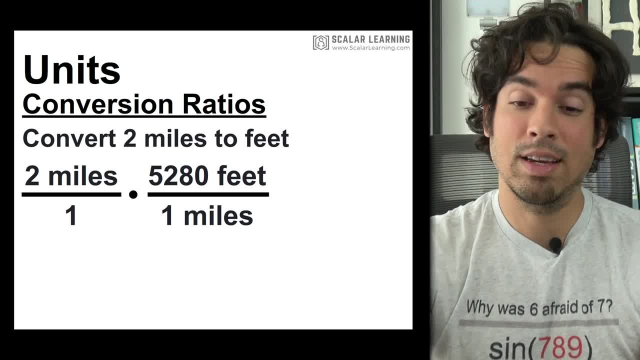 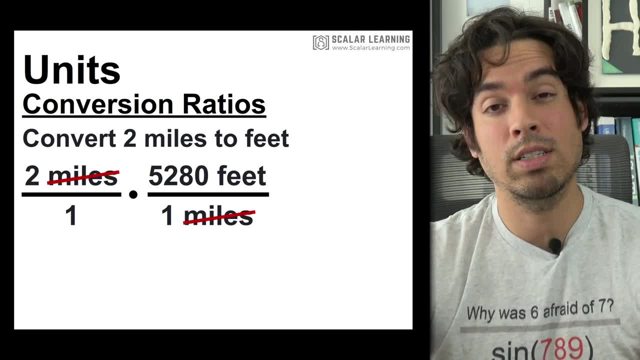 I've got five thousand two hundred and eighty feet over one mile and yes, I know it is singular, but I just had to keep the units looking the same. So now we are going to cancel out those units because we got miles on the top, miles on the bottom and we are good. 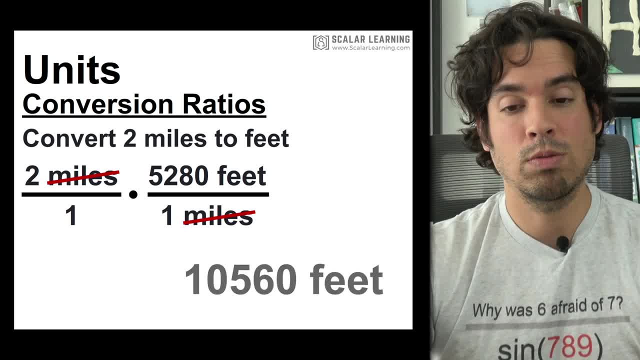 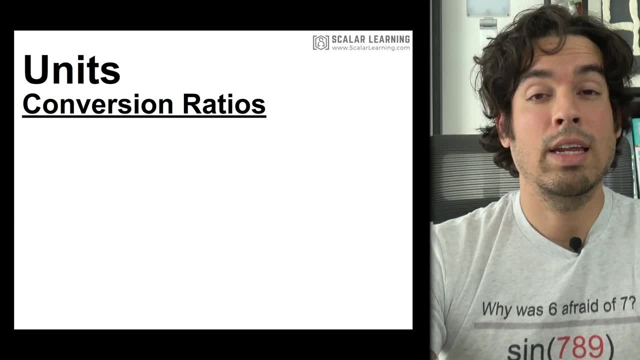 To go. and then, once we have that, we see we're left with feet. simply multiply across two times five thousand two hundred and eighty Is ten thousand five hundred and sixty feet. now let's look at a more difficult example involving conversion ratios. So let's say it says: convert three days to minutes. 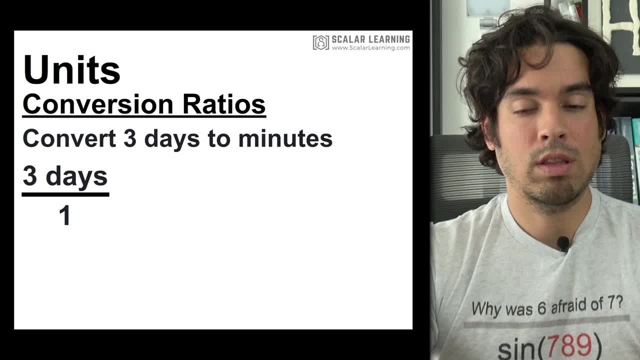 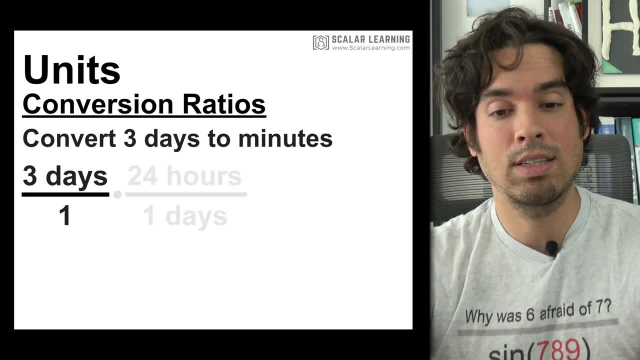 So this is going to involve a few more steps. Let's check it out first. we start with three days and I'm going to do it step by step. I'm not going to go straight to minutes first. I know that it's easy to say we have how many hours in a day. 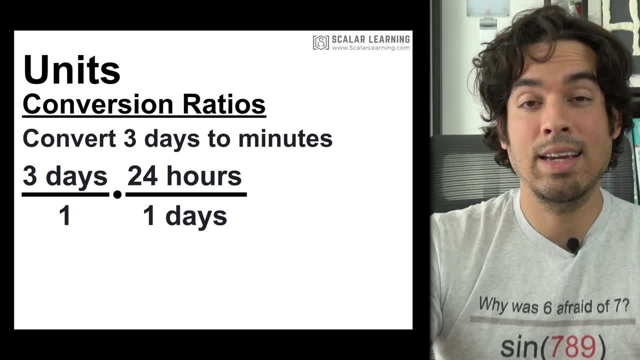 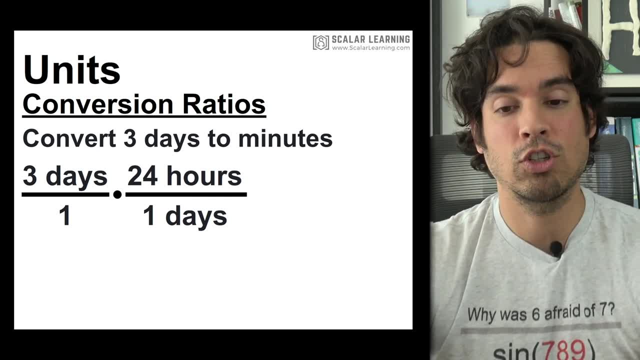 24 hours in a day and notice again, the day is going on the bottom, So it's on the opposite side of the days in the in that first ratio. So that way they're going to be able to cancel out eventually then now I've taken it from days to hours now. 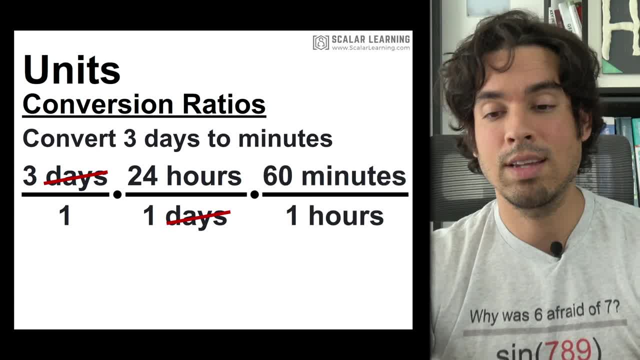 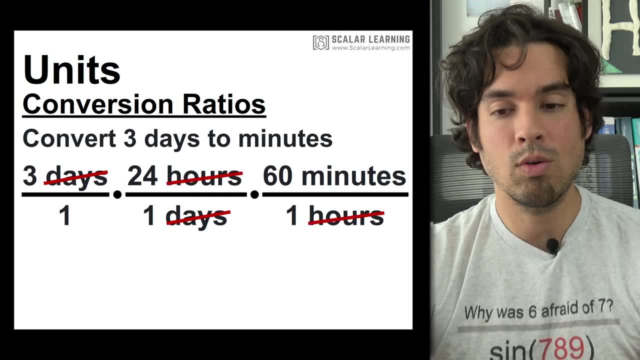 I can complete it by going from hours to minutes. so we have this next one where, again, hours has to be on the bottom and the Equivalent amount of minutes- 60 minutes- is on top. now We cross, cancel those hours and now we're in great shape. 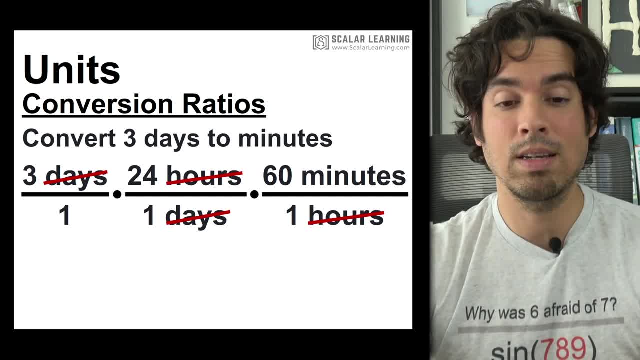 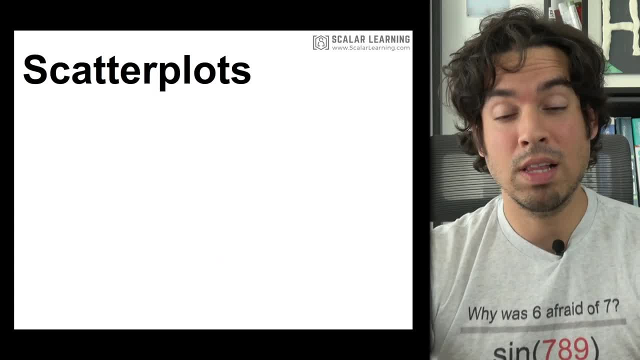 We just multiply across the top three times 24 times 60 gives us four thousand three hundred and twenty minutes, and there it is. We are done. now Let's talk about scatter plots. so scatter plots are amazing. It's a way that we use real data. 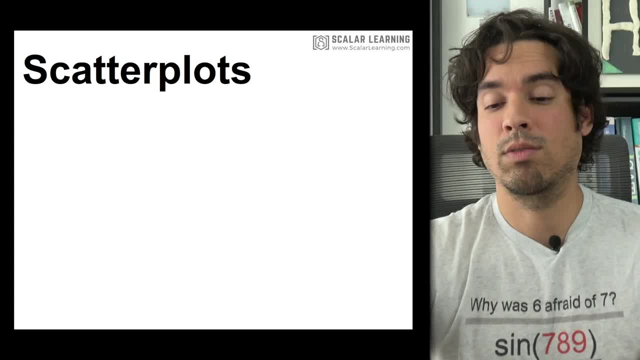 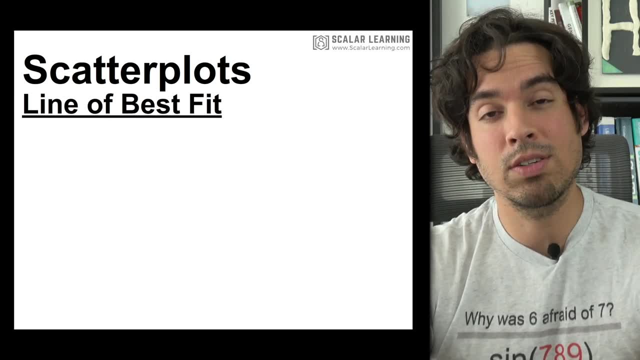 Plotted on a grid and then sort of sit there and analyze and we can maybe make predictions, make lines of best fit, etc. So they're very important. So when we talk about scatterplots, That line of best fit is one of the most commonly tested Subcategories within scatter plots. all right now. 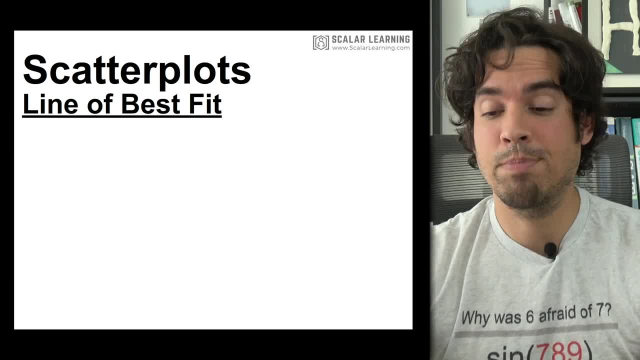 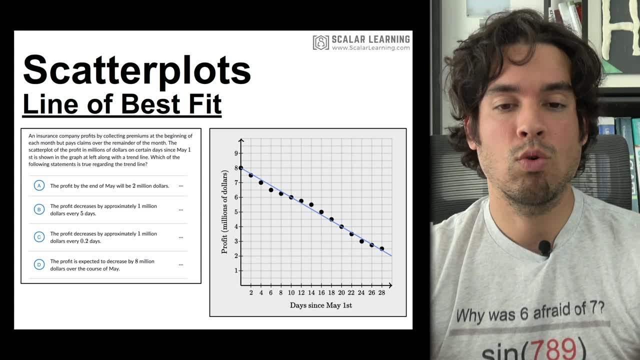 Let's talk about scatter plots in terms of the line of best fit, and the best way to do that is with this example. So you see, here We've got this actual SAT problem and a corresponding chart, and what they're asking us to do is to essentially analyze. 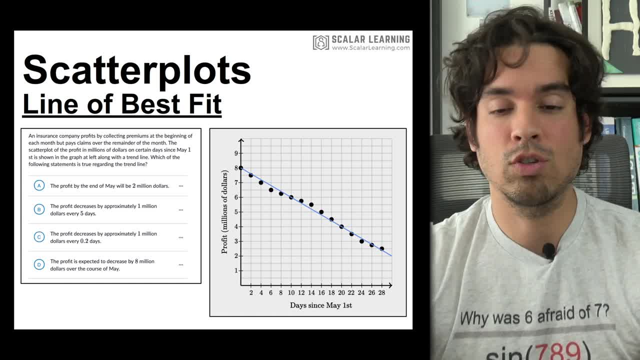 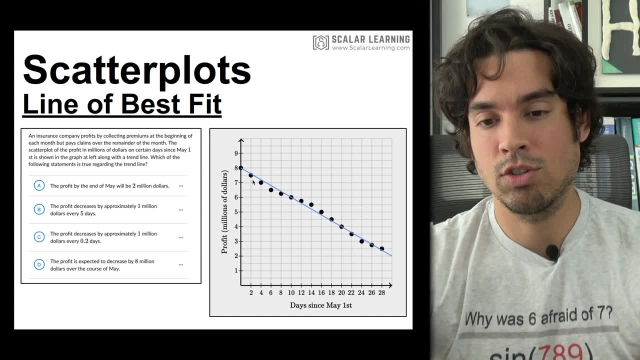 The line of best fit and use that analysis to answer these questions. so we're going to step through that here We. this is kind of superfluous in terms of what we need to answer this question, So just take it as these are real data points. 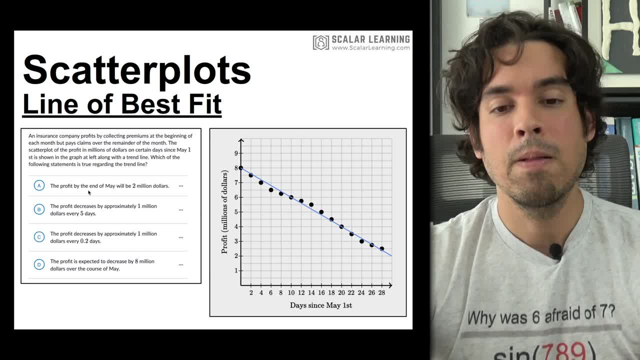 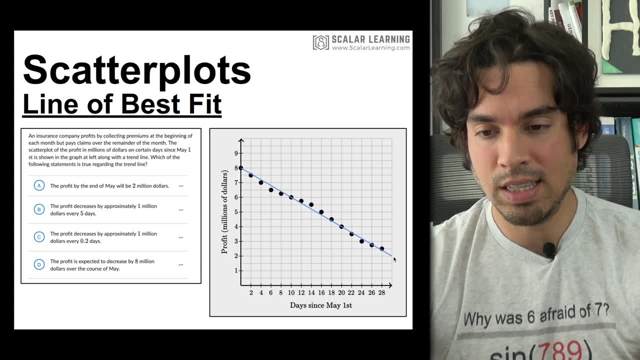 There is the line of best fit and we'll go from there. so first it says The profit by the end of May will be two million dollars. now This almost looks pretty good because we see that this line of best fit hits two million right at the end of May. 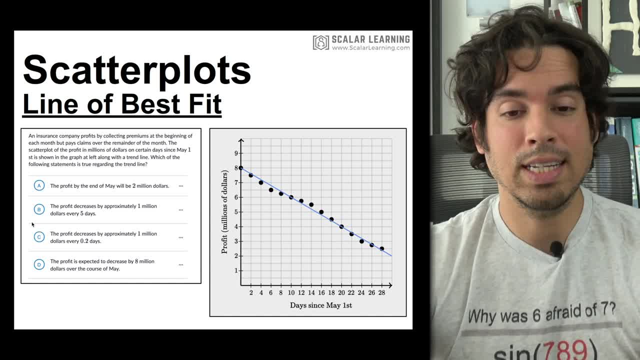 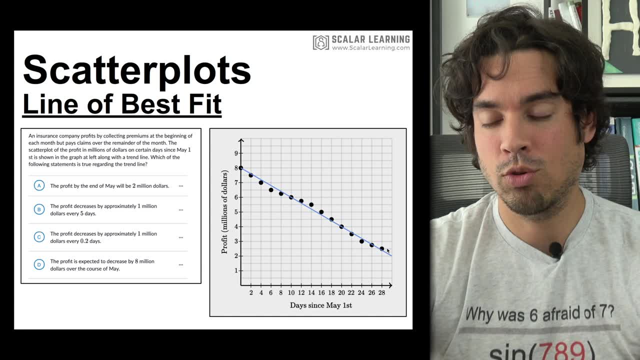 So it's not a horrible choice. the problem is that Definitive language, the problem. the profits by the end of May will be two million dollars. Let's a prediction, We don't know. even right here It's a two and a half million. Maybe it shoots back up. so to make sure, 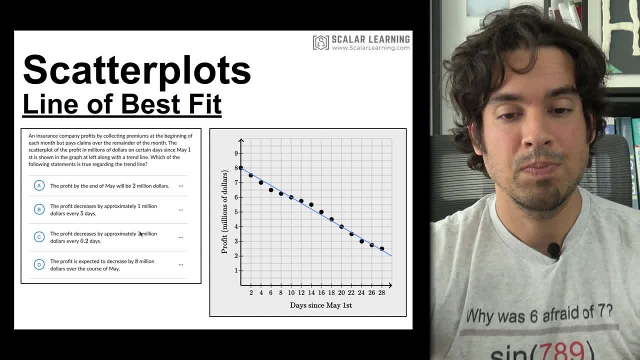 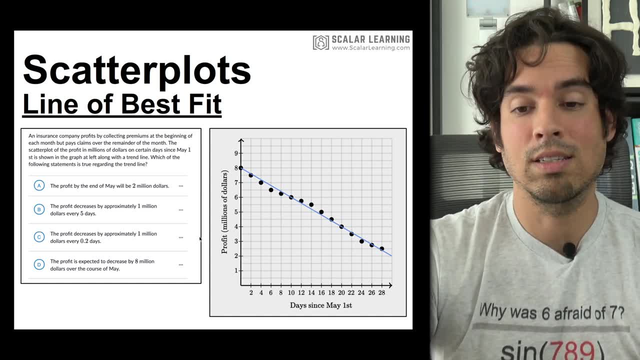 that definitive statement is going a little too far with that line of best fit. Next we're going to look at C. So it says the profit decreases by approximately $1 million every 0.2 days. Now you want to be careful not to look at any of the data points. They're talking about the line of 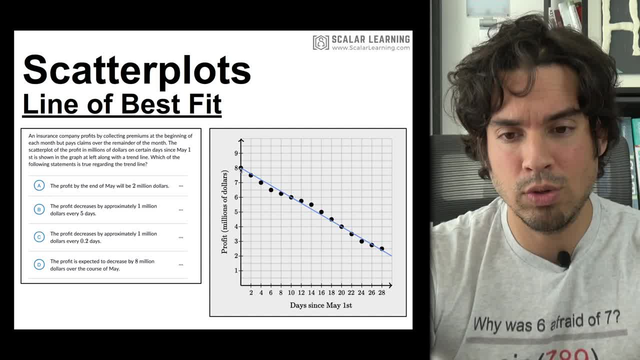 best fits. We got to stick to that. So I'd say in 0.2 days, which might be right here it's saying it's going down by a million bucks. No way, It's barely going down by maybe even a quarter of a. 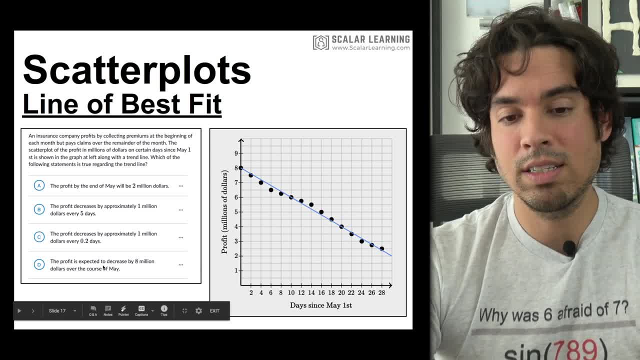 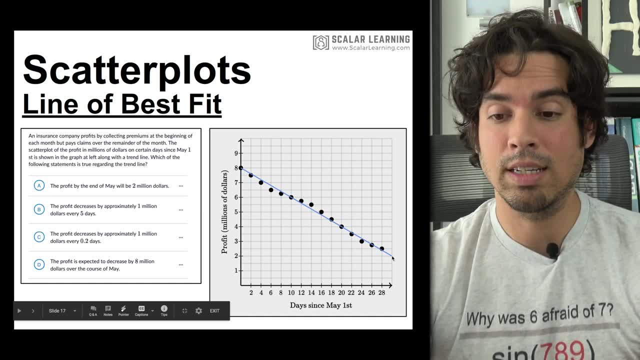 million. So that one's definitely out. Then let's look at D. The profit is expected to decrease by $8 million over the course of May. Well, it starts at a million, but the prediction is that it's expected to decrease only by $6 million, as it appears. So I'd say that's out as well. So let's. 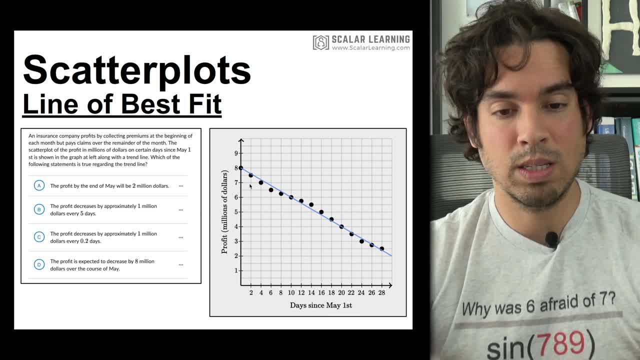 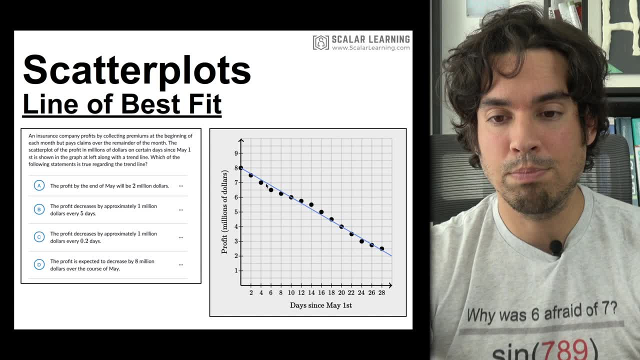 take it back to B B. it says the profit decreases by approximately $1 million every five days. We'll check it out. We're at $8 million. Here is five days right there And boom, looks like we dropped to $7 million after five days. 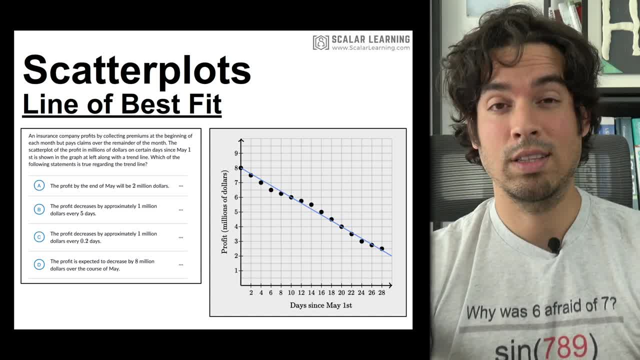 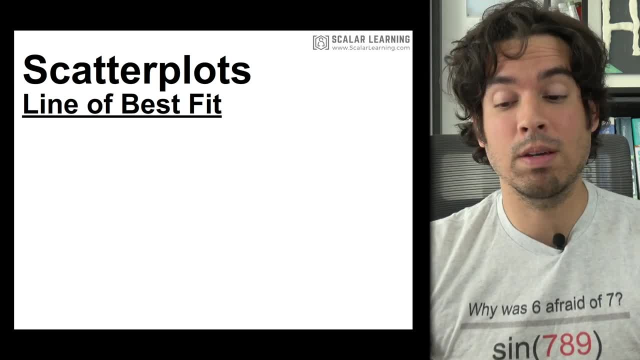 So I feel pretty confident that B is going to be the right answer in this case. Another commonly tested concept in terms of lines of best fit is your ability to draw them in and interpret them, And also not only that, but being able to distinguish whether you've got something that is. 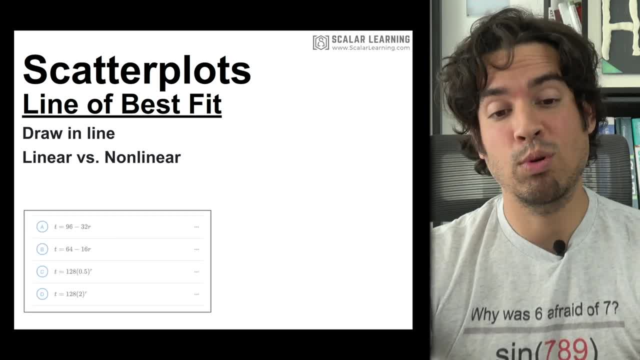 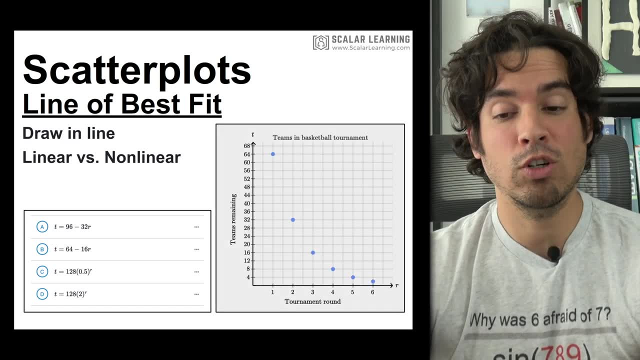 linear versus non-linear, If we take this example. here we're trying to figure out which of these answer choices is what is being graphed to the right. So we're trying to say, hey, which function is a great approximation for these data points? So the first thing you want to do is 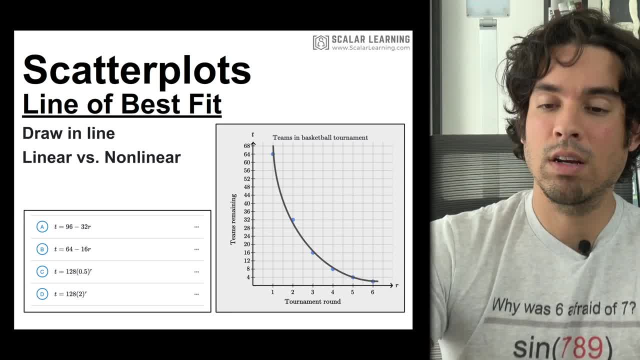 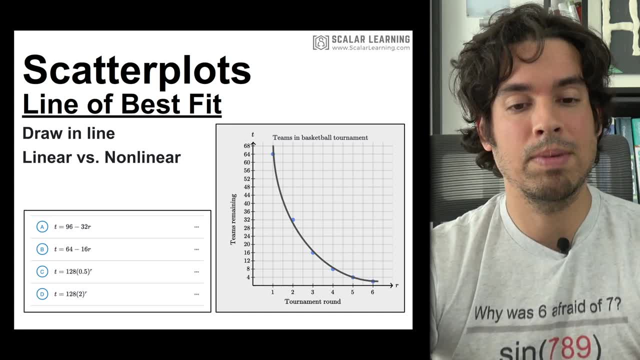 draw in that line of best fit. So we're doing our best there. And does that look like a straight line? Definitely not. It's definitely some sort of a curve to it. So I'm immediately going to eliminate A and B, because those look like linear functions. Next it's down to C or D, and those 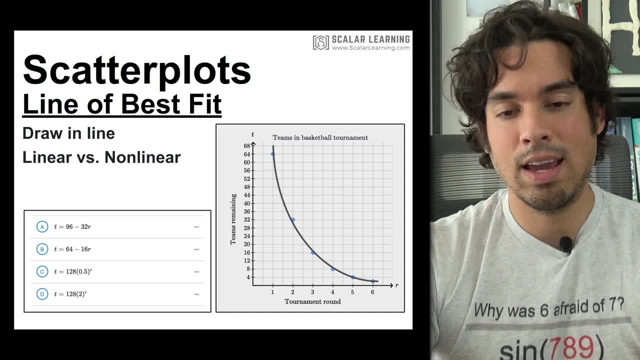 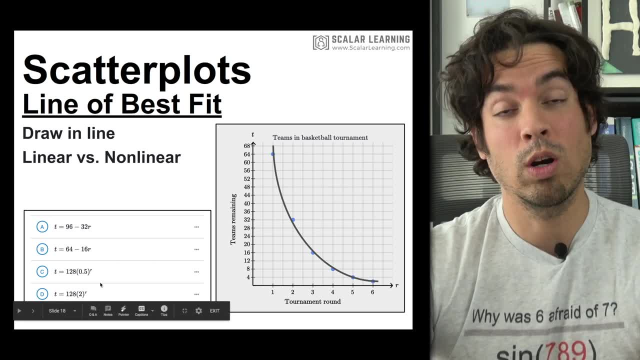 are both exponential, But it looks like it's decay. It's not a exponential growth because it's coming down. In that case, the value inside cannot be something like two, where it'd be doubling every time. It looks like it's cutting in half every time. So 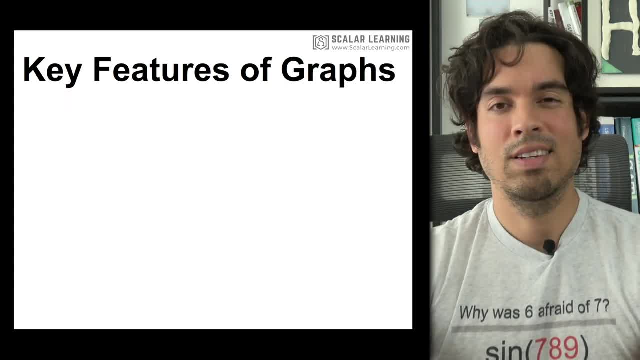 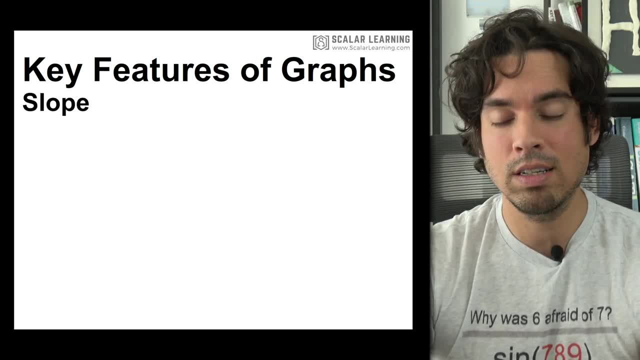 this C value looks like a great answer, and that's it. Next we have key features of graphs, So I want to talk again about some of the most important features of graphs so you can answer these questions pretty easily. So when we talk about slope, we want to break that into two categories. 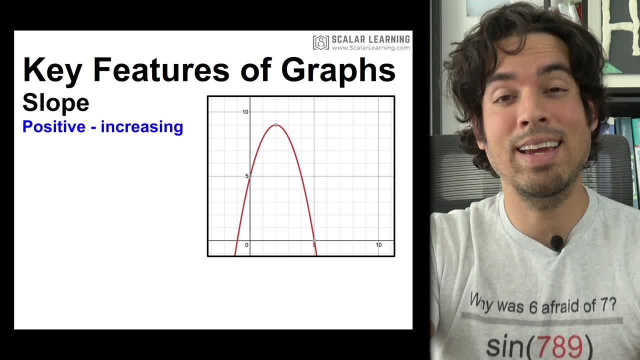 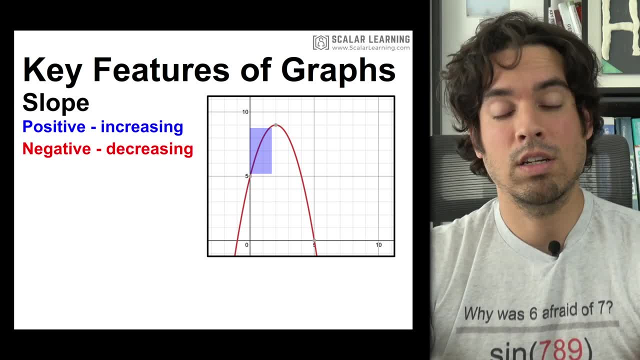 right, So slope, in this case, when it's positive, is increasing. And to give you an example, here's a chunk where it is increasing: It's going up from left to the right, And then it can also, conversely, be decreasing, where it's kind of going down from left to right. If you want to think about. 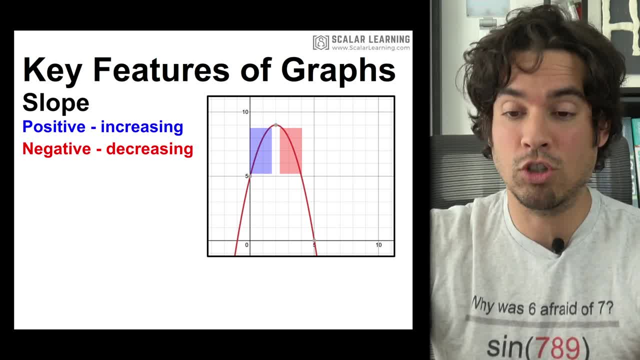 slope. it's going down like a roller coaster. It looks like it's climbing up on the left side and then boom, it's shooting over and going down. So that becomes a negative slope, Of course, if it's totally flat, we. 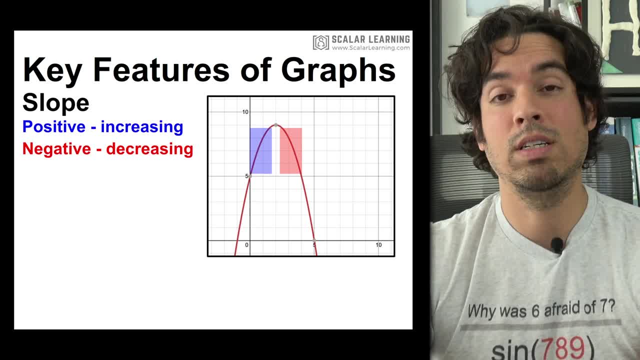 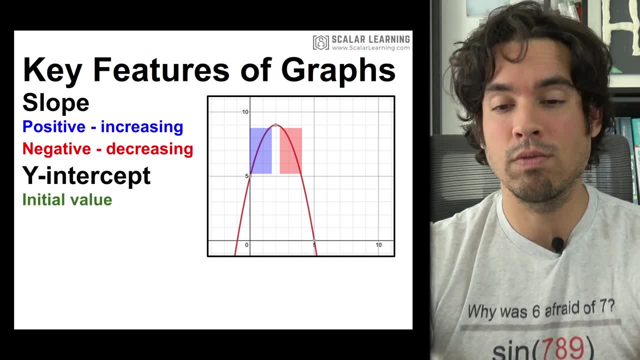 would have a slope of zero and a slope straight up and down would be considered no slope or undefined. Another critical point is the y-intercept, which is always considered to be the initial value. And you see that y-intercept right, there is that green dot. Another important point is the x-intercept and the x-intercept. 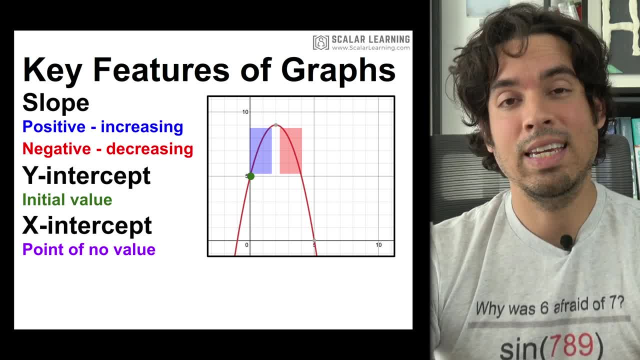 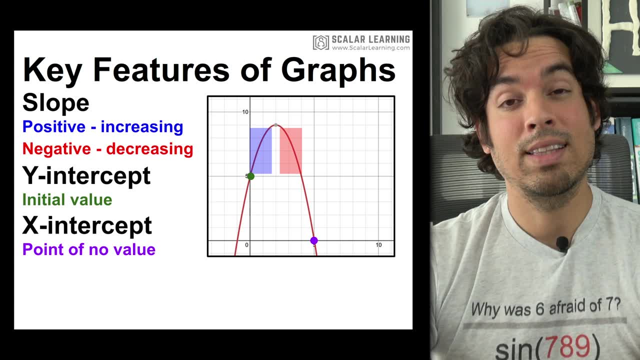 is the point of no value. So the x-intercept is the point of no value And that's where the profit goes to zero and it's denoted by that purple point down on the bottom. Last but not least, specifically for these quadratics, we have the 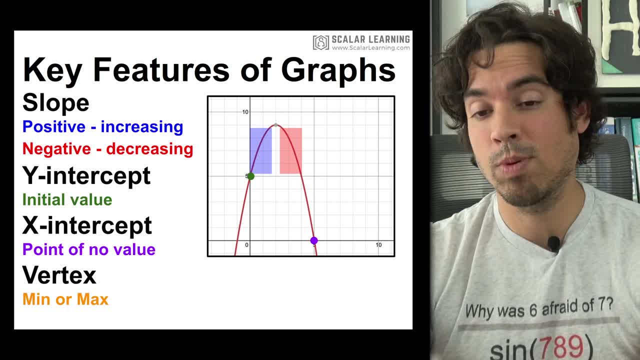 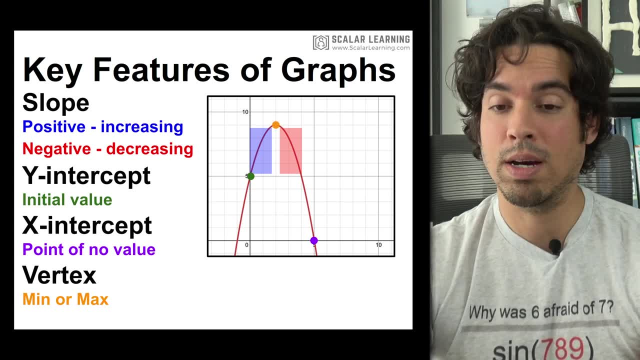 vertex, And the vertex is either the minimum or the maximum point, And of course, in this downward facing parabola, that would be the top of the hill and the vertex would be the maximum, as denoted by that yellow point. Something else that's very important to know is how to differentiate between linear and exponential. 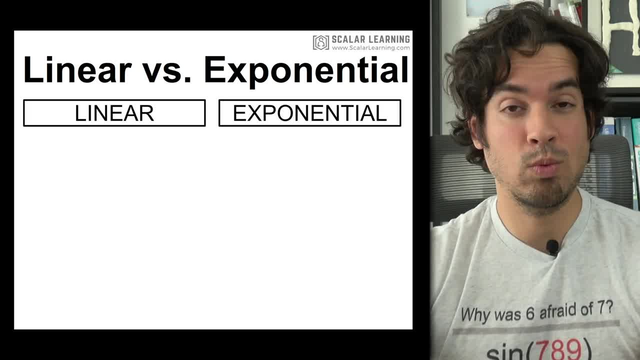 growth or decay. So I got a little table here. One side is linear, One side is exponential And we're going to show you the data here. So first of all, pretend we've got this data: 1,, 2,, 3,, 4,, 5,, 6.. 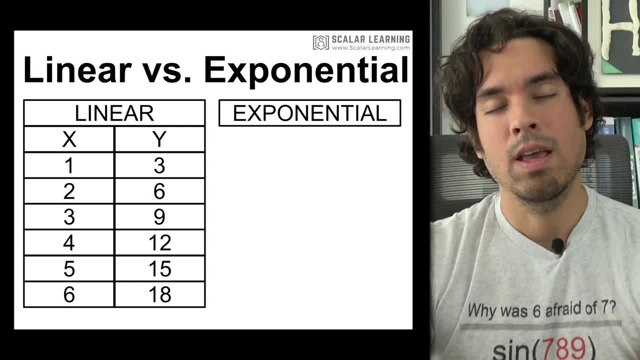 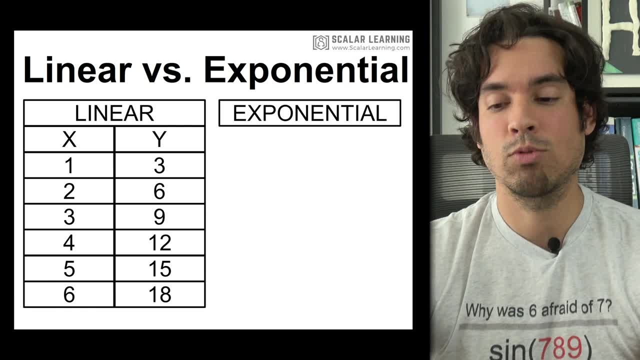 The y's are 3,, 6,, 9,, 12,, 15, 18.. How do I know this is linear? Because it is going up by a constant amount. It's something is being added to it every time. 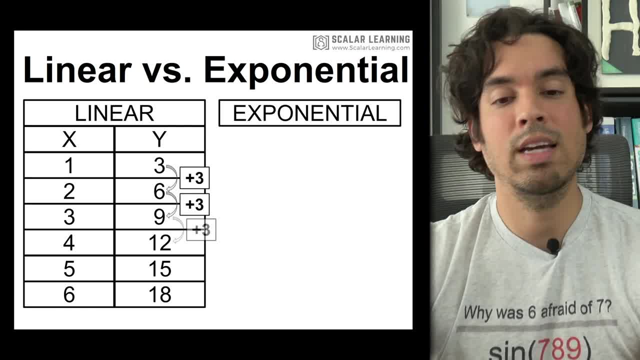 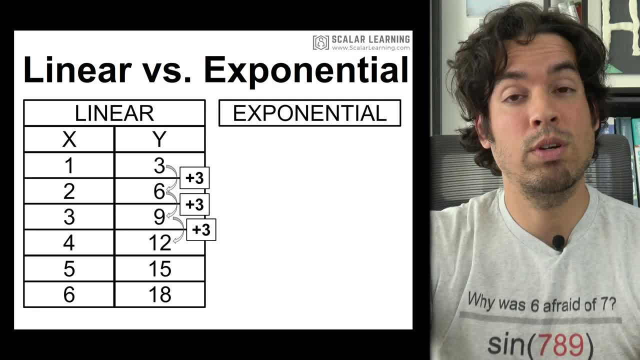 So it's going up by plus 3,, plus 3,, plus 3.. And again it's corresponding to a plus 1 on the left side. That's also very important, But as long as that ratio is plus 3 for every, plus 1 on the x-side. 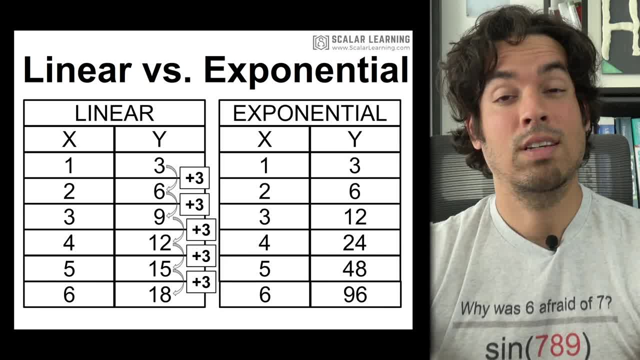 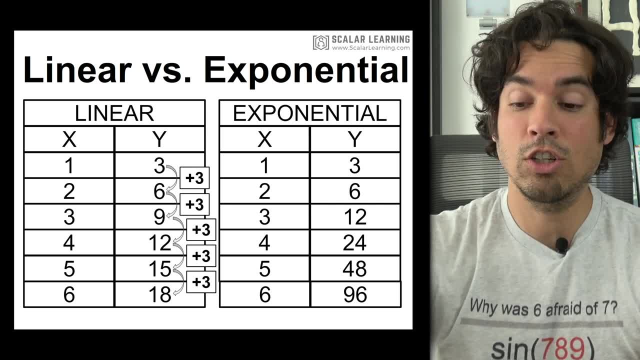 we know we've got a nice linear function, a nice linear equation. In contrast, for exponential we see that as the left goes up by 1, the y is not going up by a consistent amount in terms of addition. Instead, it's going up by a multiplying factor. 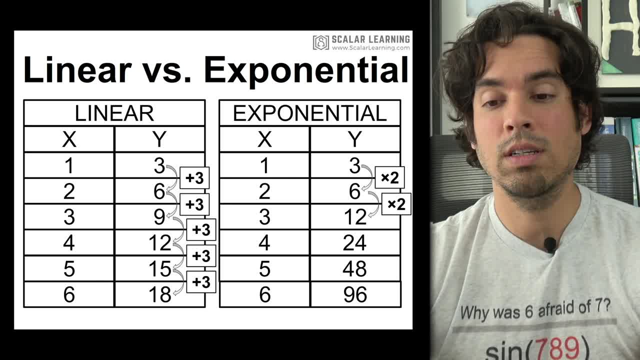 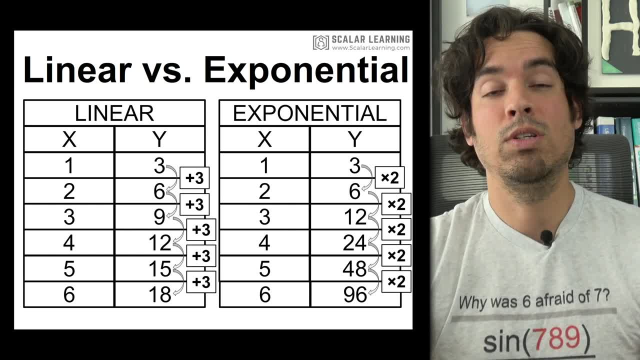 And in this case it's times 2.. So, doubling, doubling, doubling, doubling and doubling. So that is how we could differentiate, if we're looking at data, actual hard data, between linear versus exponential growth. It's also important to be able to identify graphs that are 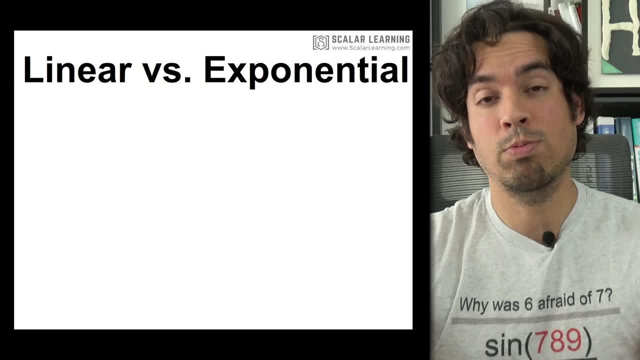 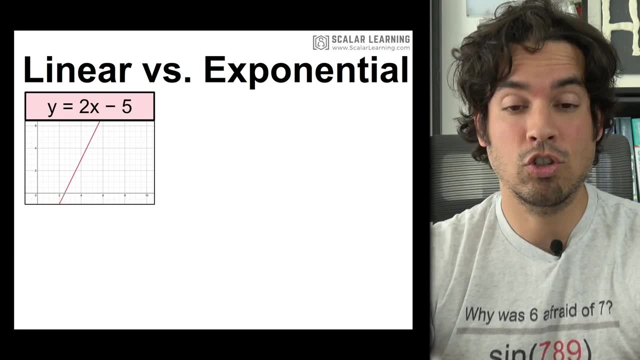 linear versus exponential, which may not be that difficult for some folks. But for folks who are unfamiliar with this distinction, linear is always a line. It's always straight, right straight down the middle. So this is one with a positive slope. y equals 2x minus 5.. 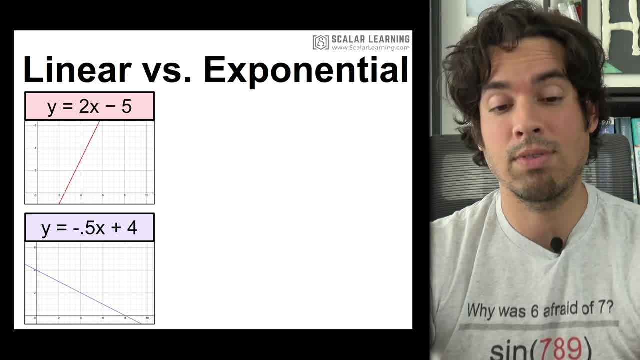 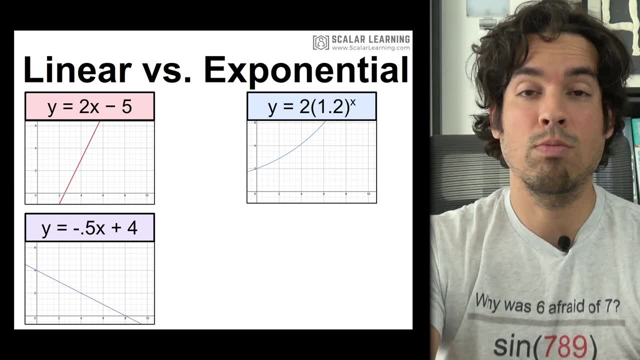 And here we got a negative slope of negative 0.5 or negative 1 half x, with that y intercept of 4.. Likewise, exponential can be positive, or exponential growth as we call it. We're sloping up And in this case that is a 1.2 inside. 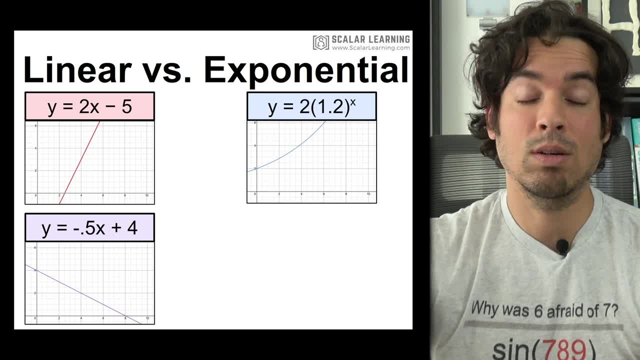 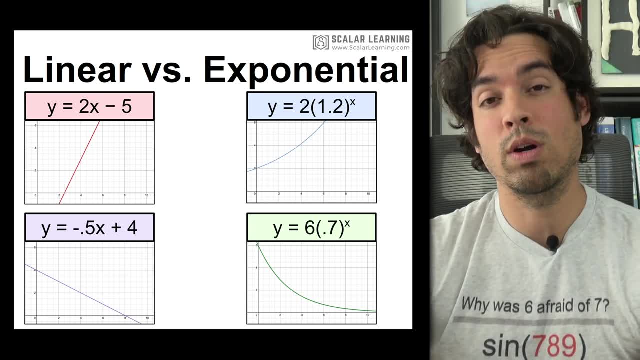 which means that's actually is growing by 20% every year or day, depending on whatever the time unit is. And then here we have exponential decay, And you notice now inside the parentheses it's now a number between 0 and 1,. 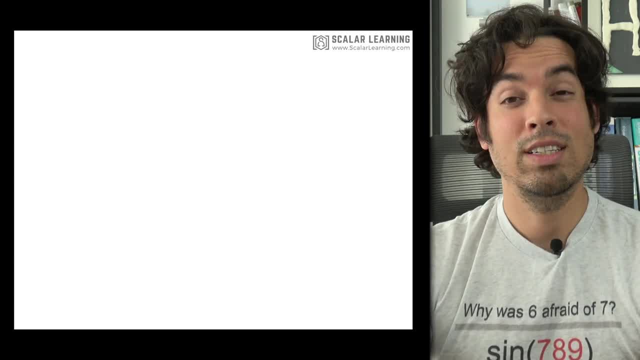 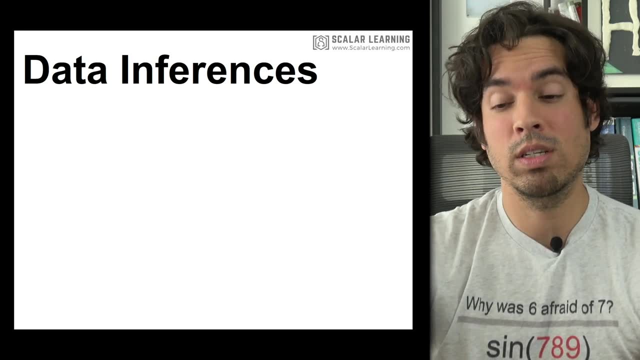 like 0.7,, 0.3,, 0.1, so on and so forth. Now let's go to data inferences. This is a notoriously difficult and confusing subcategory, So I want to go over some of the main points that you need to know and understand. 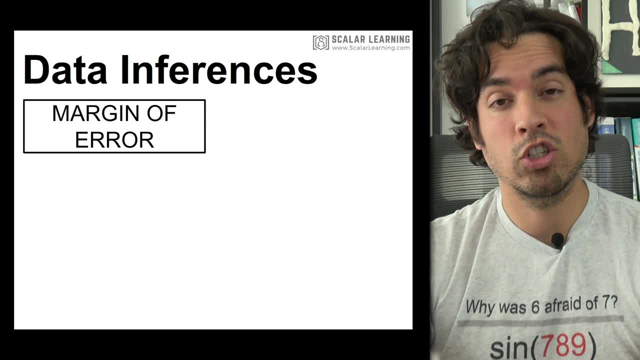 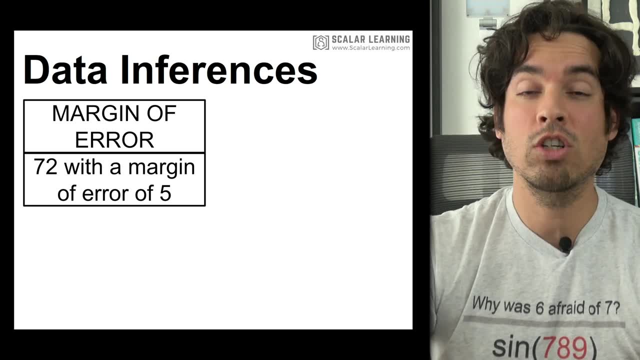 to rock out in this section. So first of all, they talk sometimes about margin of error. What is margin of error? So let's say they say the mean or the main value that we determined is 72, with a margin of error of 5.. 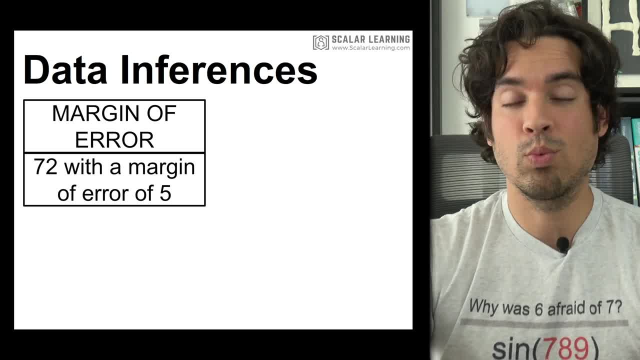 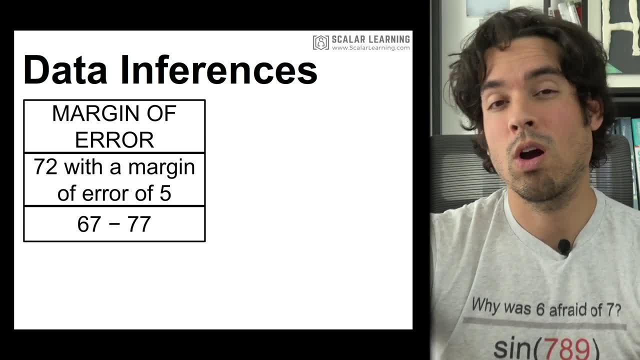 That means that the true value of whatever you're trying to measure is within 5 of 72.. So it could be plus 5 or minus 5, meaning down to 67 or up to 77.. And another thing that is often talked about is confidence level. 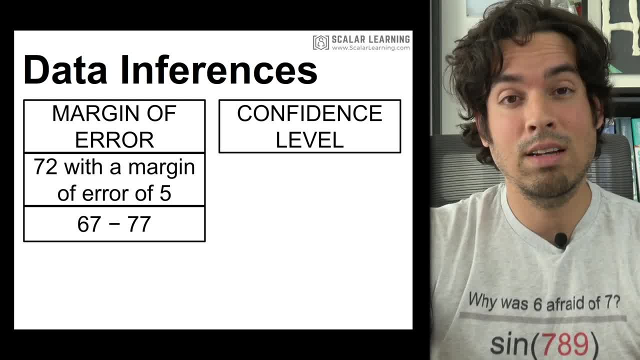 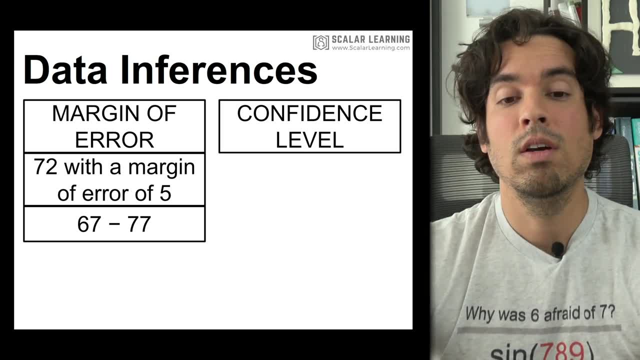 It's like: what is confidence level? Well, it's kind of what it sounds like: If you have a 99% confidence level that you've gotten the right piece of data, that's higher than 95%, higher than 80%- okay. 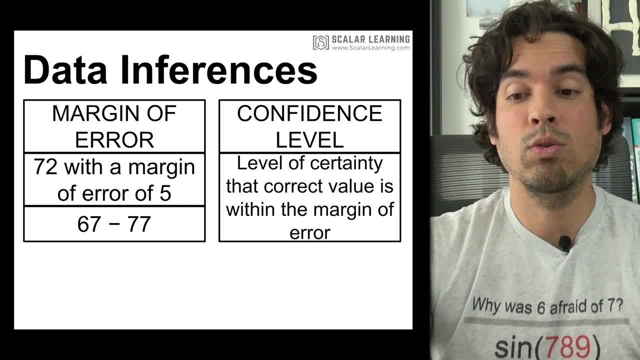 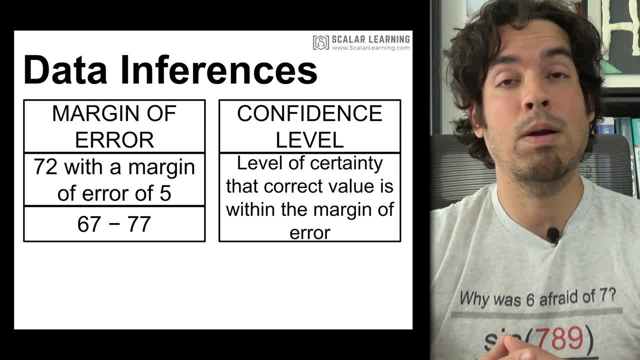 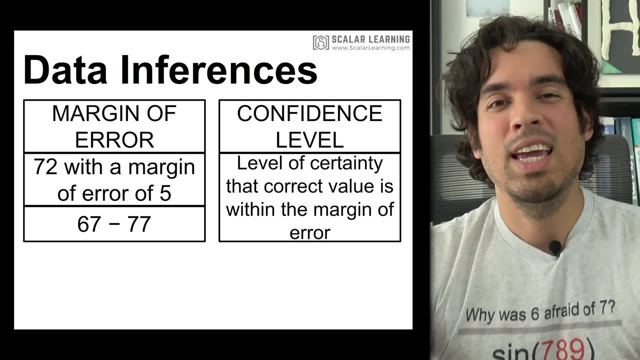 So, for example, we would call it the level of certainty that the correct value is within the margin of error of what we've measured. So it usually makes sense that if, let's say, my margin of error is, let's say, the value is 72, and the values could go up to 100 and down to 50, something like that. 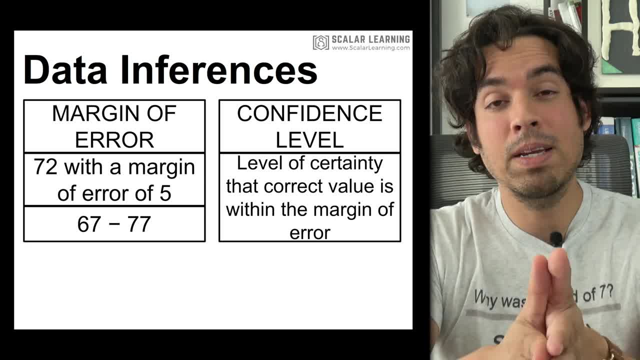 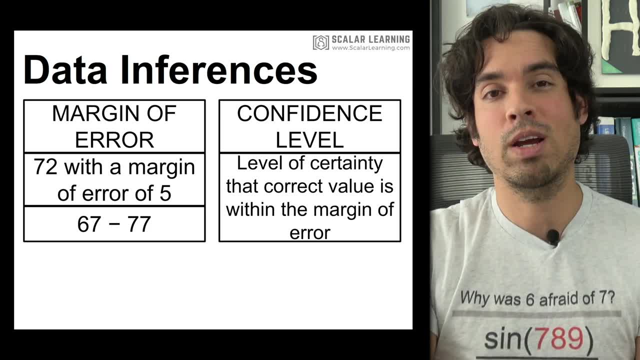 If I want to have a 100% confidence level, I'd make that margin of error as wide as possible to cover everything. Now that doesn't really tell you anything. If you have that big of a margin of error, your study is not very good, doesn't give. 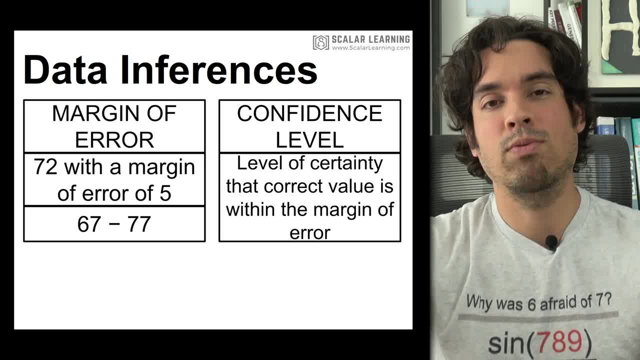 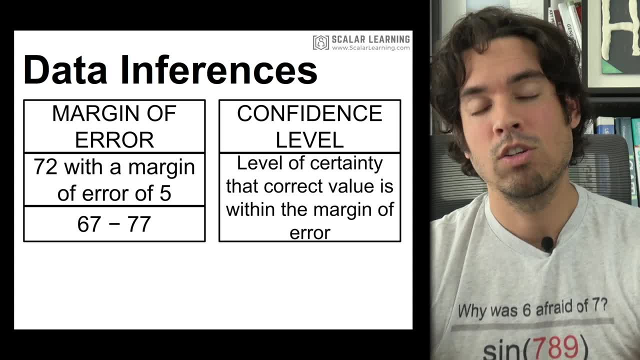 you any insights. But the point is is, if our margin of error is so wide that we know every value, potential value, is in there, our confidence level is 100%. So what that means is, as the margin of error increases, the confidence level increases. 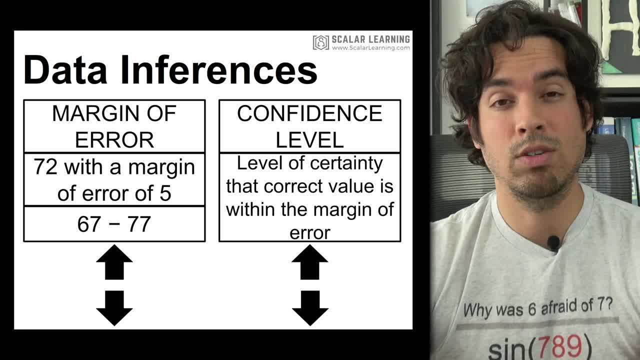 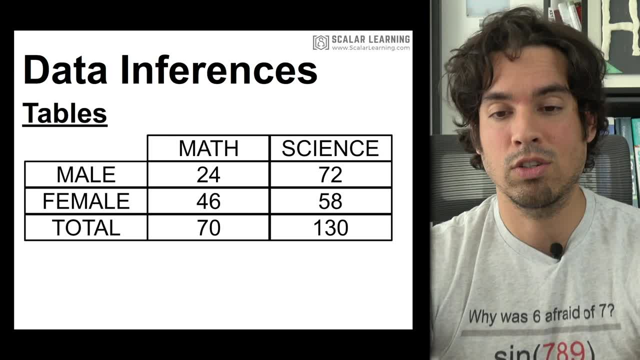 As the margin of error decreases, the confidence level likewise decreases. Another thing that you've got to be comfortable with is how to make data inferences from tables. So we're going to talk about a couple of things. We're going to talk about a couple of examples here. 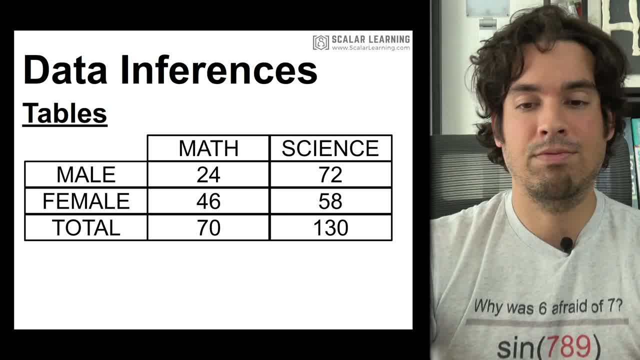 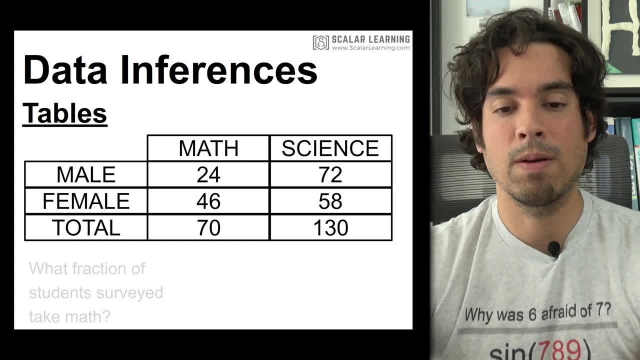 So let's say we've got this nice table of male and females enrolled in math and science at some university or school or whatever, and we've got the totals and everything listed out nicely. All right, So say we get the question: what fraction of students surveyed take math? 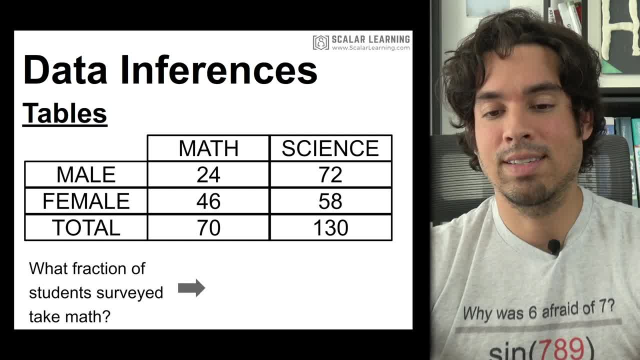 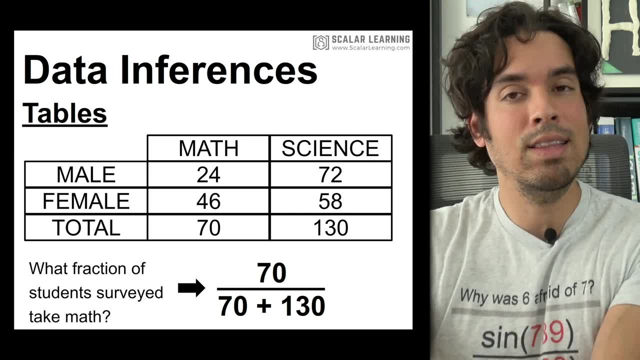 Okay, We know that the total amount of people that take math is 70,. right, We know that the total amount of students- period we're talking about, the total students- is that 70 and that 130.. Okay, So that's how we read this table. 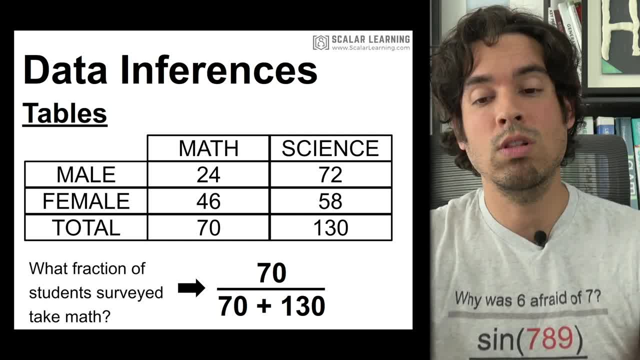 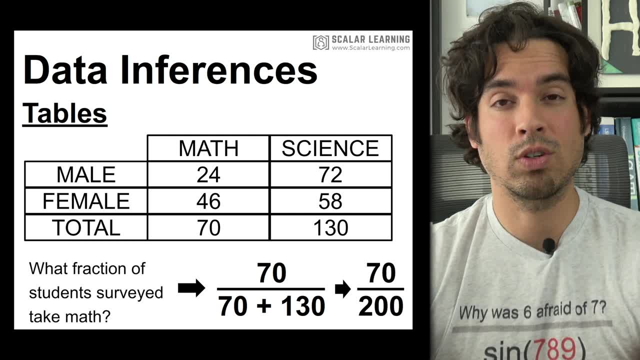 It's not just 70. That's the people that take math. but the total amount of students is the combined value of that 70 and 130, which is, of course, 70 over 200.. Now we're going to get that same data set, but we're going to ask a slightly more complex 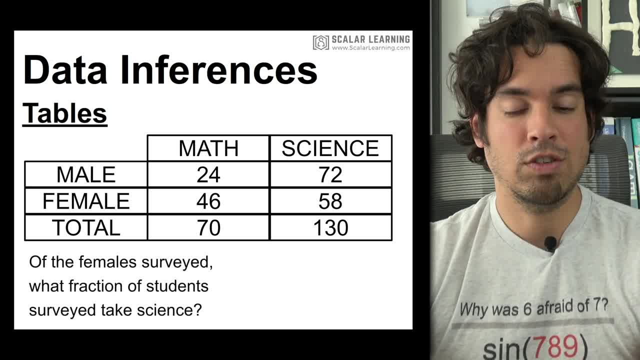 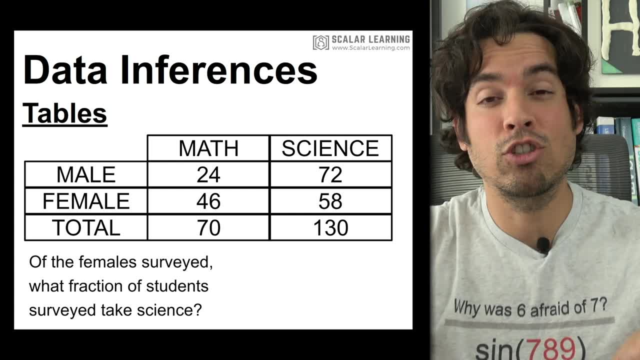 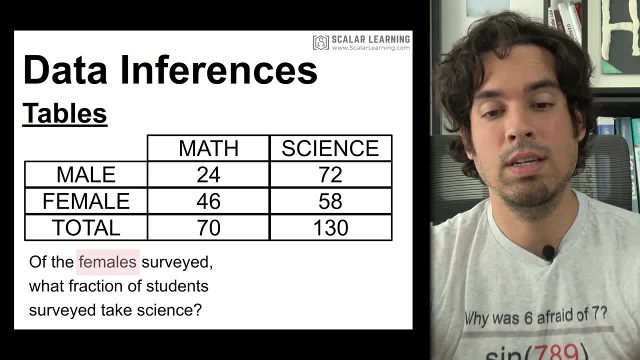 question Of the female surveyed. what fraction of students surveyed? take science. Now. this is a sneaky question, because now they're not just asking about everybody, They say you've got to look at of the female surveyed Immediately. now we're limiting the survey to simply female. 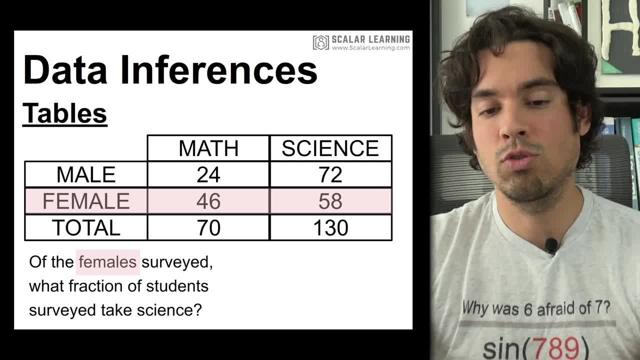 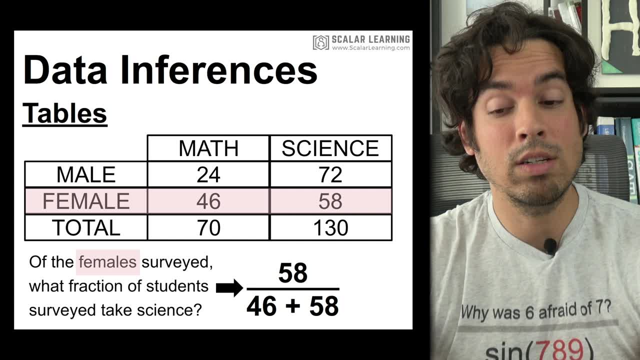 So you notice how that's now highlighted. Of the female surveyed, what fraction of students surveyed take science. Well, what is that? It looks like it's 58. take science out of. now. it's not the grand total of 200, because 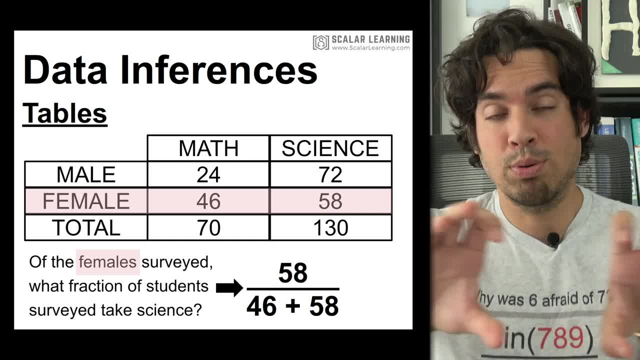 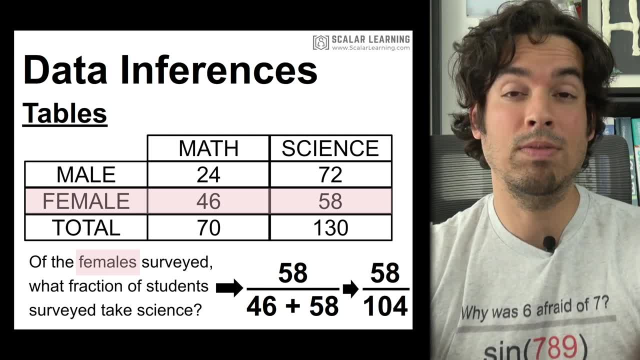 we've limited it, We've cut our group, our initial pool, to just the females. So then that total is 46 and 58.. Add those together and we get a fraction of 58 out of 104.. One more quick example. 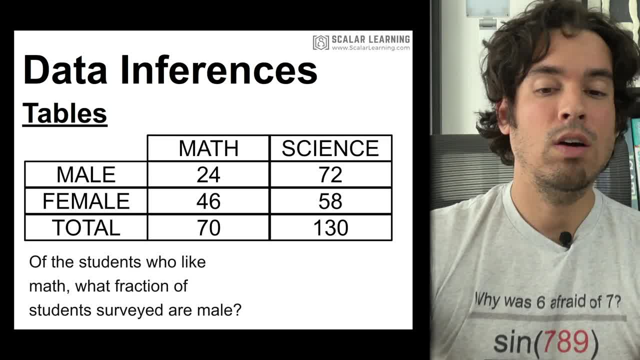 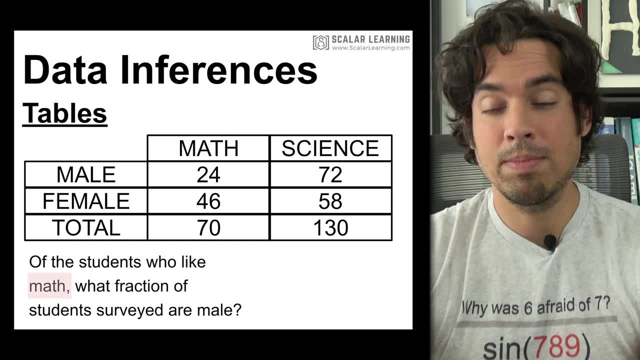 We're going to go back to our previous question, For example, with this same set of data of the students who like math. what fraction of students surveyed are male? Now, again, we're limiting it to students who like math. So that is this subsection, of course, assuming they're not just taking it, but they also. 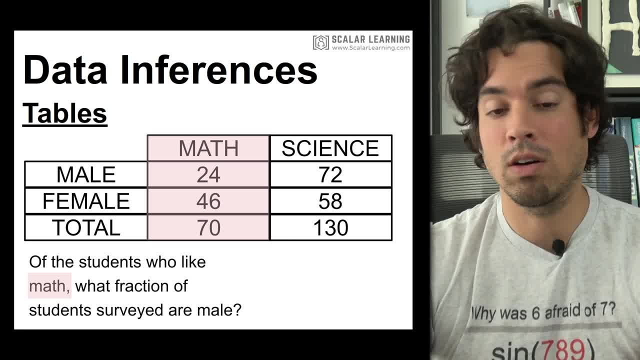 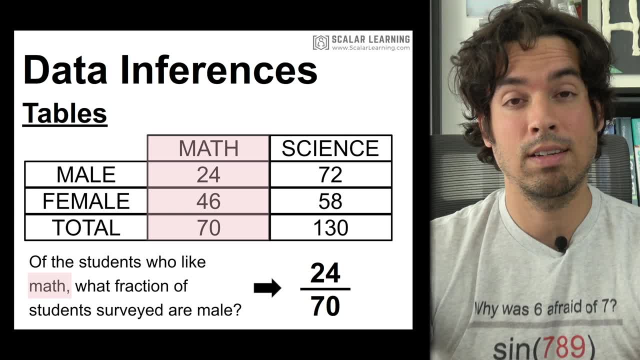 like it. What fraction of students surveyed are male? Well, we again know that it looks like there's 24 male out of a total of 70 that take math. and that's it. Now let's move on to center spread and shape of distributions. 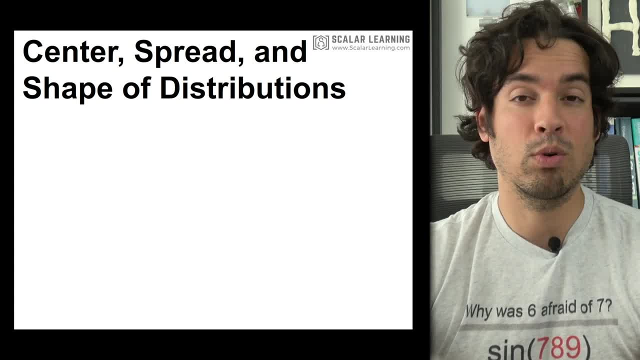 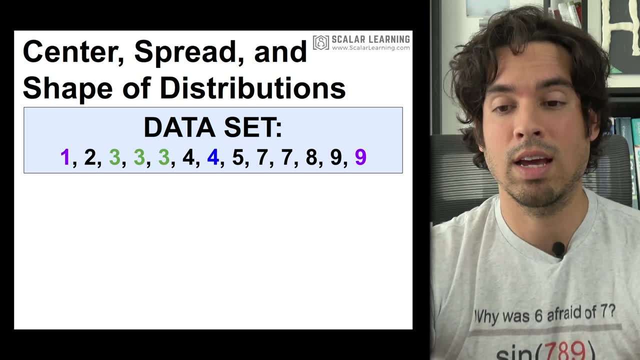 Okay, So we have a lot of information to unpack in this category, very important category. So, first of all, we are always assuming that we're analyzing some sort of set of data, So here's a sample set of data. Okay, And this is the entire thing that Red's going to come in handy where we're going to talk. 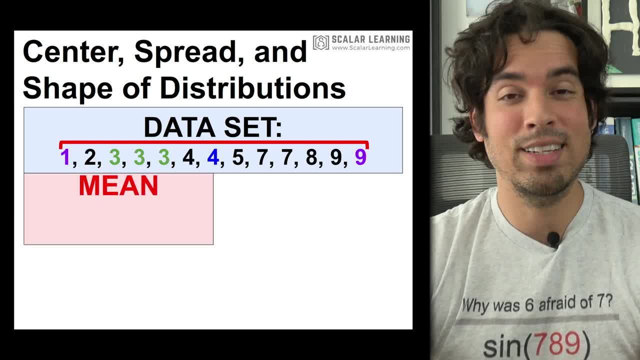 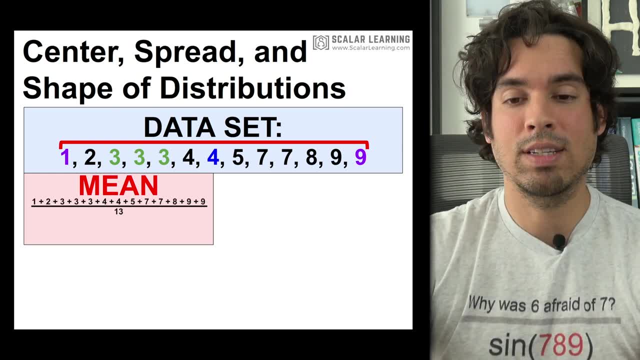 about mean, All right. So first thing you got to know is what is mean? Mean is synonymous with the word average. How do we take an average? We take that entire group of data, all those numbers, we add them together and we divide. 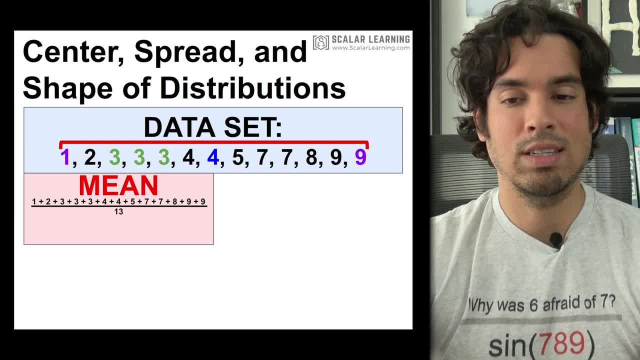 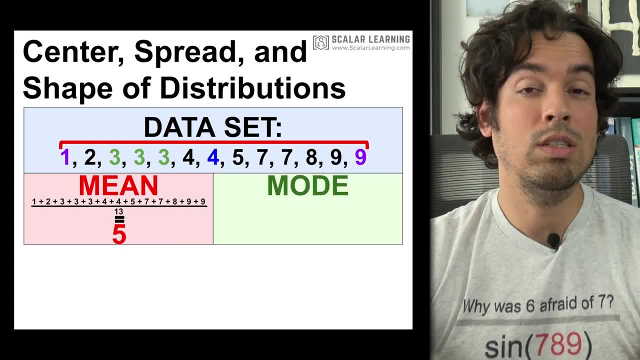 by 13.. Why? Because there are 13 numbers in this data set. if you count them up and there we sum it up, divide and we get a mean of five. All right. Next, you also need to know what is the mode. 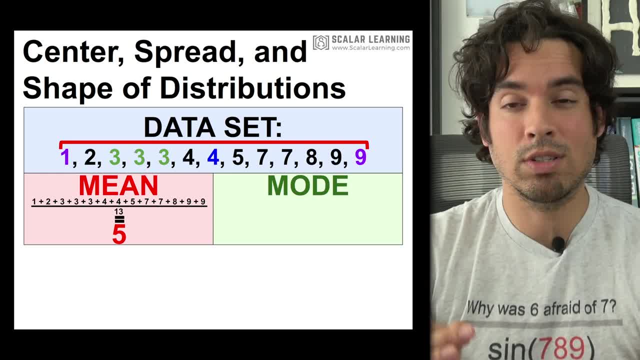 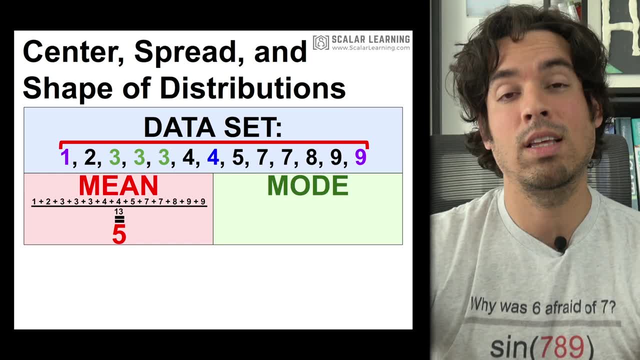 The mode value is the value that you see the most frequently, So mode kind of sounds like most. so you can use that to help yourself remember what mode is. And again, in green I've highlighted the mode which is three. Now, it's not the most, it's not the biggest value, it's not nine, it's the one you see. 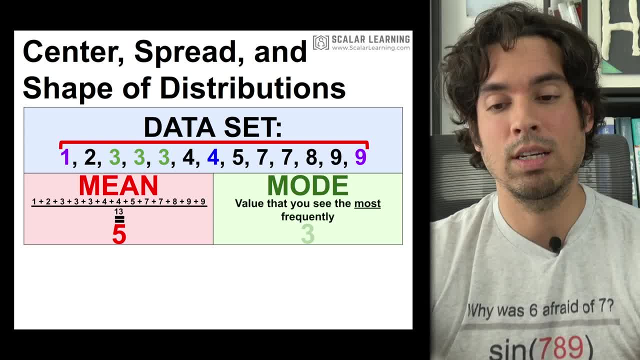 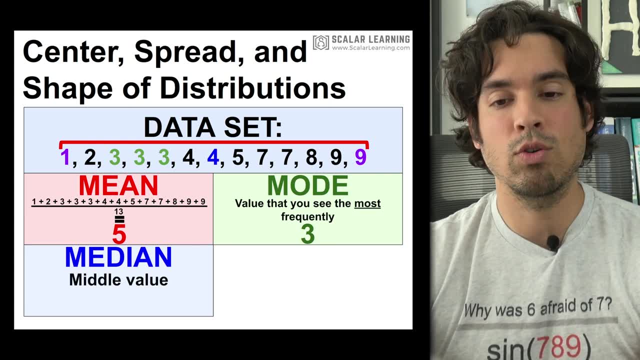 the most. Therefore, the mode, the value you see the most frequently, The most frequently is, of course, three. Next, we have the median median sounds like middle and it is indeed the middle value of the set. Now, to find the median, the first thing you have to do is organize all the data from least. 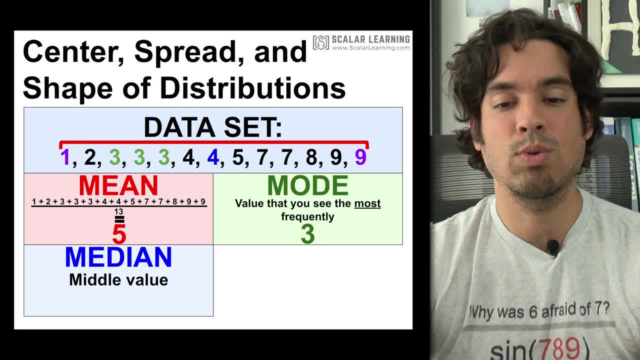 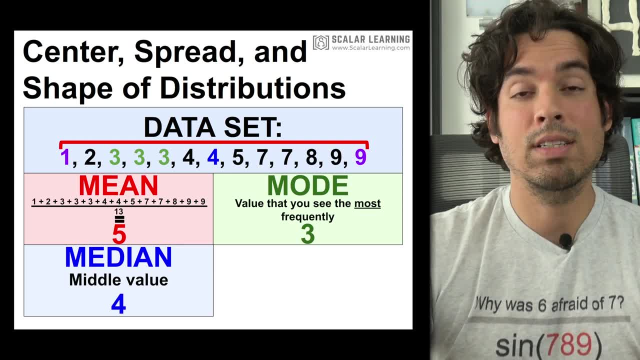 to greatest. And then you look at that precise middle value And in this case, because we have an odd number of values, it is the 13th value, which is four. In the case you have an even set of data. let's say we had 12 pieces of data. 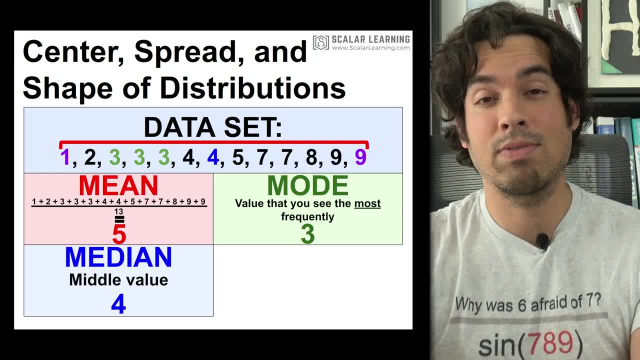 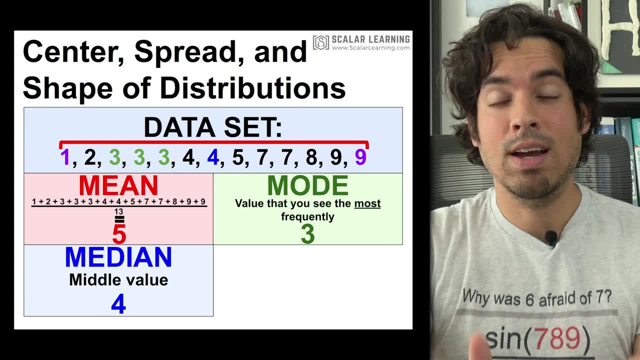 You'd have two values, kind of in the middle right You'd have the sixth value and the seventh value. In that particular case you take the average of those two, meaning if I had my two values being four and five, I'd add four and five together, divide by two and I get 4.5. 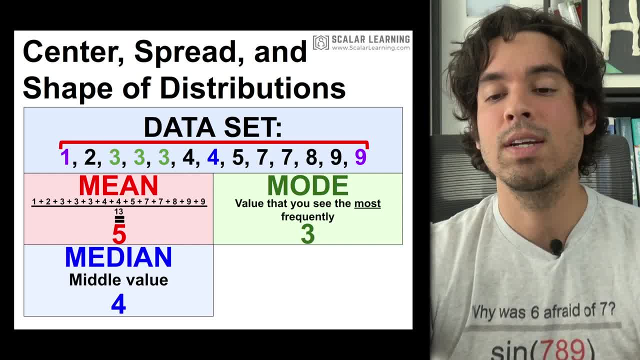 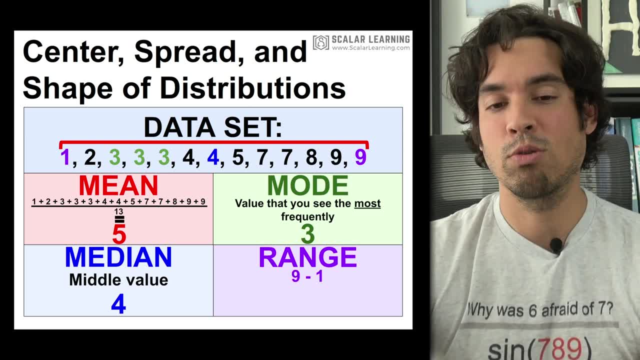 The other way to think about it is: what's right between four and five is 4.5.. Last but not least, we have the range. Range is simply the greatest value minus the least value. Those are denoted in purple right. 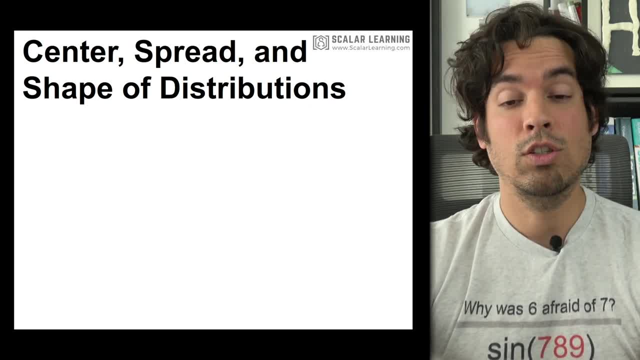 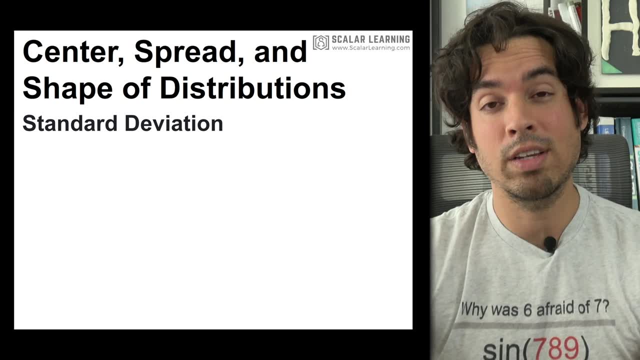 So nine minus one gives us a range of eight. Next, we're going to talk about standard deviation. Believe it or not, I've tested on the test, but the great news is you don't have to ever calculate it. You just have to understand what it means. 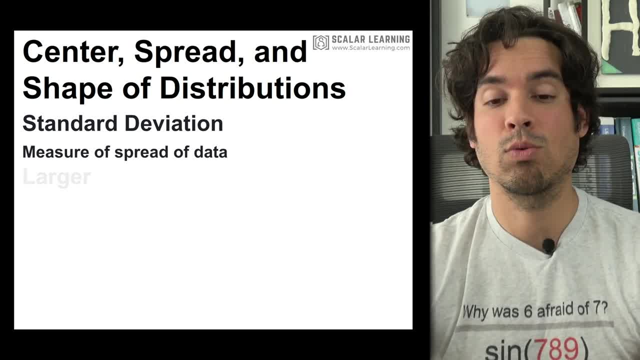 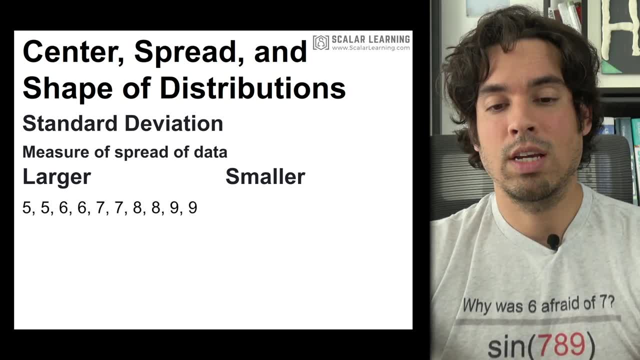 So standard deviation is the measure of the spread of the data. So what do I mean? We're going to take two examples where we have a larger standard deviation and a smaller standard deviation. So here's a large standard deviation and you can see from the data it's really spread. 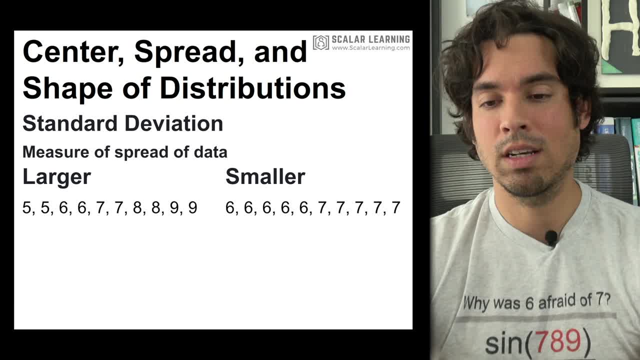 out right: Two fives, two sixes, two sevens, two eights, two nines And now, in a smaller standard deviation, sixes and sevens all the day. it's the same amount of data, but it's all bunched closer together, right. 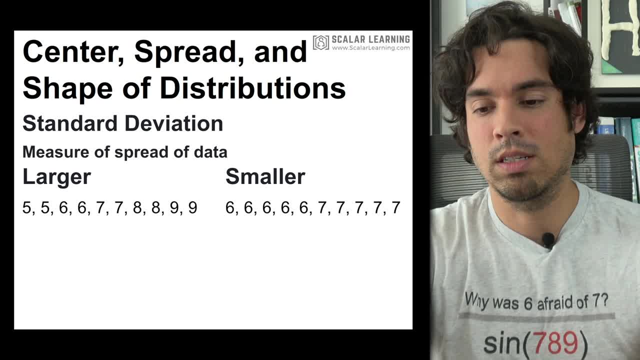 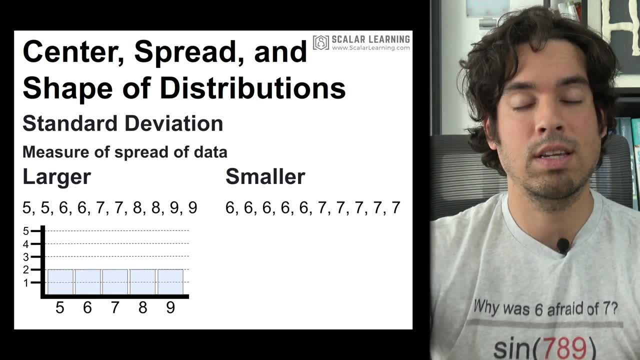 They're really close. It's really sixes or sevens, you know. maybe the mean is 6.5.. And now, what does the graph look like of the larger standard deviation? Look at that, nice, even spread across the five, six, seven, eight, nine. 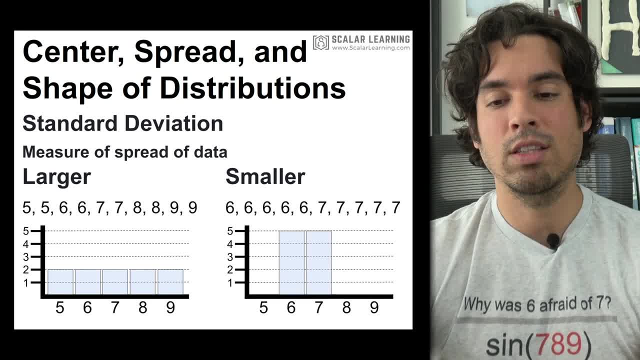 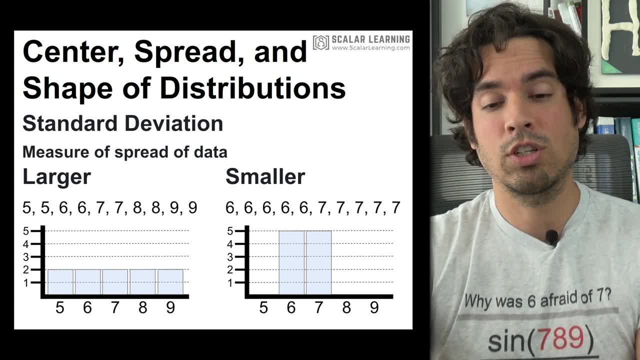 It's very equally distributed versus here It's all bunched together at six and seven. So again, standard deviation is that spread. when it's a smaller spread, it's a smaller standard deviation, and vice versa, When it's more spread out, it's a larger standard deviation. 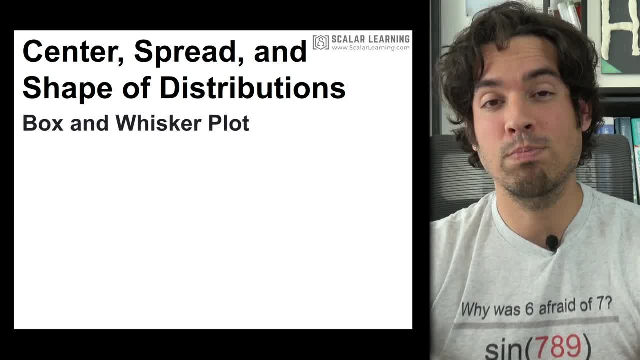 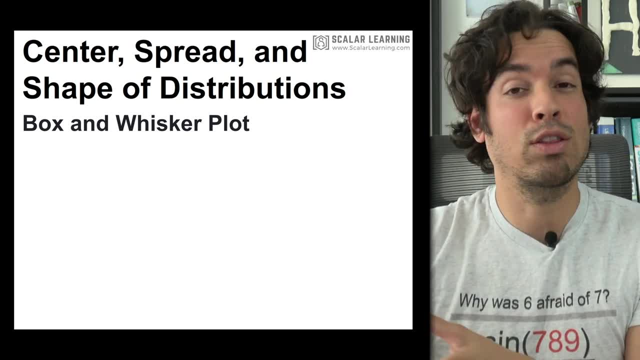 Something else you should get familiar with is box and whisker plots, And the reason why is: look, I've seen them on real test before. They don't show up very often, but I saw like a three part question on box and whisker plot. 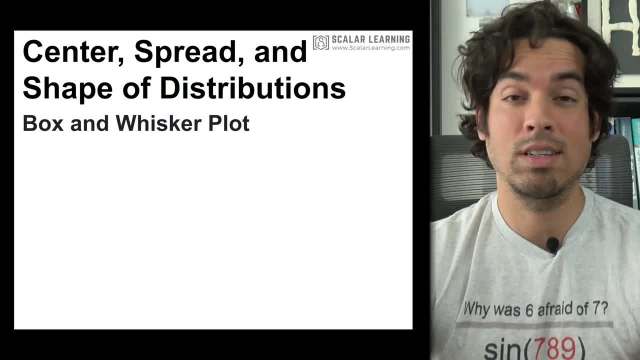 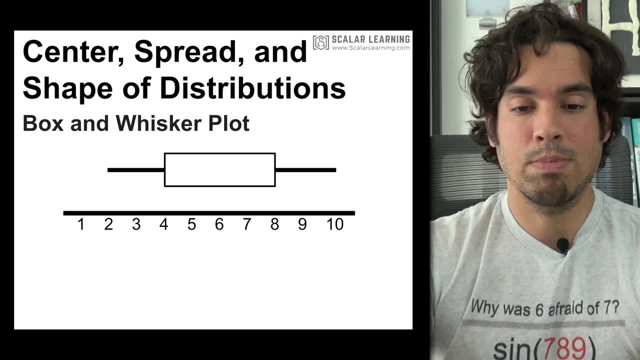 once. So I do think it's worthwhile to know how to use these, and it's not that complicated, So I'm going to explain all the ins and outs right now. This is what a box and whisker plot looks like. The data is at the bottom: one, two, three, four, five, six, seven, eight, nine, 10.. 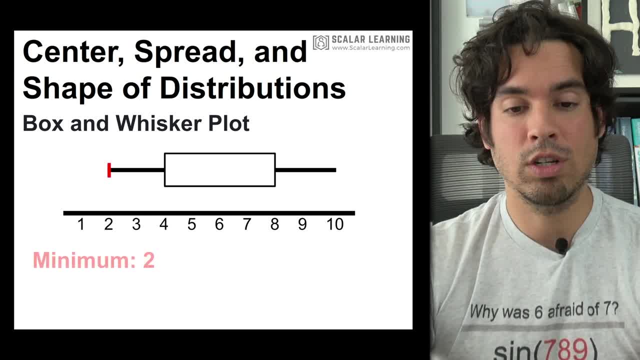 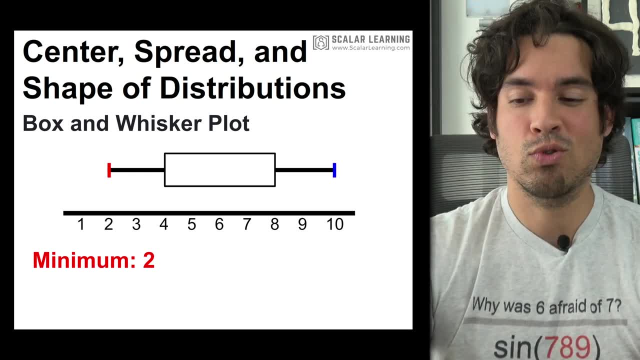 And there's some key parts. So first we've got the left edge in red, which denotes the minimum, And in this case the minimum value would be two. Then, of course, we've got that, That right edge, And that's like: these are the whiskers, of course, and that is the maximum value. 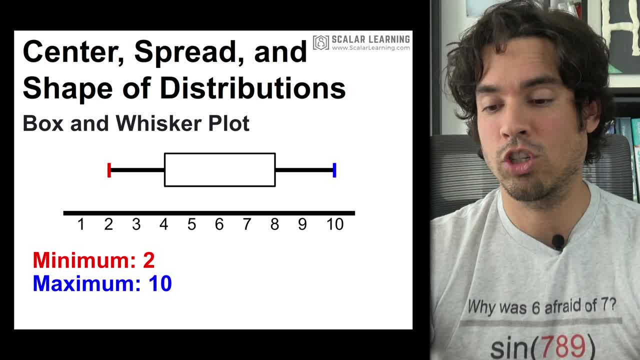 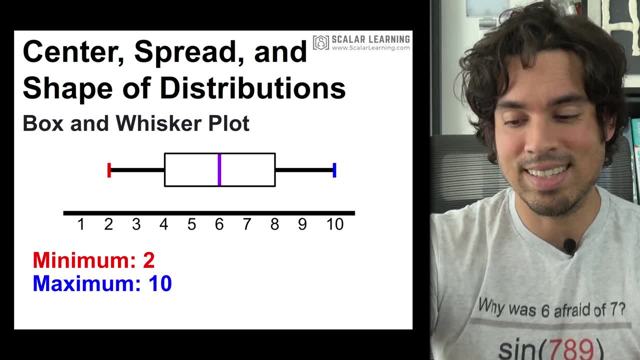 So if you know those two points, you can calculate the range, which in this case is eight. Then we've got the middle value down the line in down the middle, right there at six, And again it doesn't have to be in the middle of the box. 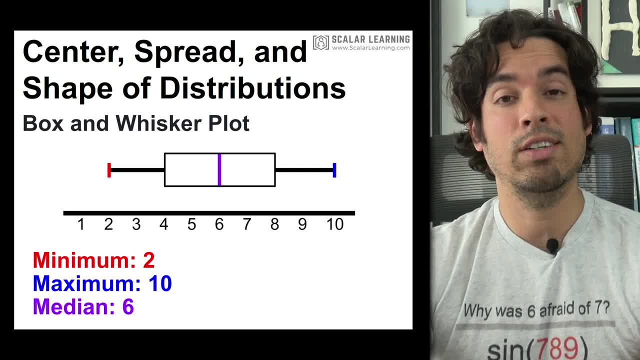 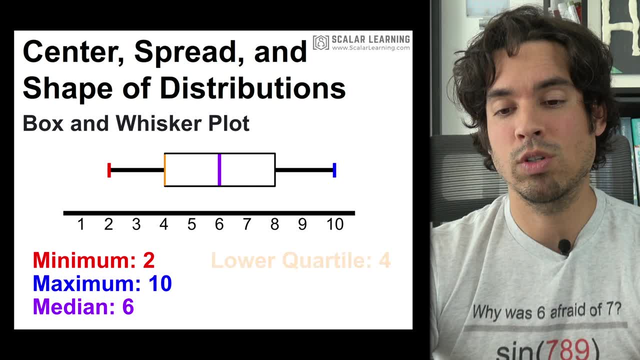 It just happens to be here. That gives us the median. So if they ever ask you what's the median in a box and whisker plot is where that line is, Then we have this orange edge to the left of the box. That is what's called the lower quartile in there. 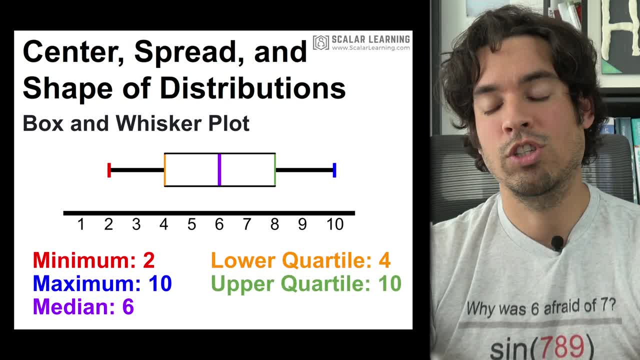 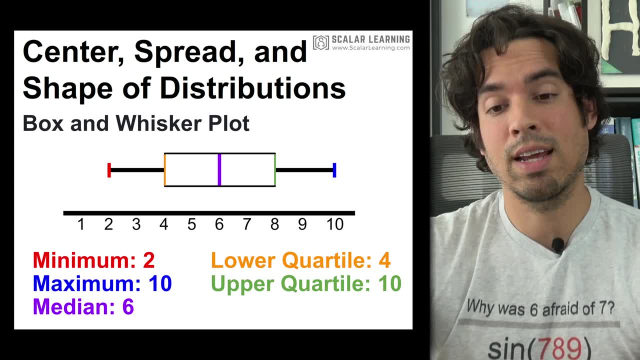 That's at four. And last but not least, we have this green line here, which is the upper quartile. Now you likely won't need to calculate the lower quartile and upper quartile from a set of data, But if you do, the lower quartile is the median of the bottom half of the data. 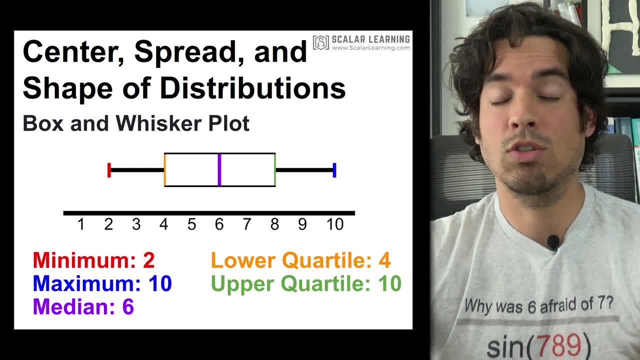 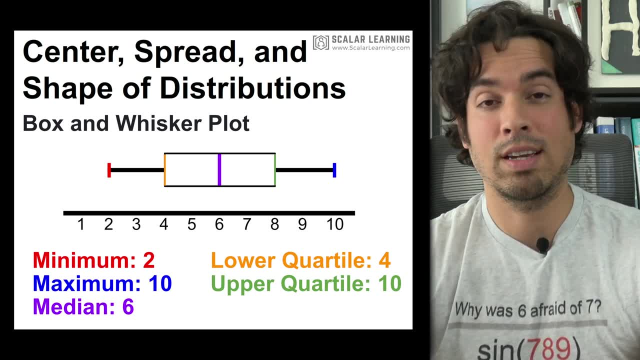 The upper quartile is the median of the upper half of the data. So I'm just telling you that. so you aren't. so you know what those terms are, but I can almost guarantee you that's probably not going to be something you'll need to calculate. 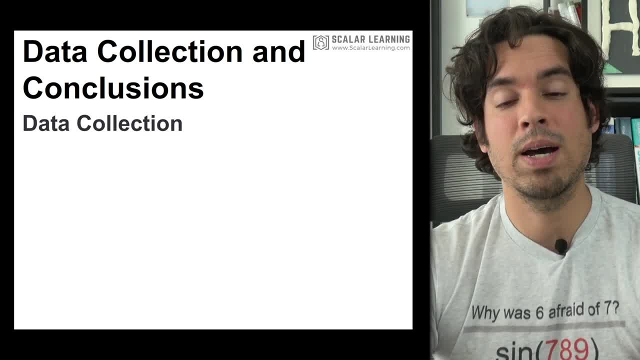 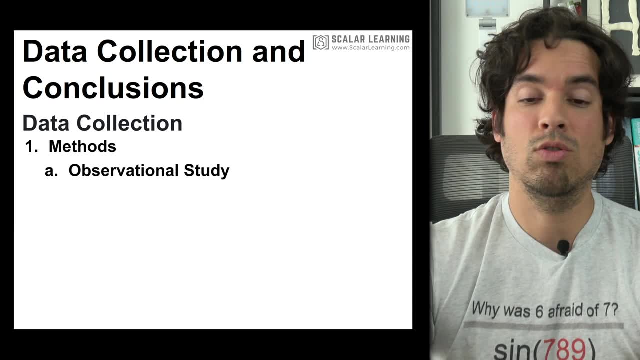 Finally, We're going to end on data collection and conclusions, talking about data collection, And again, this can be a really tough category for a lot of people, So let's talk about the main methods that we can use. We can use an observational study, and that is where you observe subjects and record data. 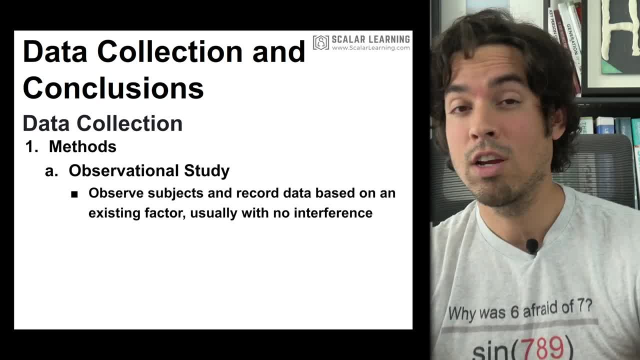 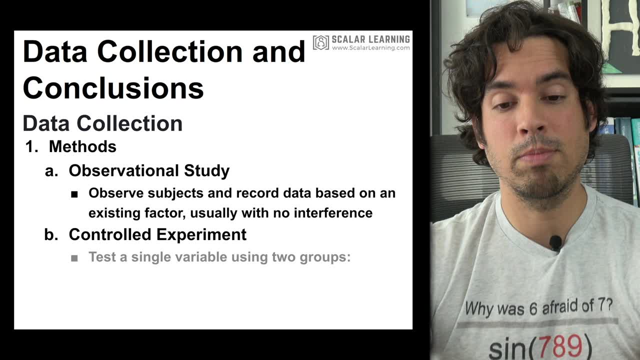 based on an existing factor, usually with no interference. So sort of like you're going out and observing animals in the wild. This is where an observational study would make a lot of sense. You might also have a controlled experiment where you test a single variable using two. 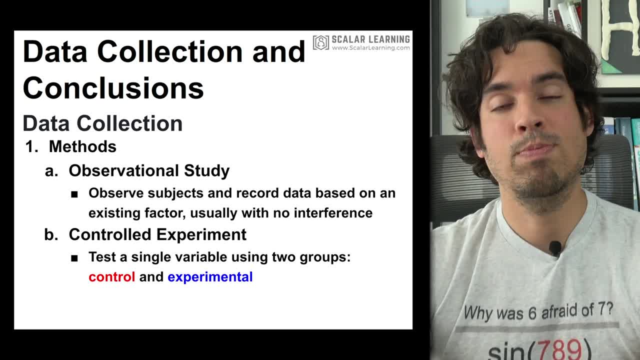 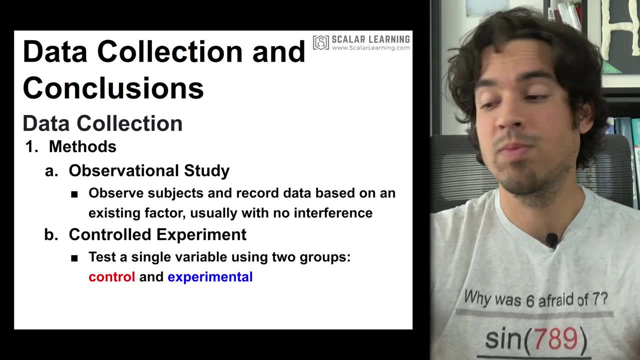 groups: a control and an experimental group. This might be something you would use if you're testing a pharmaceutical right. You want to see if it works. So you say, Hey, you guys are the control group, You take no medication. 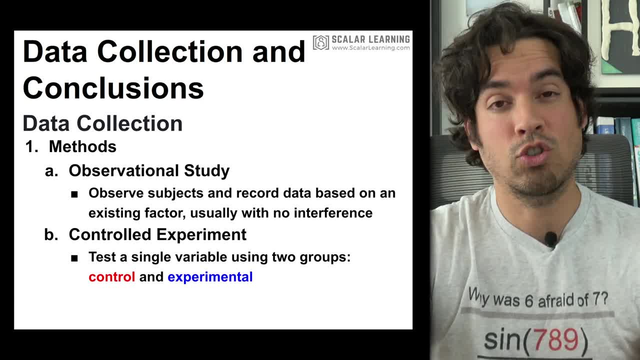 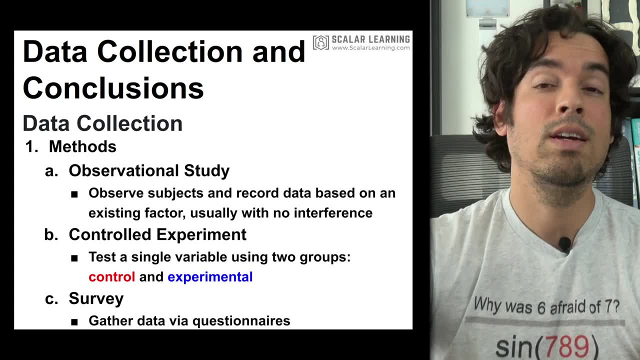 You guys are the experimental. You'll take this new drug and we're going to compare and contrast after two, three months, something like that. Finally, you could give people a survey where you gathered data via questionnaires. You say: Hey, let's scale it one to 10.. 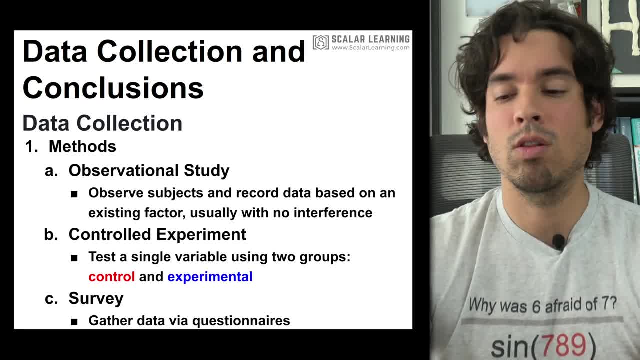 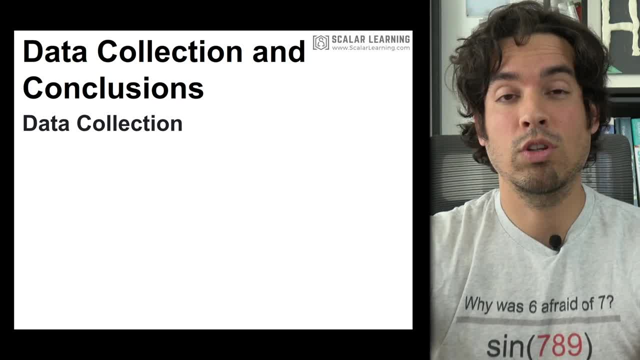 What's your thoughts on building this new highway through our town? Something, something along those lines. Now, understanding those is great, but you don't need to necessarily know those in particular, but what you want to be careful of, Because when we're thinking about how to collect and sample data, we want to look out. 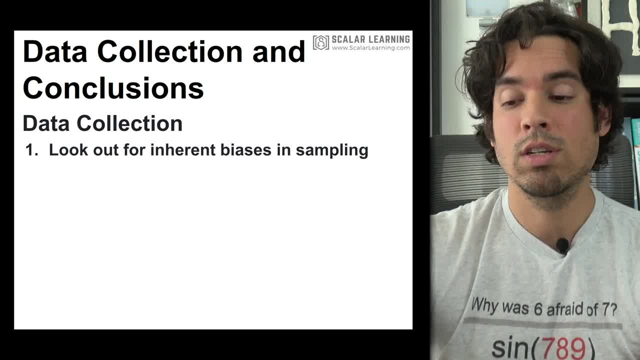 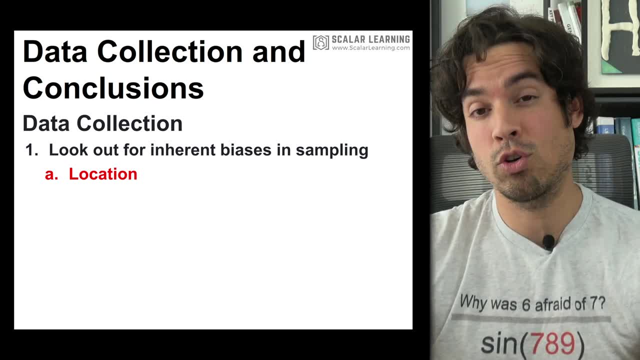 for, uh, inherent biases. That's the key. That's what they're always trying to test you on. On this test, the biases can come in these four broad categories and they're not going to make total sense yet until I show you examples, but it could be in the location of where these 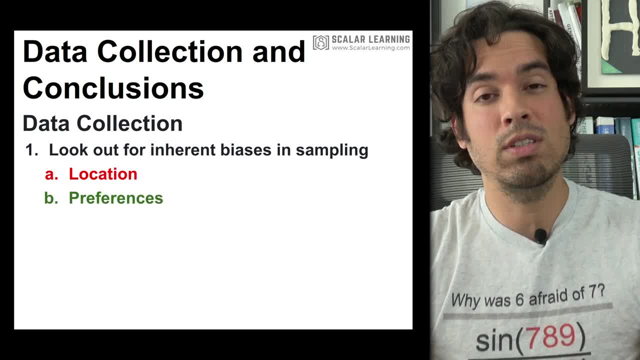 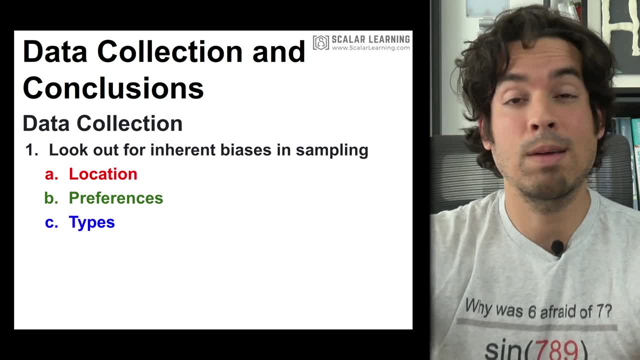 surveys or experiments are happening. It could be based on the preferences of the people that they are selecting or sampling for for these studies. It can be the types, meaning the types of people, Or even the types of people, The types of products that they're looking at. 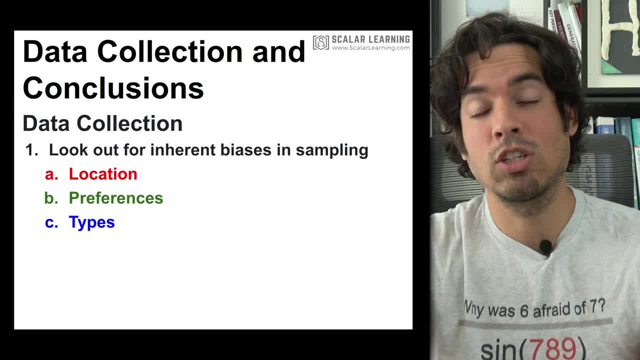 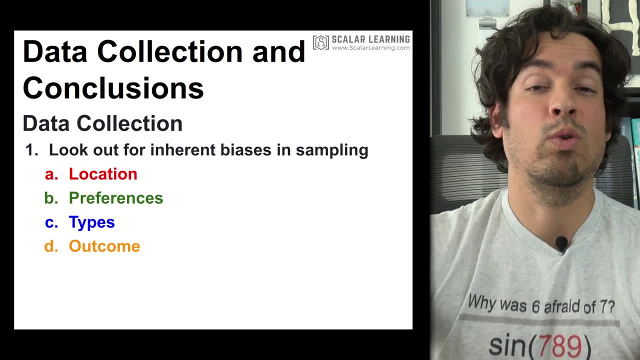 If they're making these random- uh pre- selections of groups of people or items, that can include a bias. And then, of course, if you're, if you're selecting people or things based on a certain outcome, that will, of course, introduce biases as well. but let's talk about particular examples. 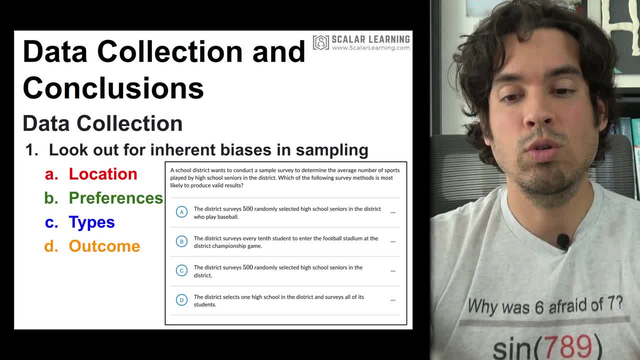 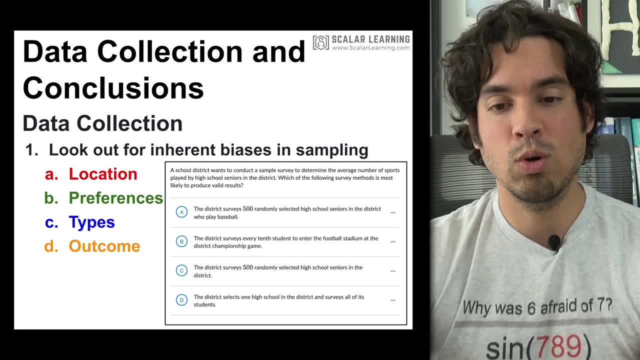 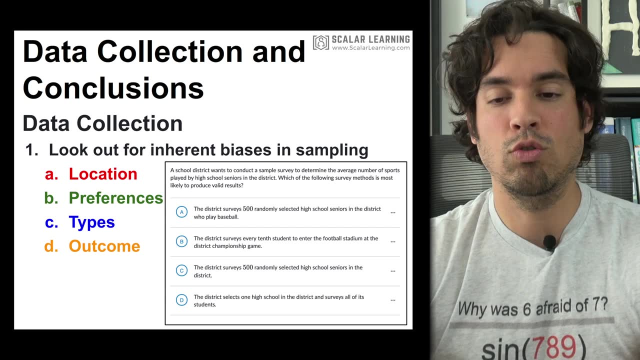 So we've got an example from an actual SAT problem that says a school district wants to conduct a sample survey to determine the average number of sports played by high school seniors. Which of the following survey methods is most likely to produce validation? So it says the district surveys 500 randomly selected high school seniors in the district. 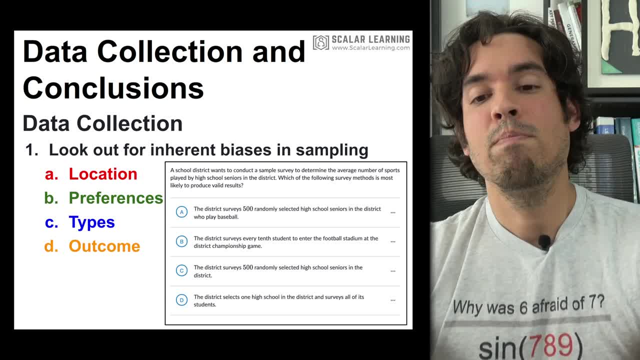 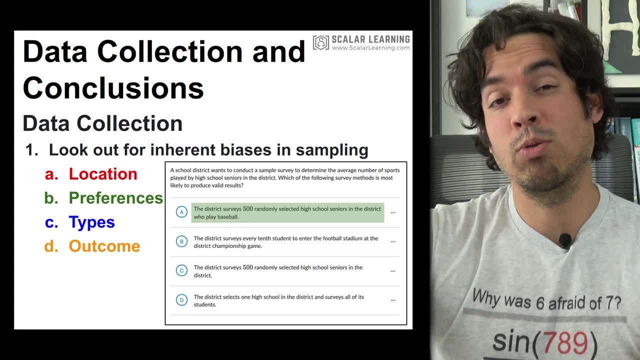 who played baseball. So I like the word random in there. but if we're trying to talk about people who play sports, the problem with this is you are inherently biasing towards people who have a preference for athletics because they already are. You're selecting people who played baseball. 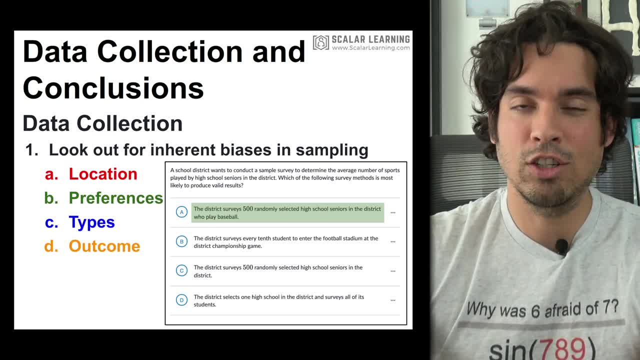 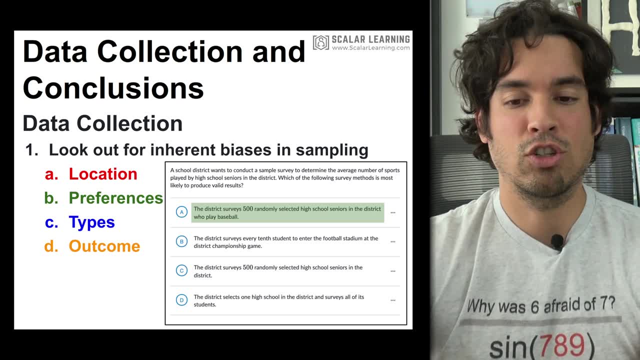 So that's an example of an incorrect bias that's being injected by by way of sampling. What about option B? The district surveys Every 10 students. They enter the football stadium at the district championship game. So to me this is a problem with the location of where you're doing it, right? 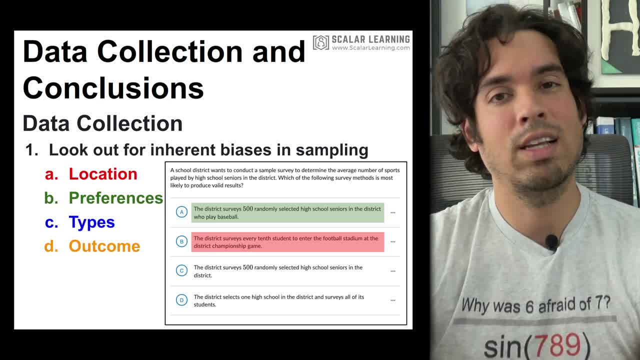 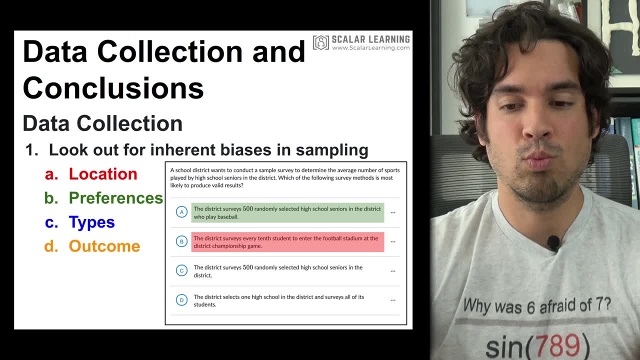 If you're doing it by the football stadium, I believe there's a greater likelihood that these people like sports. They're more likely to play sports if they're going into the football stadium. If we look at option D, the district selects one high school in the district and surveys. 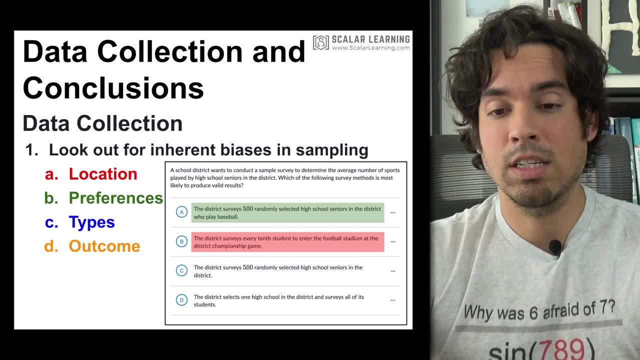 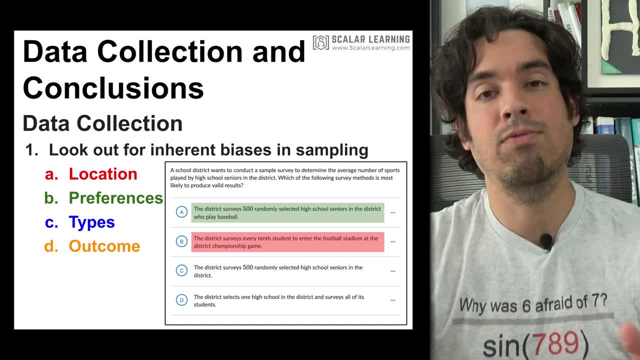 all of its students. Now, this doesn't sound like it's got a bias, but if we want to get a nice even sampling of the district, why focus on one school? We should take a sampling from the district. So this is again another location bias which is not totally clear how it's going to buy. 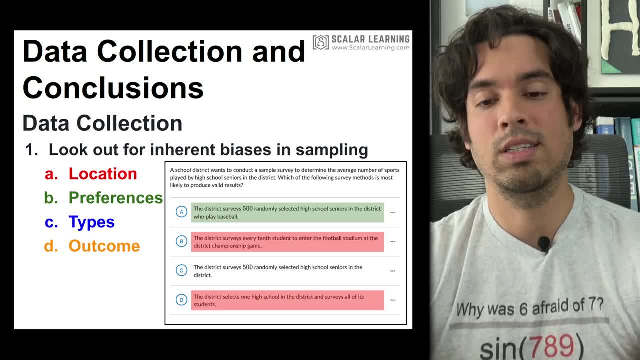 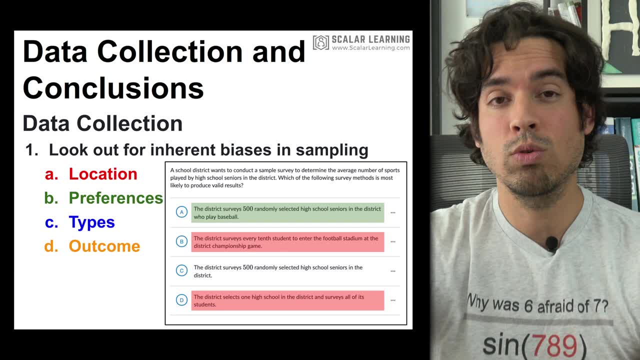 us the results. It's just not the best answer. And that leads us to C, which has said: the district surveys 500 randomly selected high school seniors in the district is perfect, It's across the whole district. That's the ideal sample space and we're good to go. 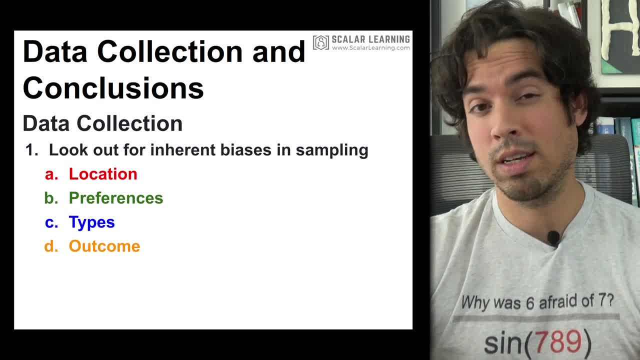 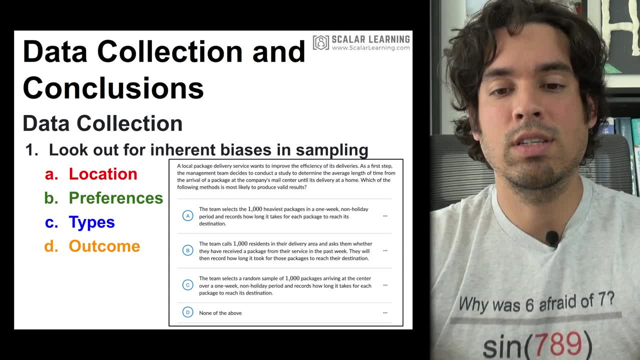 So again, we've got these possible biases and we're going to go through one more example just to continue to clarify. a local package delivery service wants to improve the efficiency of its deliveries. as a first step, The management, The team, decides to conduct a study to determine the average length of time from the arrival. 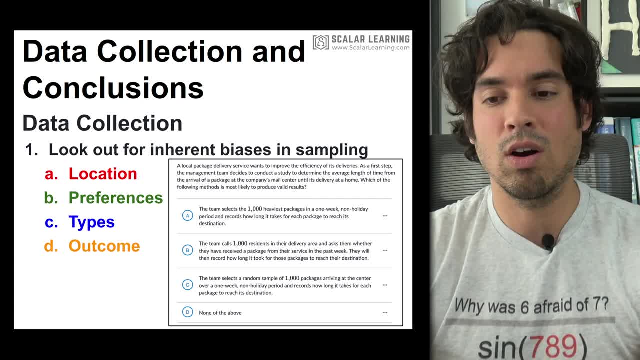 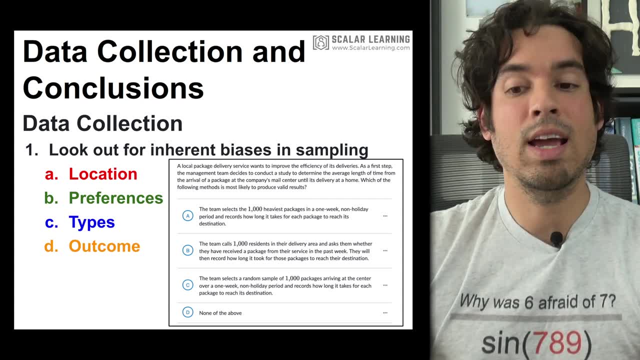 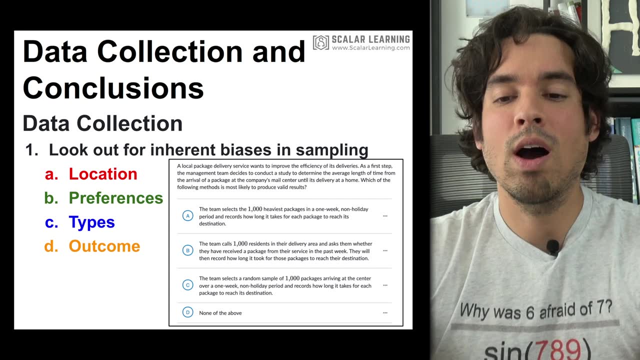 of a package at the company's mail center until its delivery at home. which of the following methods is most likely to produce a valid results? So first, it says, the team selects the thousand heaviest packages in a one week non-holiday period and records how long it takes for each package to reach its destination. 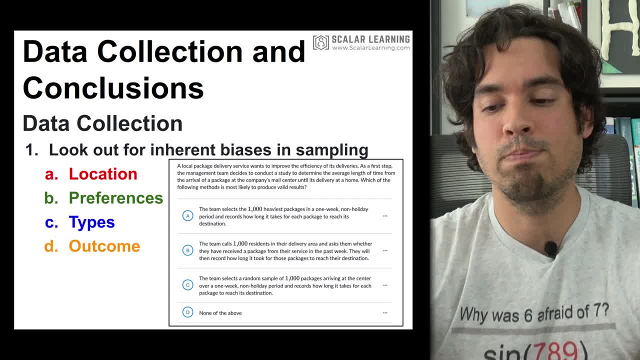 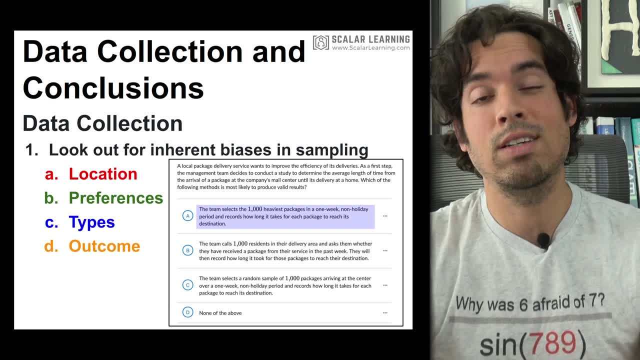 Why select the thousand heaviest? That doesn't make sense. Now we're biasing by types of packages, because maybe heavier packages take longer, Maybe maybe they don't, Maybe they're delivered faster, But whatever is the case, you're introducing some bias that's going to skew the results. 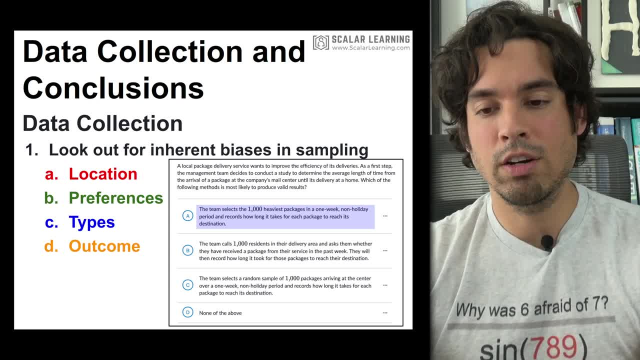 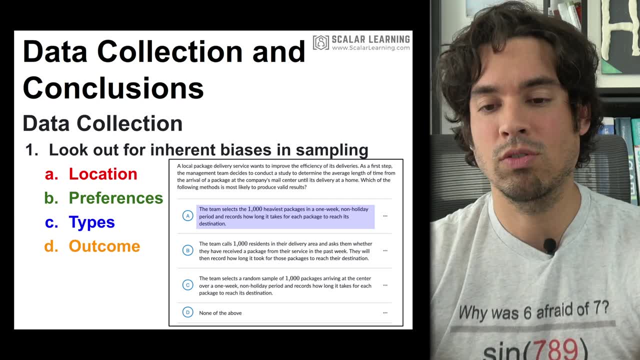 Next, with option B, it says the team calls a thousand residents in their delivery area and ask them whether they have received a package from their service in the past week. They will then record how long it took for those packages to reach their destination. So the problem with this is now: you're biasing by outcome. 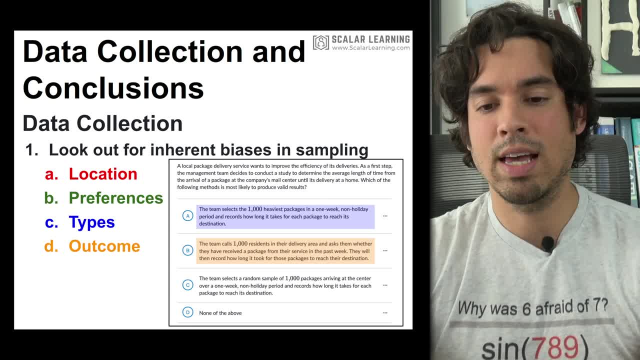 So you're calling people first and saying, Hey, did you receive it in the in the last week? And then, if you did, you're going to record how long it took. Well, wait a minute. What if they haven't received it yet? 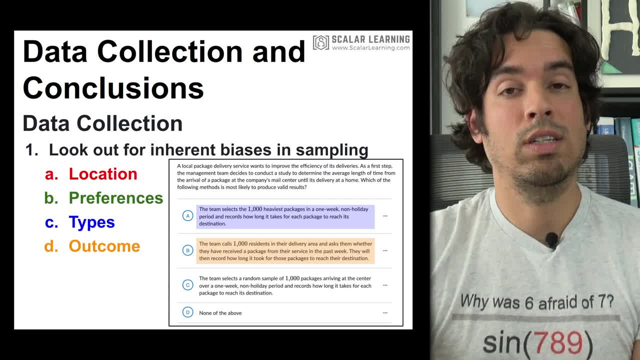 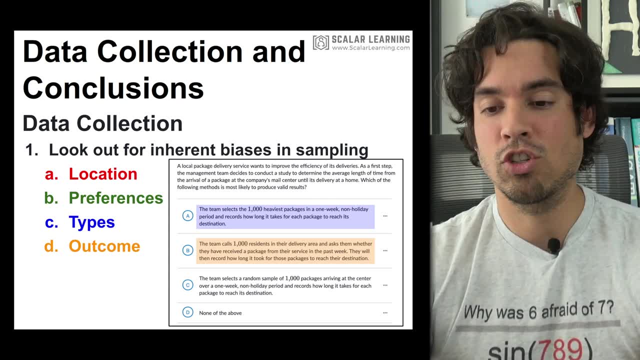 Now they're out of the study. So that's an outcome that you're using to make your sampling and that's going to bias the results. That last one: the team selects a random sample of a thousand packages arriving at the center over a one week non-holiday period. records how long it takes for each package to reach. 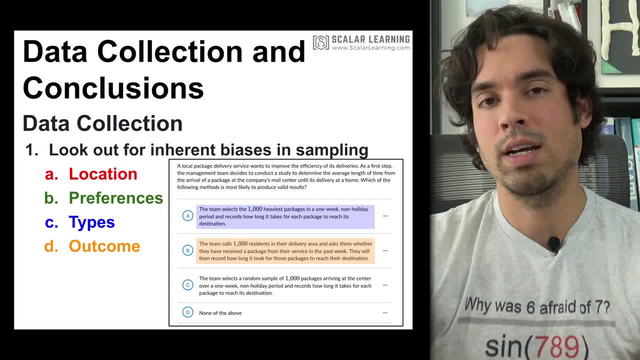 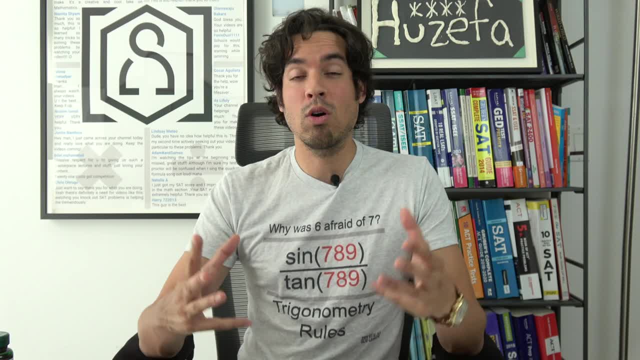 its destination: Perfect, pure, simple, no biases, and we're good to go. I hope you found this presentation useful and to everybody taking their SAT soon, I wish you all the very best of luck And if you did like this video, please click that like button. And I'll see you in the next video. Bye, Take it easy, Take it easy. 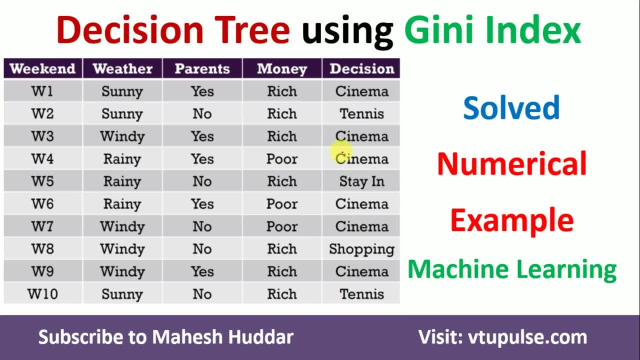 Hi, welcome back. In this video I will discuss how to construct decision tree using Gini index. In the previous videos I have already discussed how to construct decision tree using information key. The link for those videos is given in the description below.